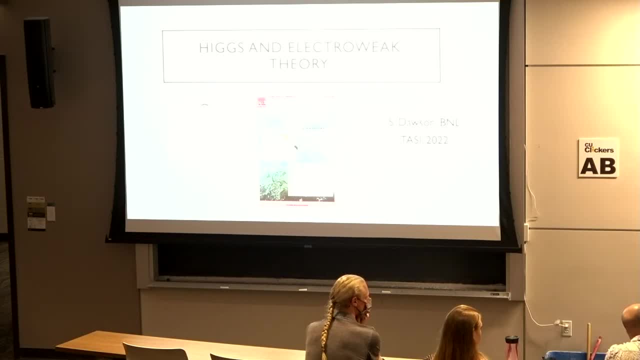 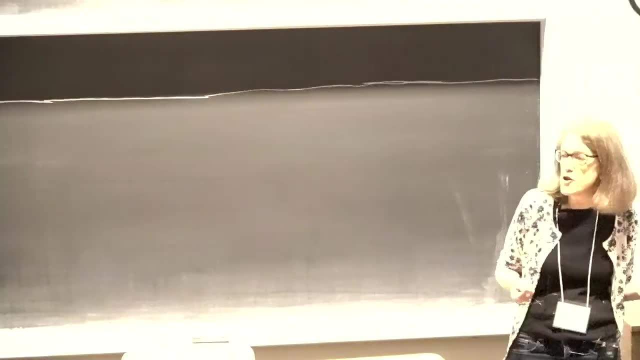 It's one of my favorite things: to come and talk to students and talk about the Higgs boson and just talk about why I study physics. I've done many, many lectures on the Higgs and it's always new. There's always something I learn, so I hope you'll ask me lots of questions. 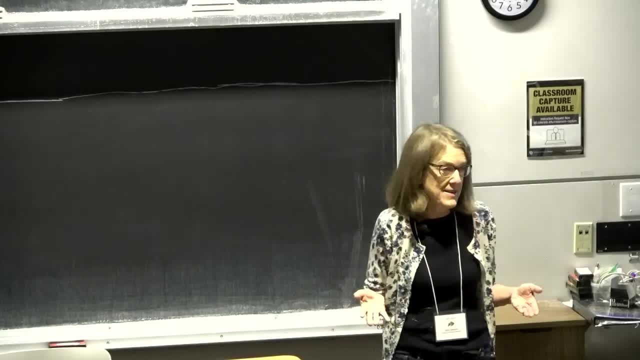 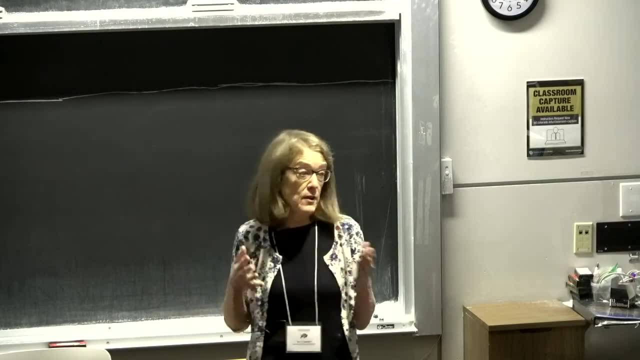 I have PowerPoint slides, which is bad because you talk too fast, but I'm short so I can't write too much on the board. So it would really, really really improve my lectures. if you asked a lot of questions, I'm friendly. 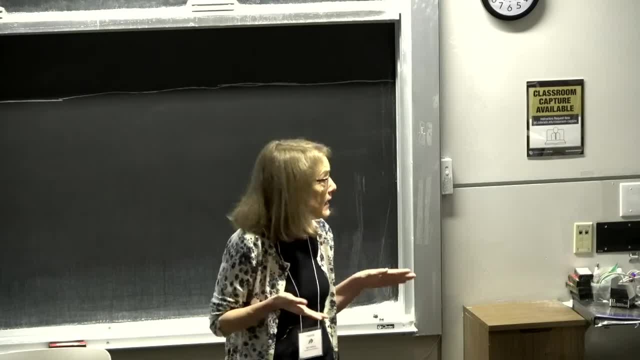 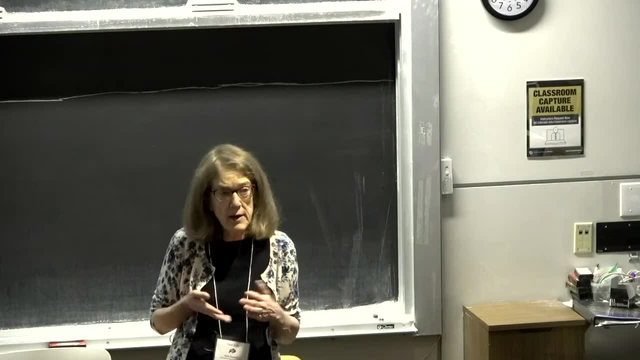 I like questions. Go ahead, Ask me questions any time And, in particular, if you find mistakes in my lecture notes- I hope there aren't any, but there always are- please tell me so I can try to make them better. So. 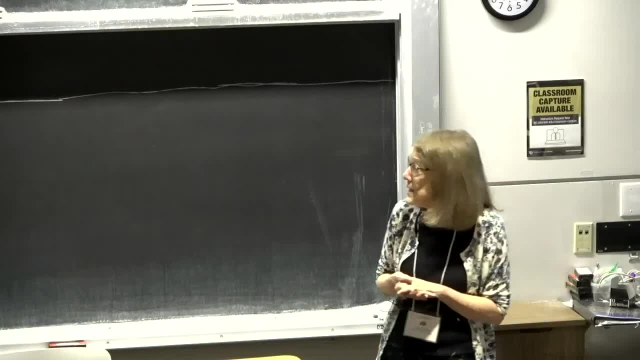 So I'm going to start and talk about the Higgs, and I hope you all have stolen the Higgs Hunter's Guide from wherever you can get it on the web. If you need the two HDM Feynman rules, that's where they are. 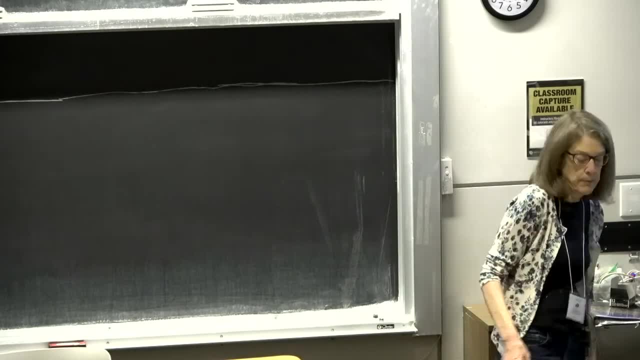 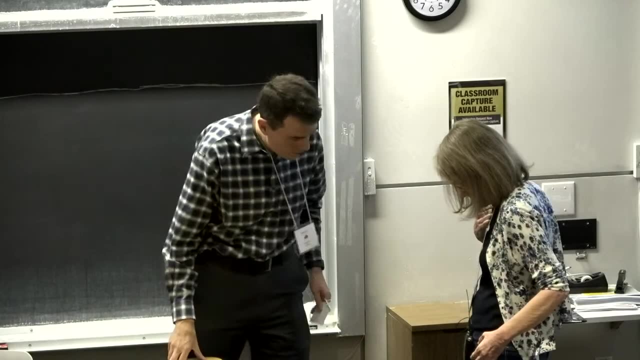 I don't know about the rest of the book, but the two HDM Feynman rules, they're all right. Okay, Yeah, My mic isn't on. I don't hear it. Guys, is my mic on? Hey, AB guys. 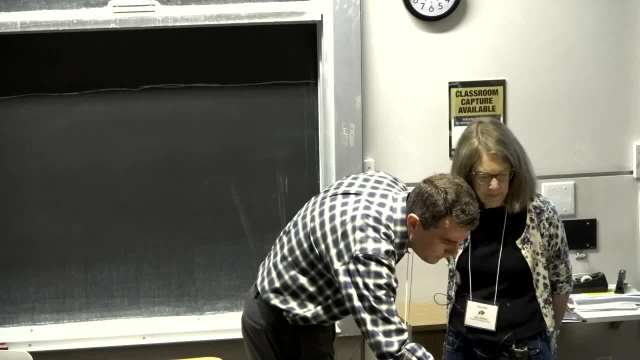 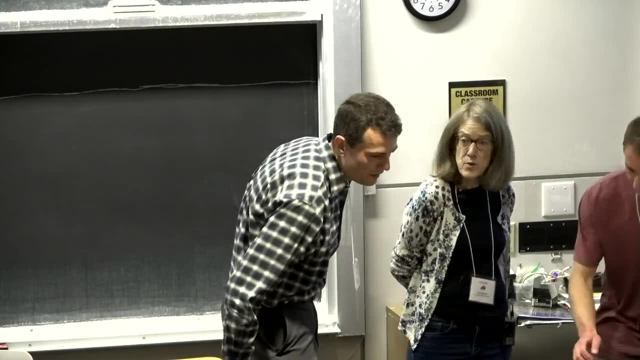 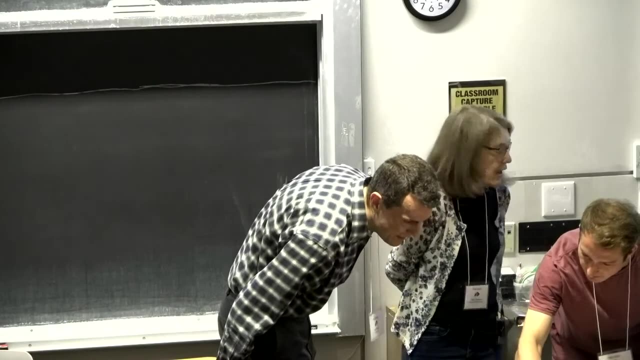 I hear it on. It needs to be a little louder. Maybe I need to be louder. See, that's what happens when you're the first Yep. No, it's me, So I'll keep blathering before I start. So my notes are posted. 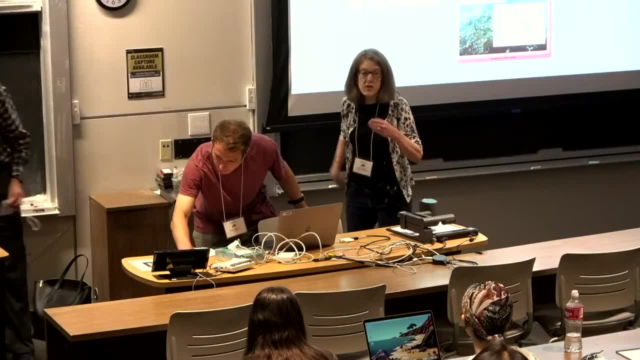 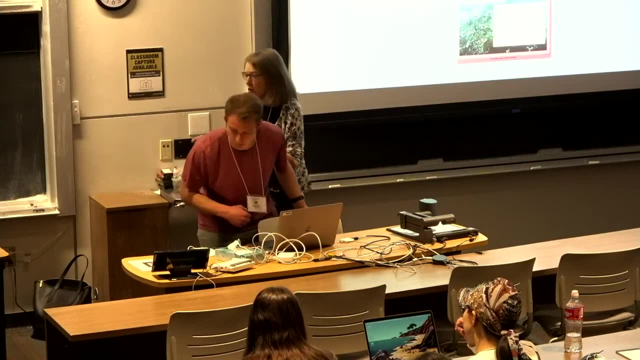 And what I'm going to do. I posted the first set of notes, but I'll just organize each day with what I did that day and then put the next days on So you can look ahead and see what I've got there. It's easier to not have to write down notes. 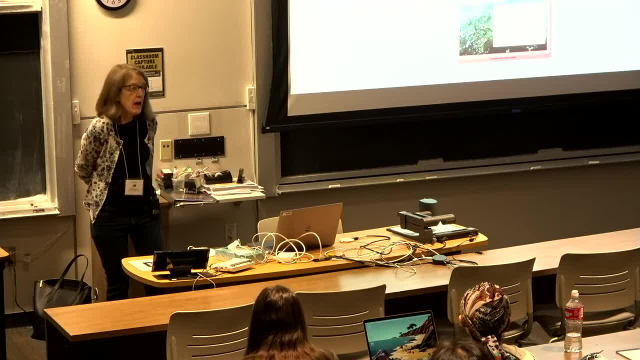 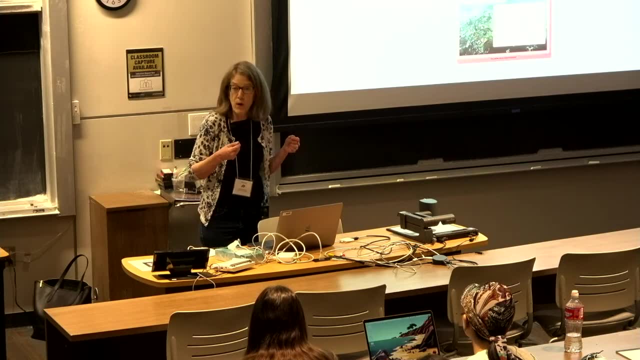 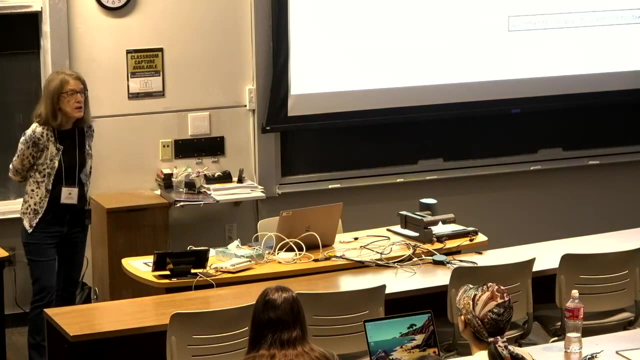 Am I good? Okay, So I'm going to talk about the Higgs boson and also electroweak theory. Do I have a pointer here? Is there a pointer? One more thing? Okay, So the plan of my talk is I'm going to talk about the basics of the Higgs boson and the basics of electroweak symmetry breaking. 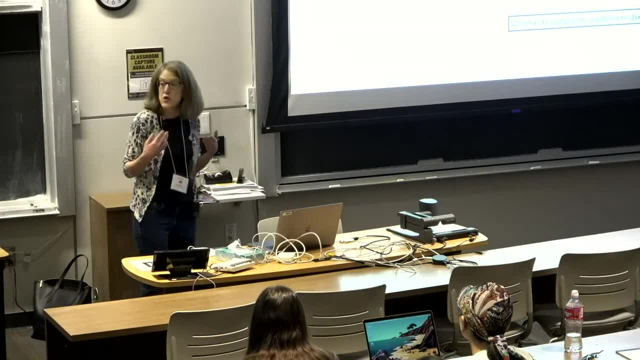 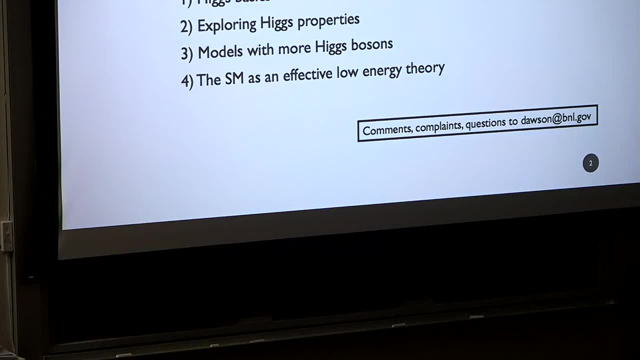 And this will be like kind of a nice exercise. You're probably all suited, You're super good at Mathematica And you can type this into some Mathematica code and go through it and get the W mass, And this is a really good thing to do. just, you know, to see that you understand it. 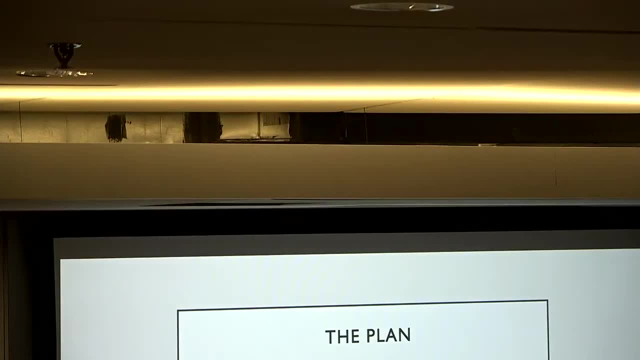 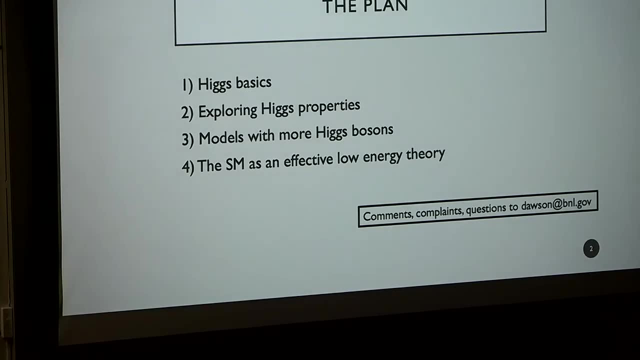 See how all the factors of twos and minus signs and all that stuff works out. And then after that I'm going to talk about the properties of the Higgs and how we explore the Higgs boson properties. What is it that we know about the Higgs? 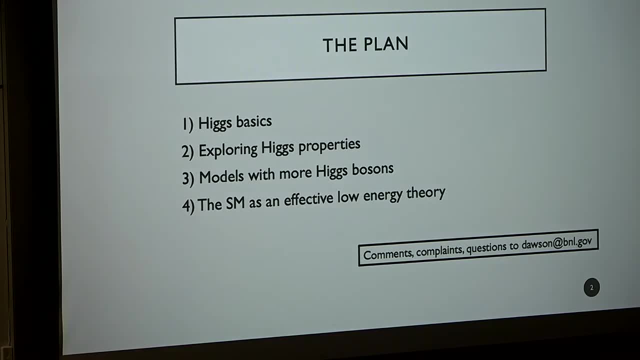 And why am I still talking about it? Why don't we know everything? What do we need to know in the future? And then, probably in my third lecture, I'll talk about models with more Higgs bosons, And my favorite models happen to be models with an extra scalar singlet and an extra Higgs doublet. 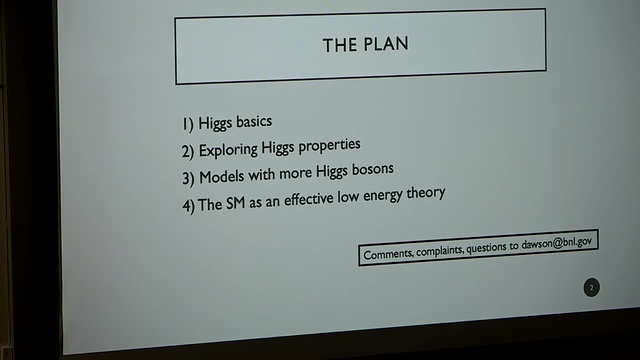 But there are millions of models And these two models will sort of illustrate the general principles of looking beyond the minimal model of the standard model. And then in my last lecture I'll make connections with what Anisha is going to tell you. Anisha is going to talk about setting up an effective filter in the formula. 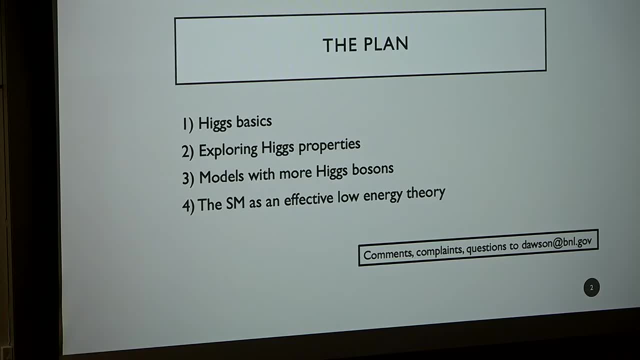 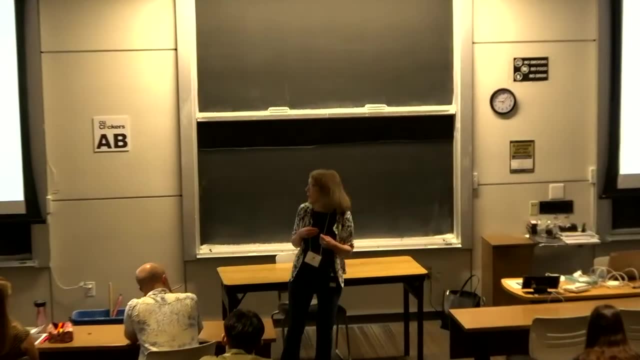 And she's going to talk about the effect of field theory, But of course you can think about the standard model that we know and love- It's just some effective, low energy field theory- and try to learn new stuff by looking at it in this new way. 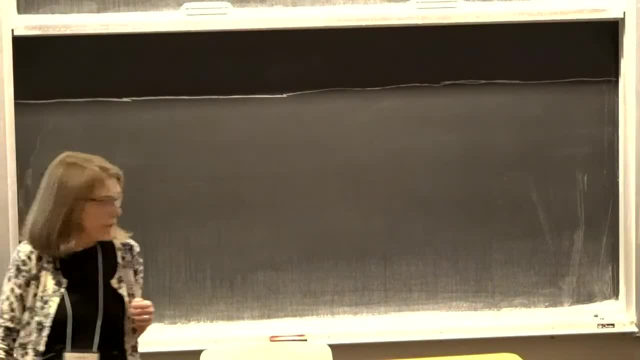 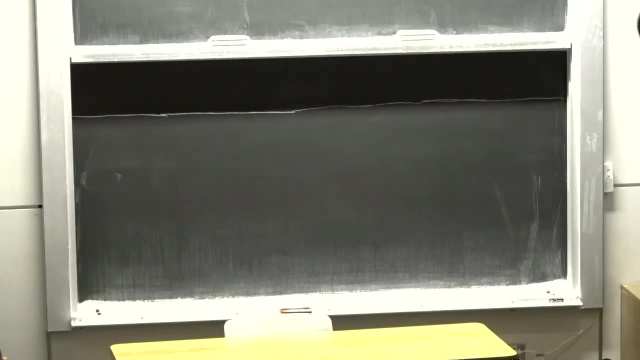 So again, comments, complaints, questions. My email is probably better than the Slack channel, although I will try to respond to Slack. Okay, So in the last decade, the particle physics world has just been completely different from when I was a student. 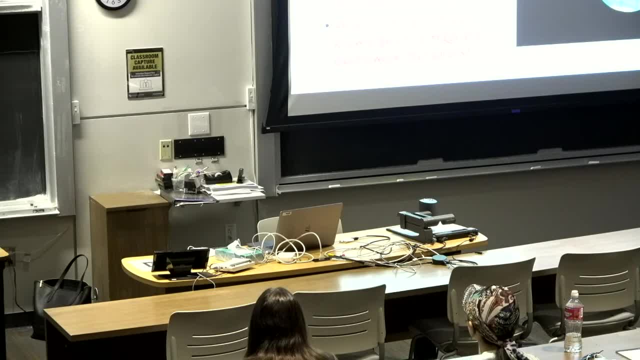 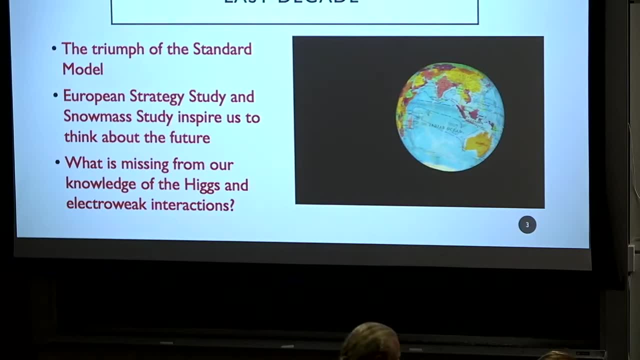 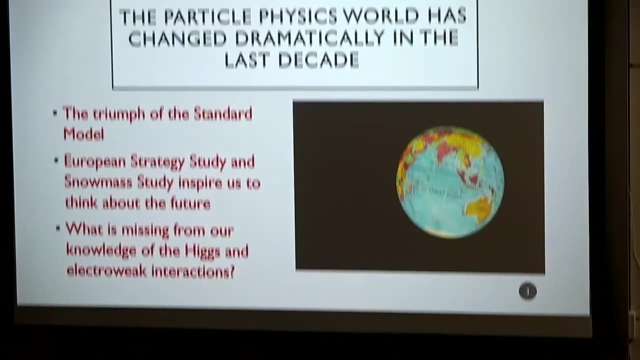 It's just like boom. it's different. We found the Higgs boson Because before we found the Higgs boson, there were lots of models which explained the world without the Higgs And in fact, as I'll tell you probably tomorrow, there are lots of reasons why a standard model Higgs is a lousy object and why it has all sorts of theoretical problems. 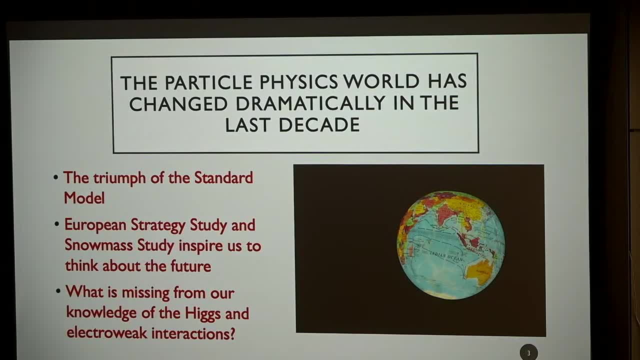 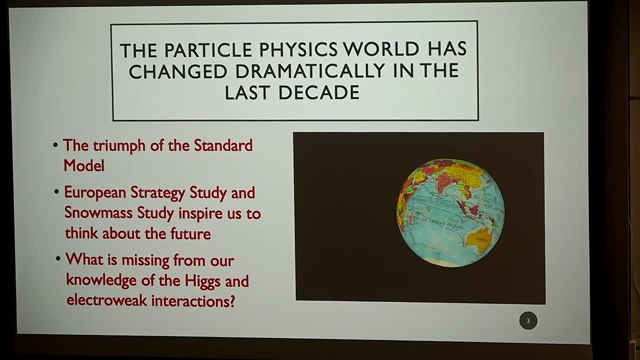 And you know it might not have been there but we found it. And then we found that the standard model, everything works. I could show you plots up the wazoo of calculations, measurements, calculations, measurements, and they all agree. 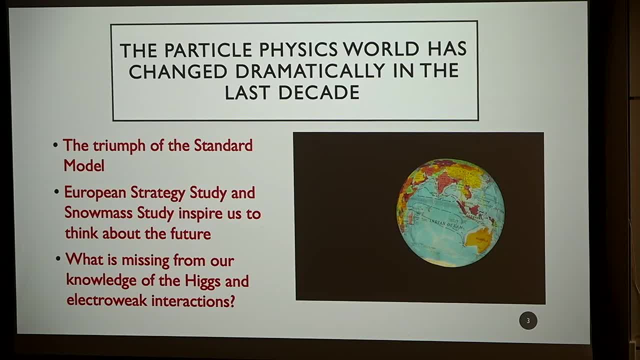 There's pretty much nothing That doesn't agree with the standard model, And this is weird. Everything really agrees. So the question is: how do we know where to go beyond this? And there's been a lot of soul searching in the particle physics community recently. 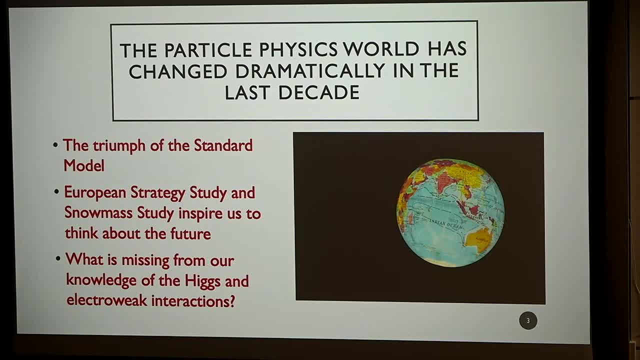 A few years ago, the European community gathered together to think about their future beyond the LHC And, as many of you probably know, the recommendation was to build what's called a Higgs factory, a high-energy E plus, E minus machine that would study. 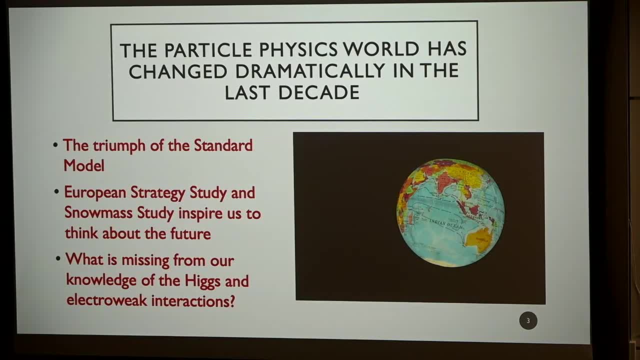 All the properties of the Higgs. So that tells you that we really got to understand the Higgs boson And we really have to understand why would I spend umpteen billion dollars and umpteen years measuring everything there is to know about the Higgs? 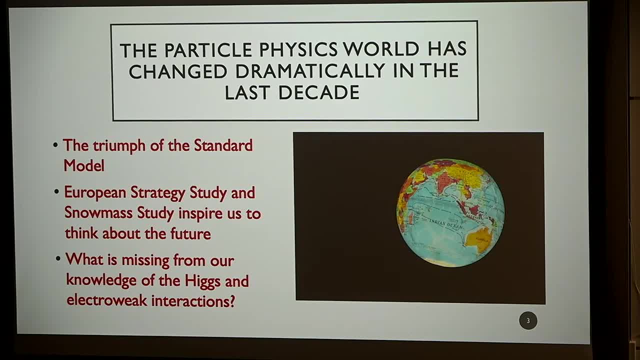 And this is a really serious question for your generation to answer. So what is it that we're missing? And at the moment, as we speak, the US community is undergoing what we call our snowmass process, where we gather together to make a plan for the US community. 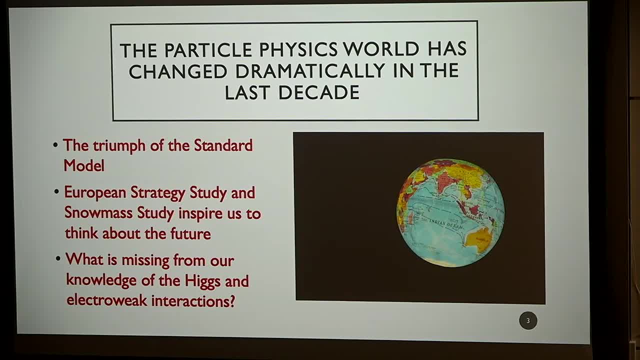 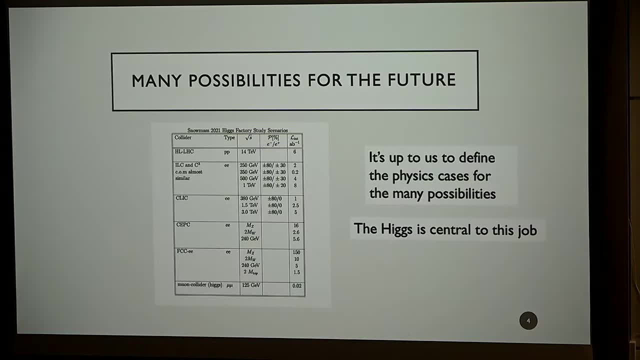 Where are we going? So how does the Higgs feed into our future studies? Okay, So before I start talking about the Higgs, let me talk about the possibilities. I say for the future, but it's really for your future, It's not for my future. 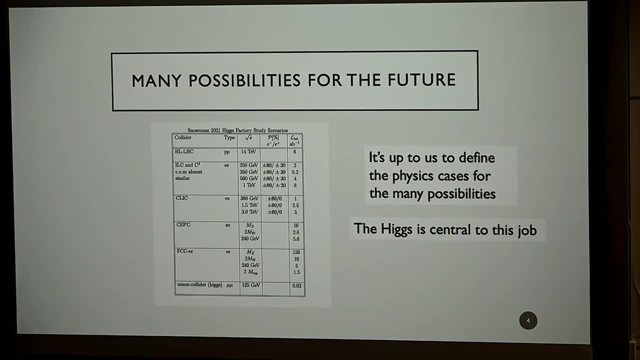 It's for your future, because these are very, very long-term projects we're talking about. So at the moment we have the high-lumine LHC. I'm looking for a stick or some kind of point. Okay, well, we have the high-lumine LHC, which is the top line here. 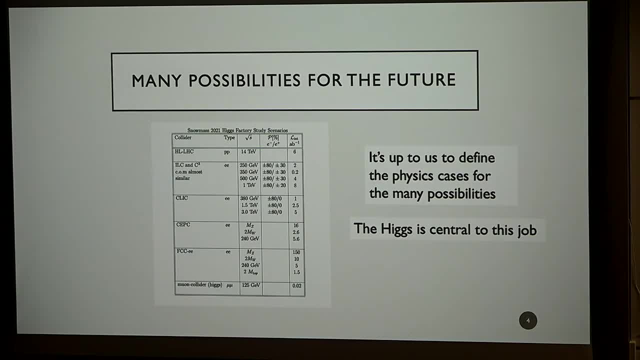 Proton-proton collider at 14 TeV. There are no plans to upgrade the energy of the LHC, So 14 TeV is what we have, But there are plans to run it longer and longer And you'll notice, on the far right there it says six inverse adobarns. 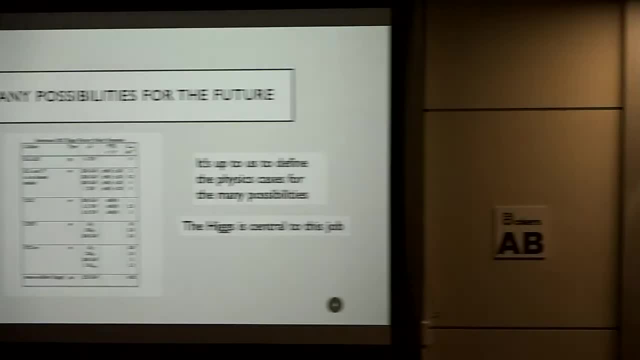 So that's really the 20-year plan. The plans that we had a few years back were three inverse adobarns, But we're not going to run it longer, We're going to run it longer. We're going to run it longer. 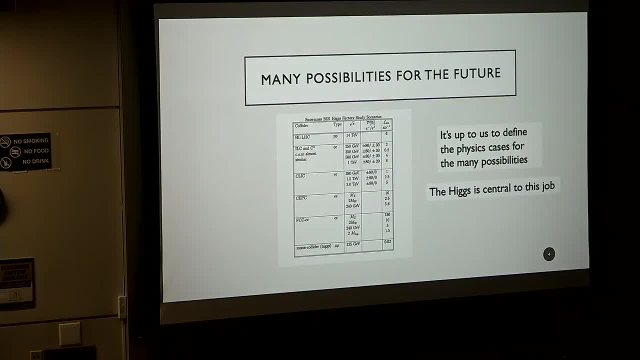 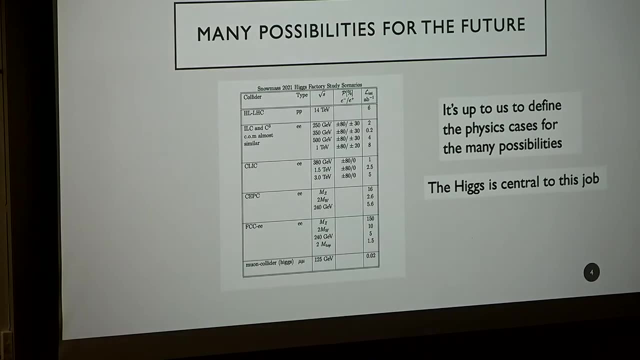 We're going to run it longer, But we can just keep running forever until the detectors fall apart. So that's the 20-year plan. That's maybe your 10-year plans. shall we say, You guys are mid-career scientists at that point. 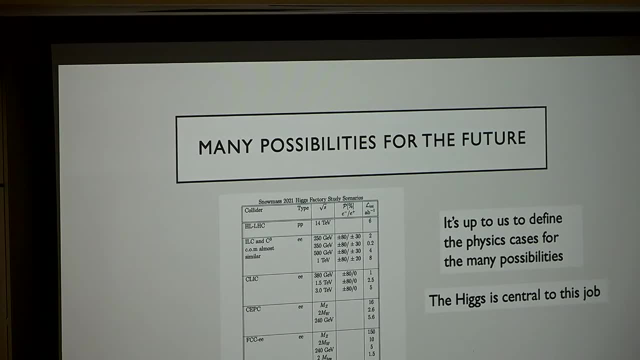 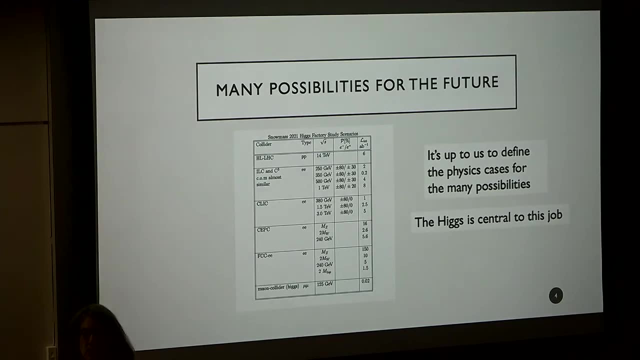 I'm retired. And then there's a whole host of E plus, E minus machines. There's the ILC, which is an E plus, E minus machine that we've been talking about for 20 years, 30 years, a very long time. 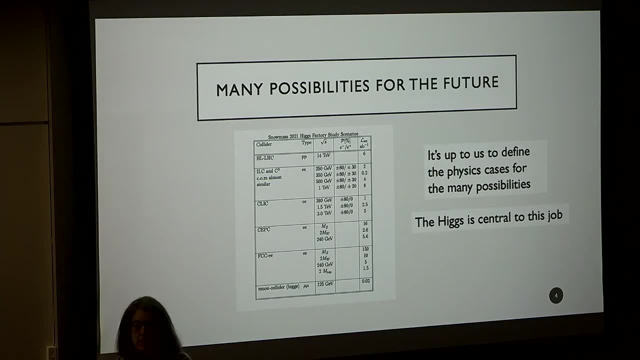 And the ILC would run at 250 GeV And as I talk about the Higgs, you'll see that this is not a random energy, but 250 GeV is the energy where you get the best Higgs measurements, And you'll see that. 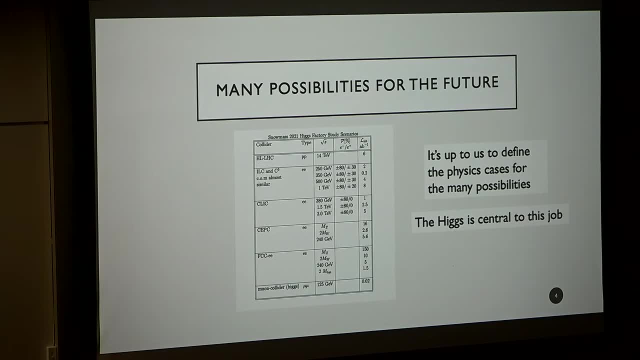 I'll show you plots of cross-sections. It says, aha, that's the right energy. But then you see that the ILC is predicted to step through energy. So the next energy is 350 GeV. So anybody want to tell me why that's good? 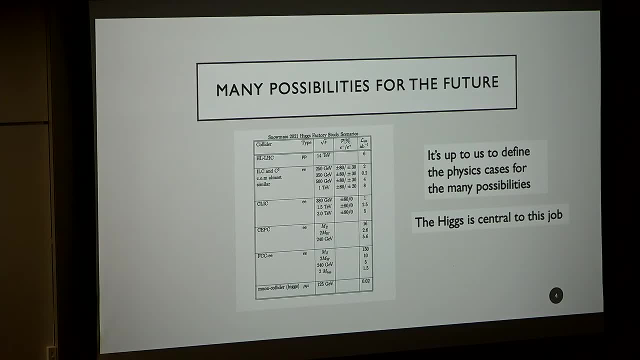 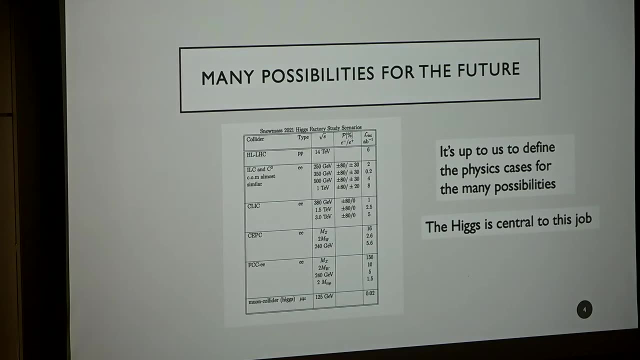 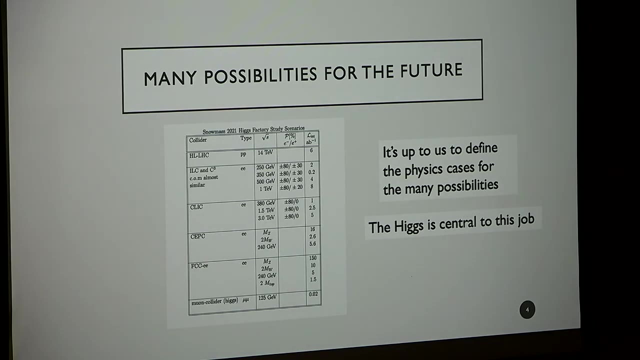 What's special about 350?? Yes, you can make two tops right. The top mass is 175.. So after we've measured everything we want to know about the Higgs, then we'll go to 350, and then we'll measure the okay. 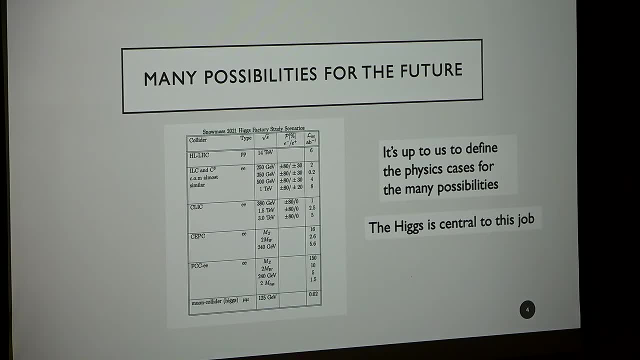 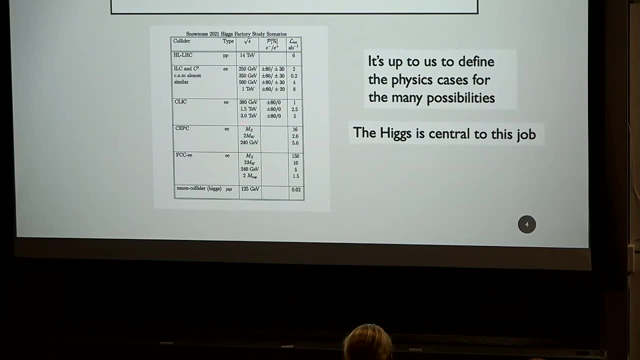 and then we'll measure the TT-bar and then we'll keep going to 500 GeV and a TeV to higher energies And you'll see the next machine, Qlik, is proposed to go up to 3 TeV in E plus, E minus. 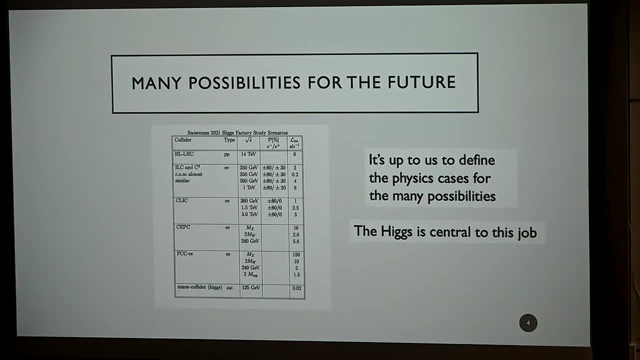 CPC is a Chinese E plus, E minus machine. And finally there's a muon collider here. This would run on the Higgs resonance to start to measure Higgs couplings and then perhaps go to higher energies. So we've got a whole lot of plans for machines which are designed just to measure Higgs properties. 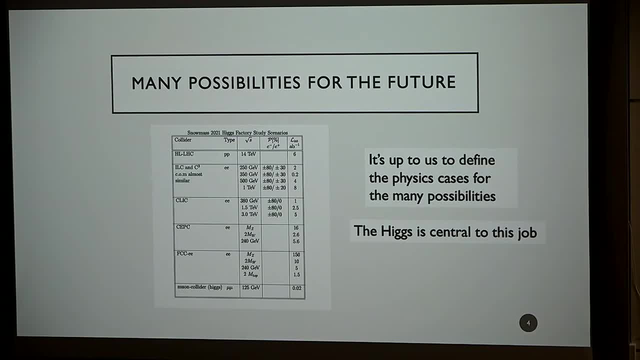 Yes, Oh, why is it only 0.2 inverse out of arms of the TT-bar threshold? Oh, because, okay, that's a good question- You measure the Higgs couplings with a lot of luminosity, Right, Because you want the Higgs couplings really precisely. 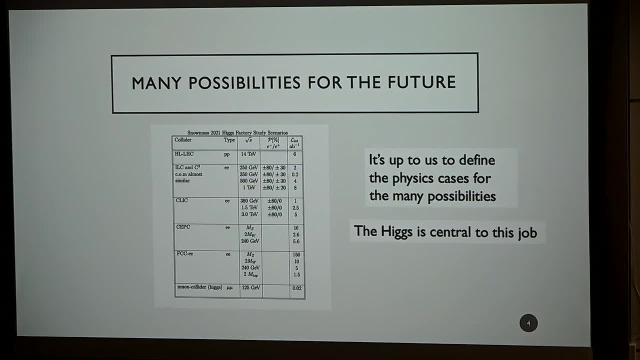 because BSM models are going to predict that maybe the Higgs coupling to Bs is a little bit different, So you need a lot of luminosity. 0.2 is just enough to do a threshold scan and get the top Hort mass very precisely. 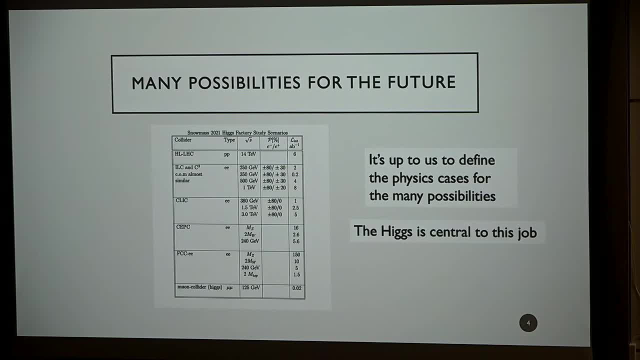 So that's all you need for the top mass. You can see here that the different machines, they keep changing the luminosity depending on you know some projected desires. I mean, I don't think this is fixed in stone. Okay, so it's up to us to define these physics cases. 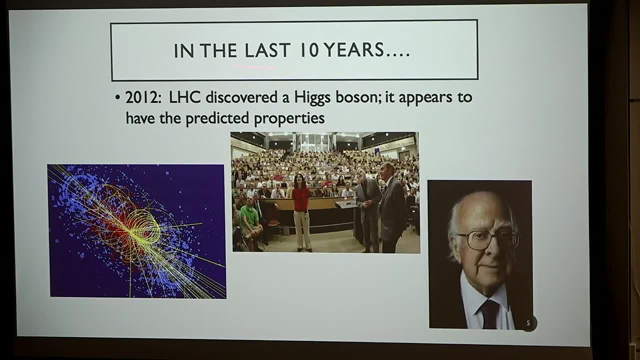 Okay, so here we go, The pretty pictures of finding the Higgs. Here's the discovery announcement. You've all seen this. This is an ATLAS display, Peter Higgs. So we found the Higgs boson a decade ago. 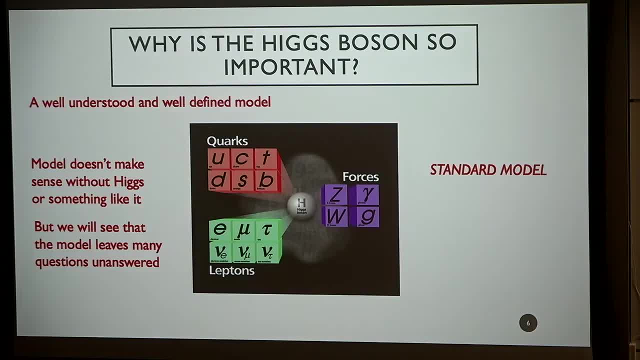 and everything we know about the Higgs is kind of standard model-like. So we have to ask: why is the Higgs boson so important? And the reason it's so important is because we have the standard model. It's important because we have the standard model. 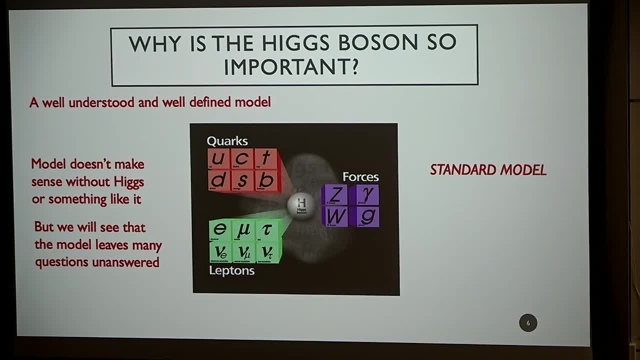 which is well-understood and well-defined and, as I said, well-supported experimentally. So we've got the standard model with the quarks and the doublets here, up down charm's range, top, bottom. We've got the leptons here. 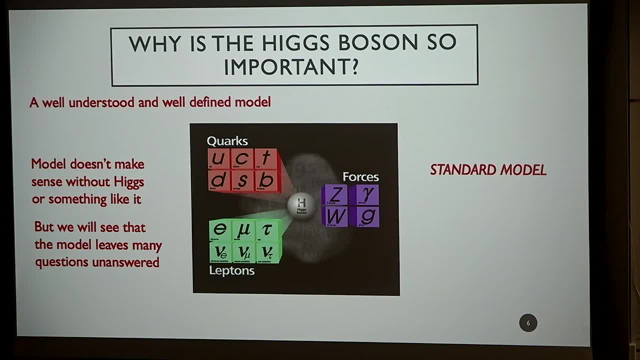 We've got the force carriers over here and the Higgs, But this model, as I'm going to claim in the next few lectures, it leaves a lot of things unexplained and it makes absolutely no sense without the Higgs. If you remove the Higgs from your model, it doesn't make sense. 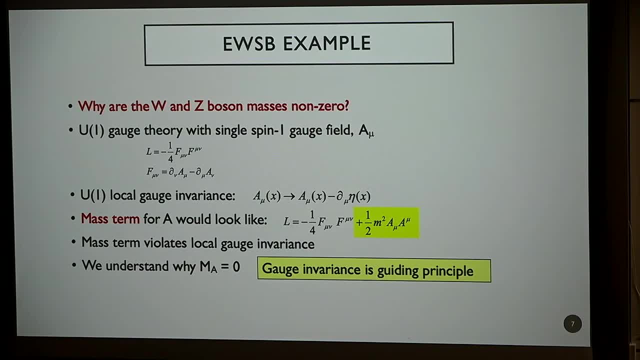 So let's start with doing some physics here. Enough background. So here's a really simple example of electroweak symmetry breaking. We notice there are four force carriers: There's a photon, there's a gluon, there's a W and the Z. 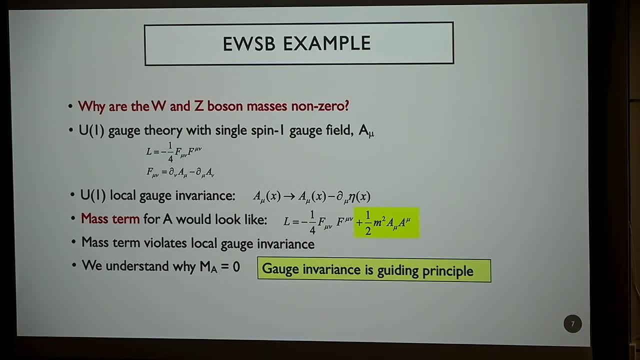 And the photon. we know that its mass is zero. very, very precisely They measure properties of light coming from the sun, So its mass is zero. We know the gluon mass is zero- Not as precisely as the photon mass, but we know it's zero. 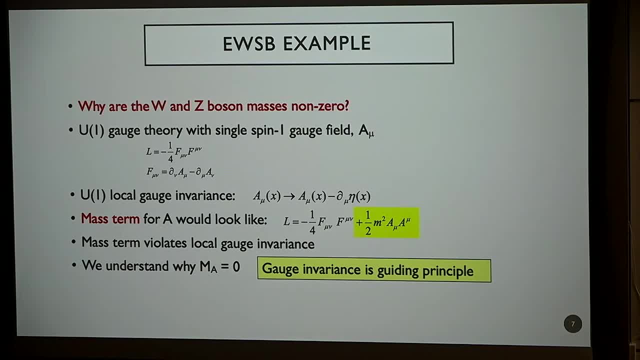 So the question is: why are the W and Z? Why is the gluon mass is not zero? So let's start with a simple example, a U1 gauge theory with a single spin-1 gauge field, which I'll call L. 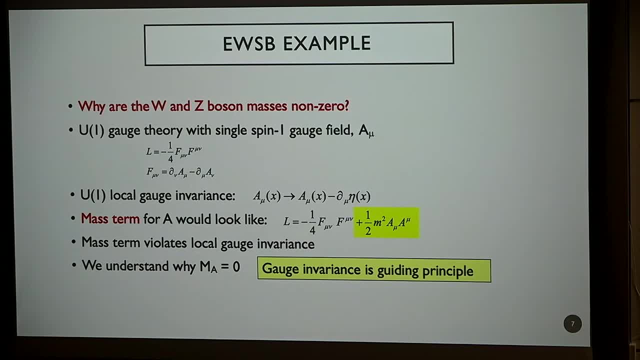 And this is quantum electrodynamics. So the Lagrangian is just F mu nu, F mu nu, and here we have F mu nu. It's just the covariant derivative here. So this has what we call a local gauge invariance. 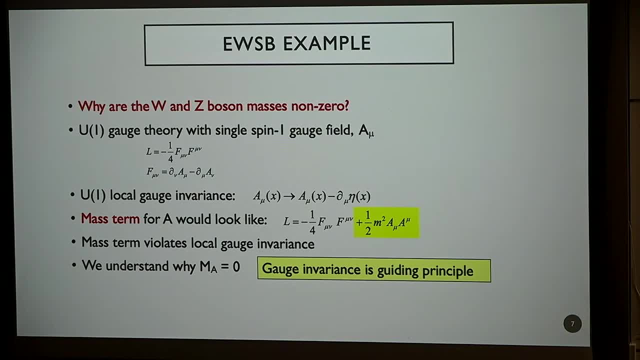 So I can make a transformation on my gauge field, shifting it by the derivative of any function: d, mu, A to X. So that's fine. So my theory has this gauge invariance, But if I wanted to add a mass term, 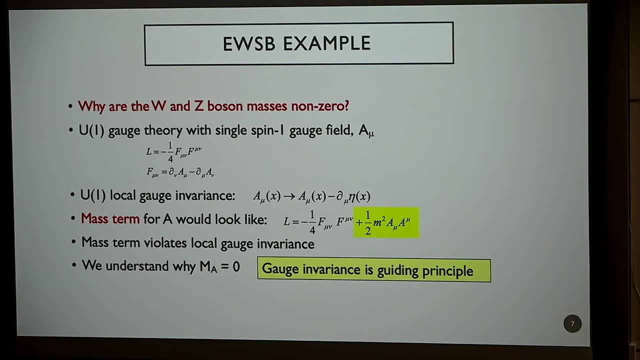 is this distracting when I go back and forth? It probably is right. Yeah, You're saying yes, OK, I'll pick one side. I'll pick this side today and that side tomorrow. So a mass term for the A for the photon. 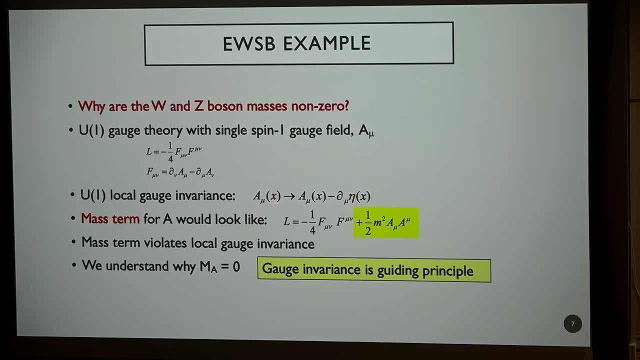 would be M squared A mu, A mu. So you know already that if I add a mass term it violates gauge invariance. Bingo, I can't have a mass term for my gauge fields. So we understand why the photon is zero. 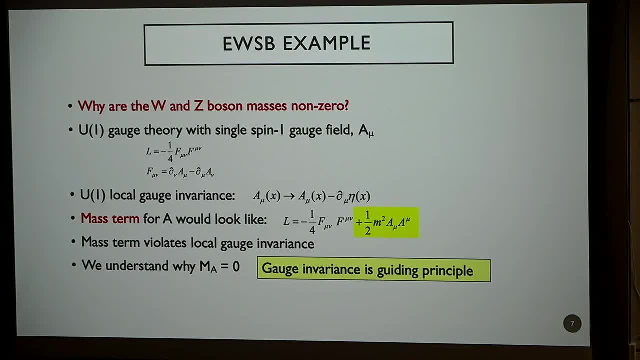 So the whole basis of this, of our theory, is going to be gauge invariance. Our theory has to be gauge invariant, So we cannot add a mass term for the W and Z, because it would violate our gauge invariance. What about Stuckelberg? 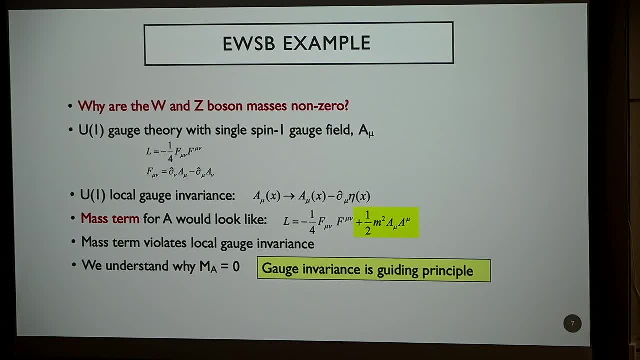 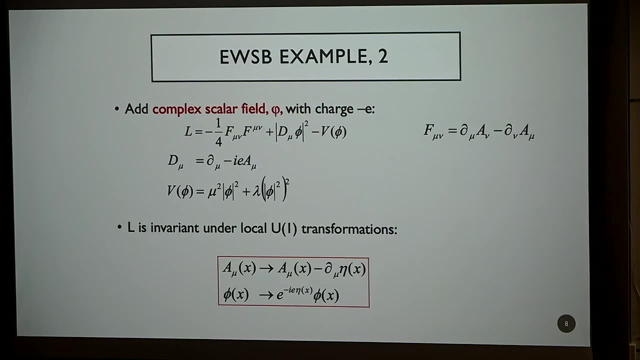 What about what Stuckelberg mass term? That's another story. We can talk about that one later. Sorry, But yeah, That would derail me. So we can add a scalar field phi with this charge E to the theory. 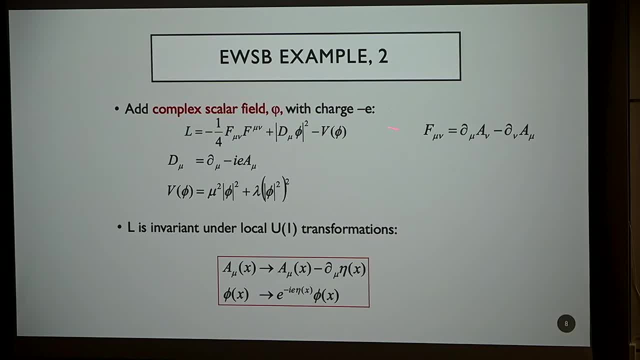 And we can still have gauge invariance. So we have the same theory with our scalar field. So we just have d mu phi minus some potential. I'll write down the most general potential. So this is just a U1 theory. So my most general potential is mu squared. 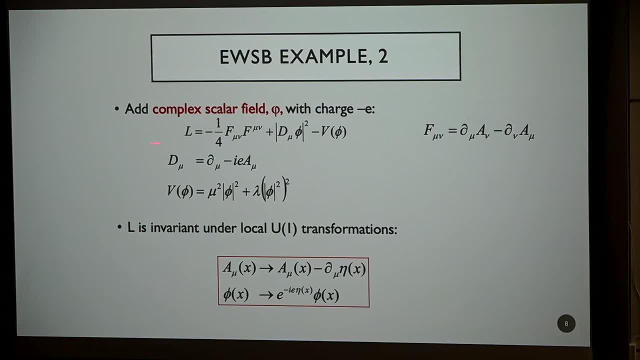 phi squared lambda phi to the fourth. It's got this covariant derivative And again the theory is invariant under these local U1 transformations. So I can transform A by a derivative and phi by a phase here And it's instructive to actually do this. 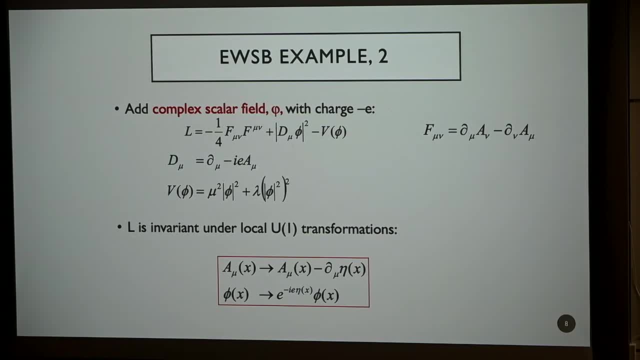 with the Mathematica code and see that this construction preserves gauge invariance. So here we go. We have the most general thing we can write down that's invariant under these local U1 transformations. But what happens when we do this? Well, I've got two cases. 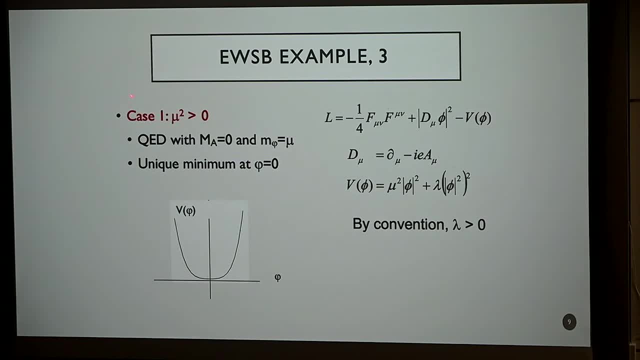 I've got this mu squared, the mu squared and the potential positive. So here's my potential. It's just a quadratic equation here: Mu squared, phi squared, lambda phi to the fourth And by convention we'll take lambda to be positive. 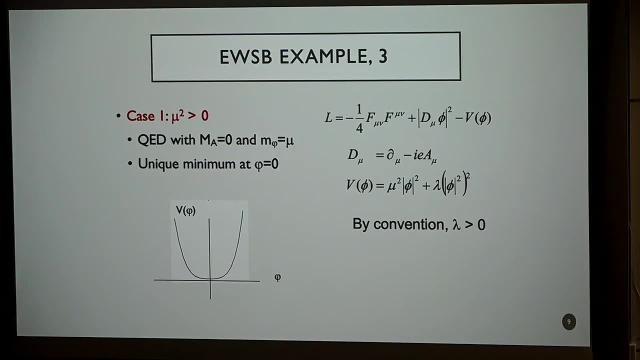 So this is just quantum electrodynamics with a massless photon and a scalar field, mu. So when this happens, there's nothing particularly interesting that happens. But what if, for some reason, mu squared were negative? And I'm going to say, we just postulate this. 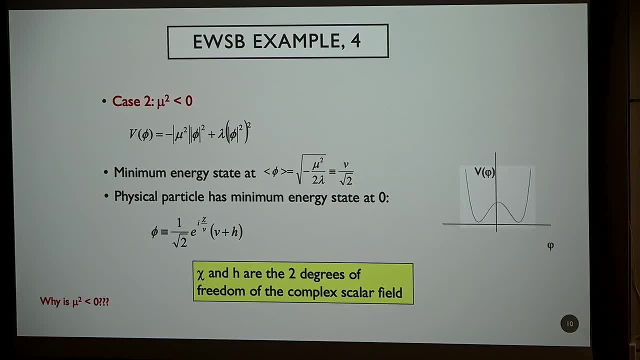 I wrote down here. why is mu squared less than zero? Well, supersymmetric models can kind of explain this, But in general we don't have a clue why mu squared is less than zero. But if it is less than zero, something deep and profound happens. 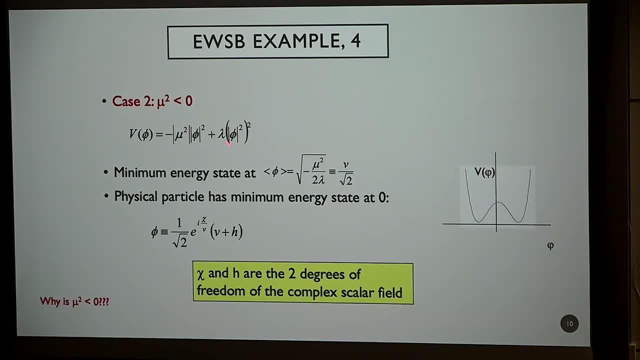 If this term here, where I put the absolute values, just to remind us, if this term here has a minus sign here, then the potential looks like this: And physical states always have their minimum energy at zero. That's just quantum mechanics. 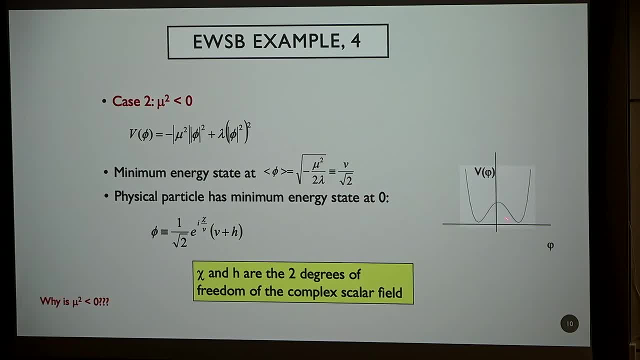 So the minimum energy state is not at phi equals zero, but it's at phi equals v over square root of two, And this is the definition of v. So minus mu squared over two lambda. And why is there a square root of two there? 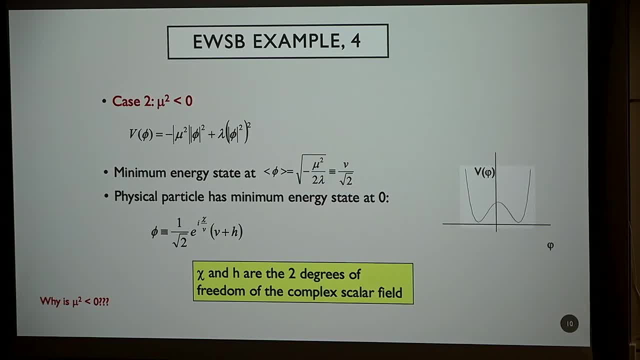 And it's just to screw you up, It's just to confuse you. It's put in by hand, There's no physics in it whatsoever. But this square root of two is here, by definition, by convention. It used to be. sometimes people went back and forth. 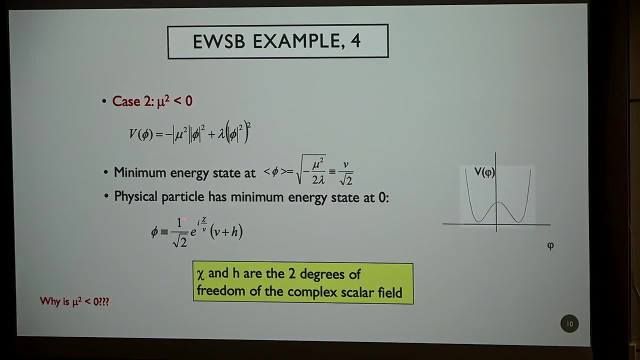 but now everybody does it this way. So the physical particle has its minimum energy state at zero. It's right here. So the physical particle- I'll call it h- is just v plus h. So we define our scalar field to shift it away. 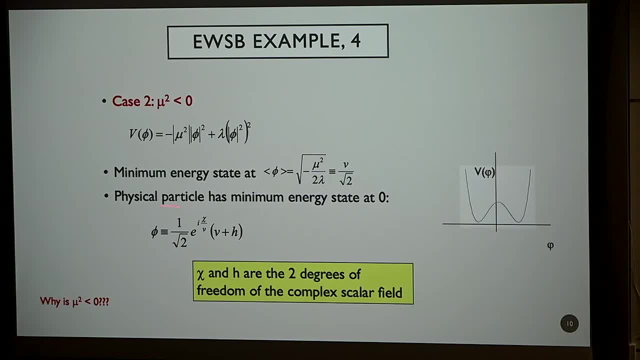 so h has its minimum at zero. And then the other dimension of our complex field I'll call chi and I'll just put it in a phase. So chi and h are the two degrees of freedom of the complex scalar field. So we've got a physical scalar. 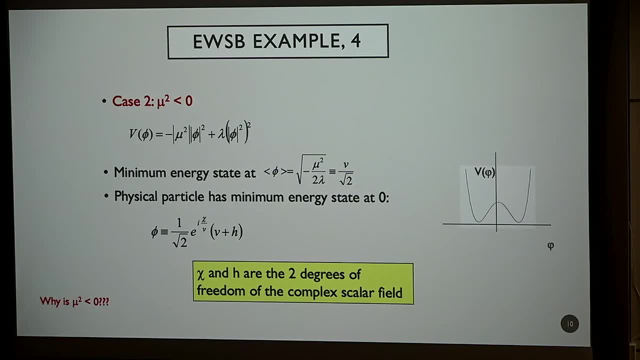 and we've got this thing, chi. And of course you all think: well, this is trivial, She hasn't done anything at all. right, All I did was say the mu squared is negative, and I did a little bit of algebra. 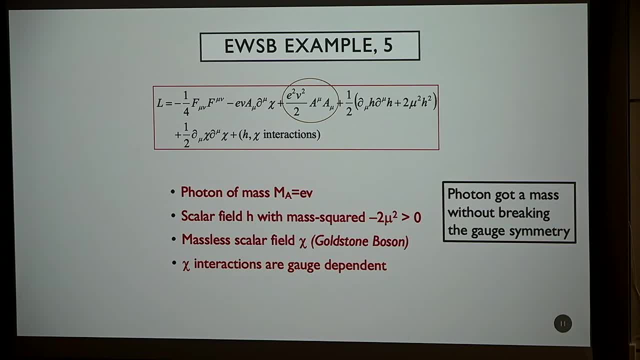 But what happens is truly amazing. and this is the miracle of electroweak symmetry breaking. So you just go put in this phi field into your potential and do your algebra and what happens? You've still got your gauge fields, but now you've got a term: e squared, v squared amu, amu. 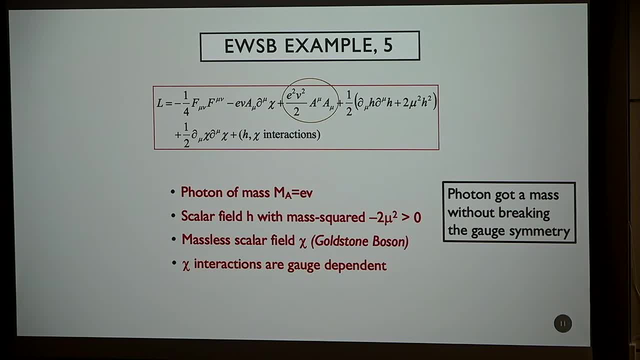 So, because of this spontaneous symmetry breaking, you have generated a mass for the photon field. So here we go, Here's the mass. And the mass is predicted in terms of this parameter v. So it's e squared v squared over 2.. 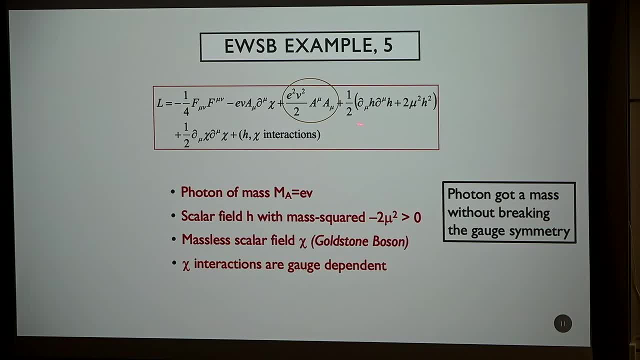 And then just doing algebra, no trickery. here we have the Higgs field, d mu h, d mu h. So this has a kinetic energy term here. So it's a propagating field. It has a mass term here, with the correct sign. 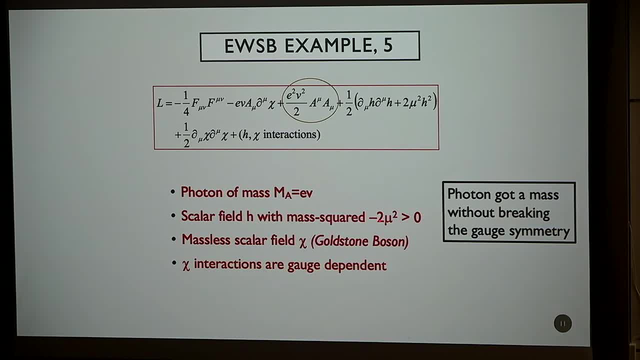 So it's a scalar field with mass squared minus 2 mu squared. Remember mu squared is negative. It's got this massless scalar field, chi, which is what we call the Goldson boson. So these chi interactions are gauged. 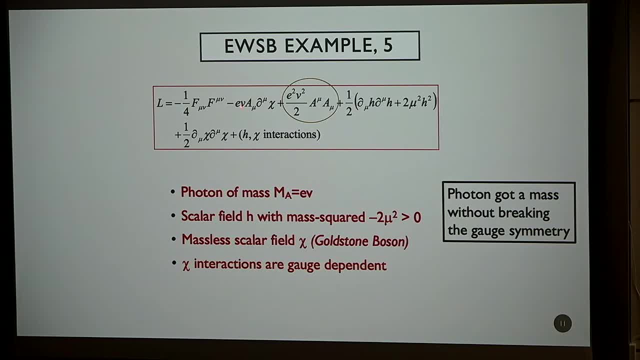 And what do I mean by that? Look at this term here. This is a funky term. It mixes the photon field with this Goldson boson field. So we can redefine the A field to what we say, gauge away the chi field. So if I redefine the A field, 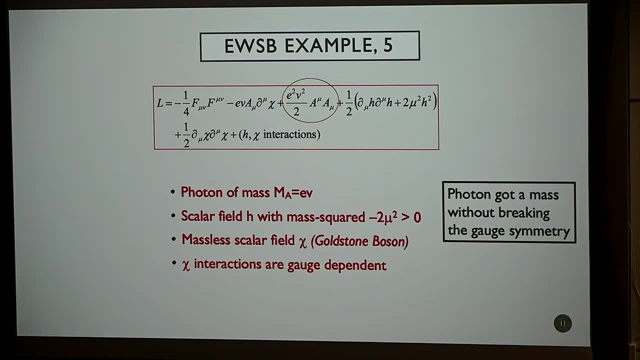 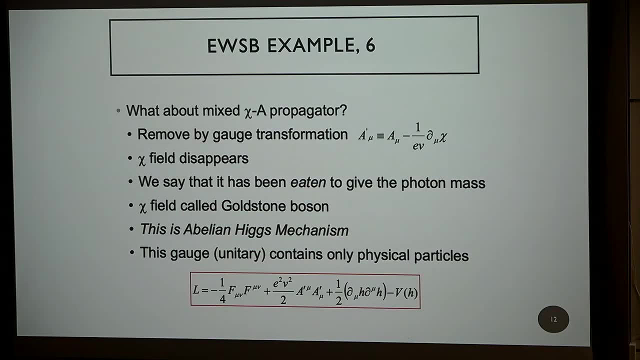 I can get rid of this term so that I don't have this mixed propagator. Okay, So this is the end of this simple example here. So we'll remove this mixed propagator here by shifting the gauge field like this with the d mu chi: 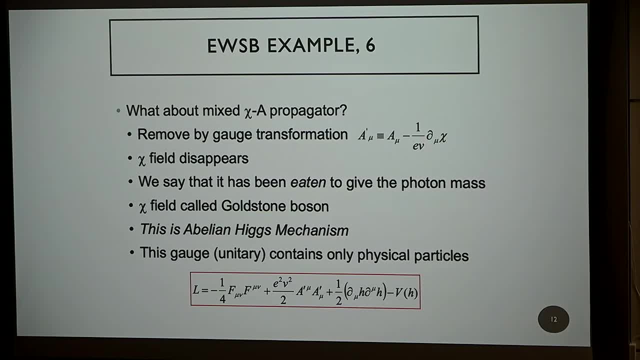 And when I do this, the chi field disappears And we say that it's been eaten to give the photon mass. That's the standard terminology, But it's really just a gauge transformation, a redefinition of my scalar field, And so this is what's called the Abelian-Higgs mechanism. 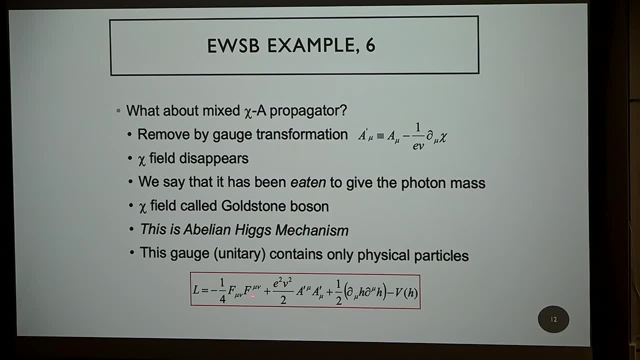 And so this gauge has only physical states. So the Lagrangian has a scalar field which is an F mu nu. F mu nu- It's got the mass term for the photon. Here we go, And it's got a propagating Higgs field. 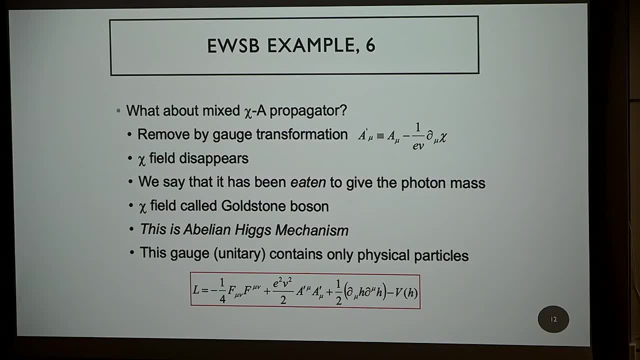 And you can work out the potential just by algebra. So any questions before I continue? Yeah, I mean it has d mu h, d mu h. It's just got the correct kinetic energy term, Right, If it didn't have this term? 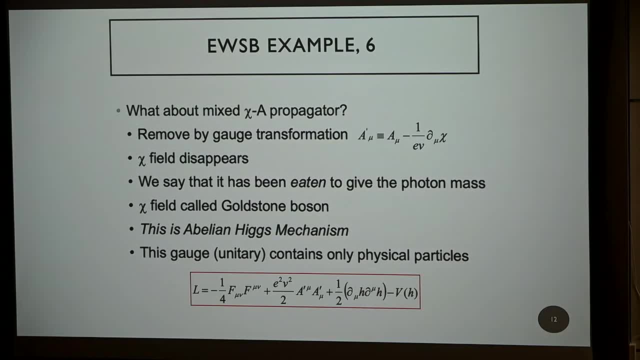 it wouldn't propagate. I wouldn't be able to write it as a physical field, It would have no kinetic energy. Yeah, What do you mean? there are only physical states Because there are some A's that have negative mass. No, Everything has a proper mass term. 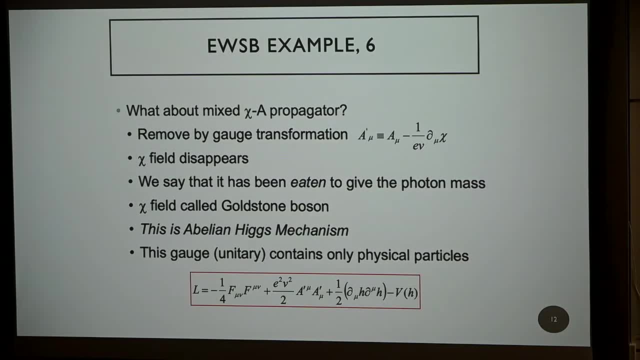 The signs of the mass terms are the correct signs. Yeah, That's what I mean. So you have this A field. It's got a mass term with the proper sign. I could go look for it. It's a physical thing. I've got the H. 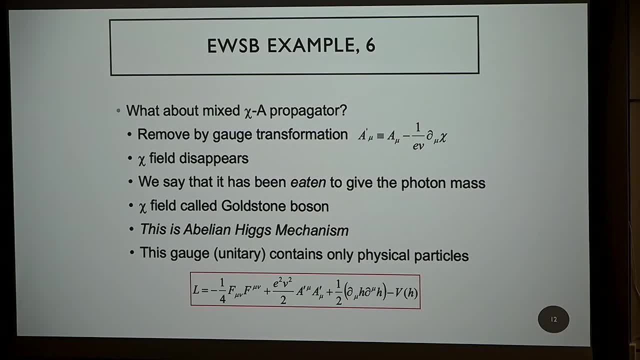 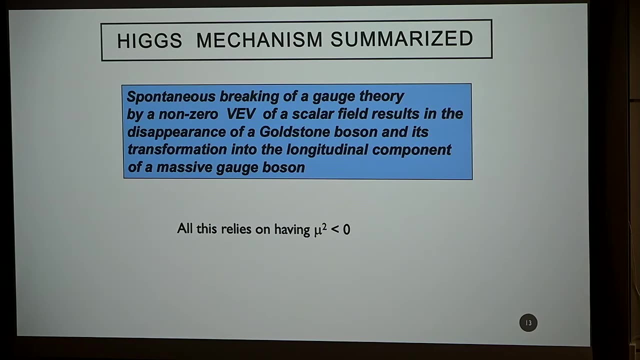 It's a physical thing. I've got the potential here, which is just algebra from back, a few slides And I can calculate its interactions And that's it. So this is very nice. So this is spontaneous symmetry breaking. It comes from a non-zero vev of a scalar field. 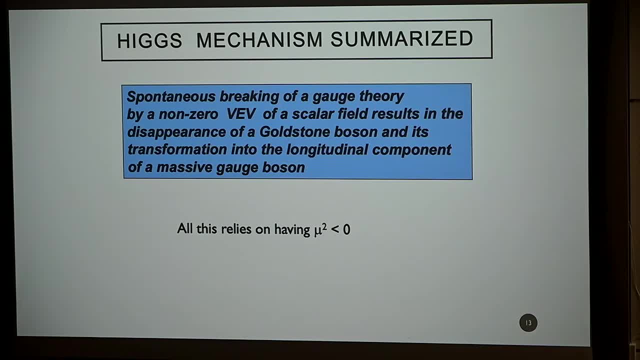 and then results in the disappearance of the goldstone boson and the transformation into the longitudinal component of a massive gauge boson. So what do I mean by that statement? So remember quantum electrodynamics, the photon. You know how many degrees of freedom a photon has, right? 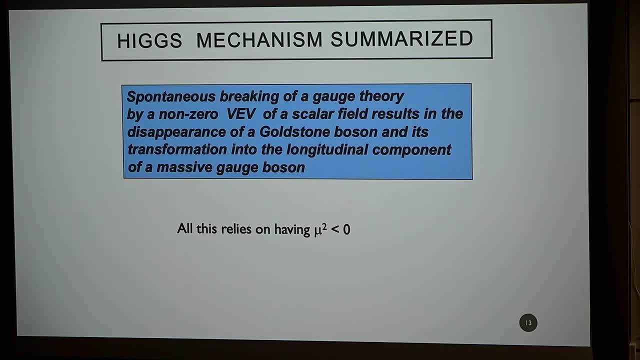 Two. Good, It's got two transverse degrees of freedom. It does not have a longitudinal degree of freedom. A massive gauge boson has a longitudinal degree of freedom. So when I give this A field, a mass, it acquires a longitudinal degree of freedom. 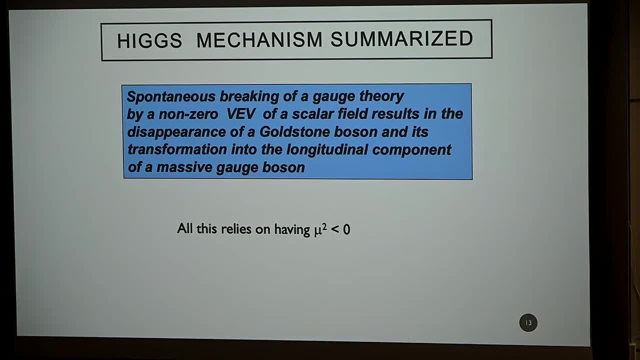 So all the exciting stuff about Higgs, physics and spontaneous symmetry breaking, all the cool stuff is going to be in this longitudinal degree of freedom which you didn't have without the spontaneous symmetry breaking. And then here's this caveat: You've got to have mu squared less than zero. 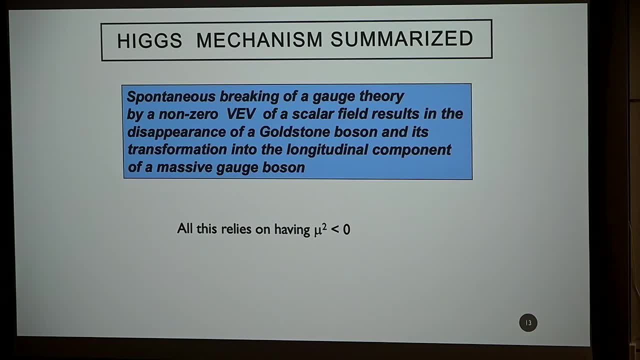 It all relies on this magic that this one term is negative. So, as young scientists, you should continue to think about this problem with theorists that have been thinking about it for generations. Yeah, So you said there are potential SISI explanations for mu squared being less than zero. 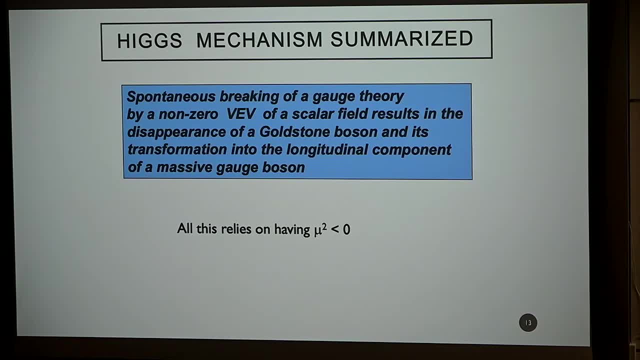 Yeah, You want to hear them. So if you have a grand unified, supersymmetric model, so way up at the Planck scale you've got a model, and Gigi's an expert in this. I'll pin you. So if you have questions. 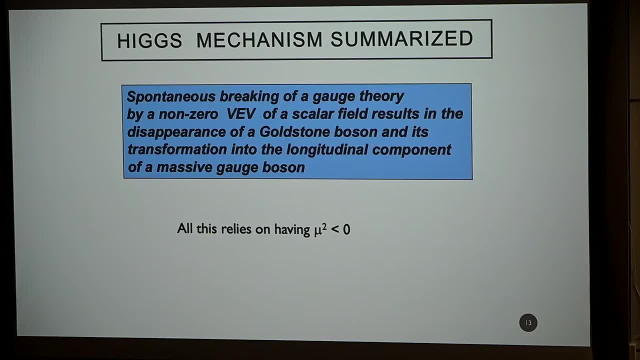 you can ask her. But if you have a grand unified model at 10 to the 16th G of E or something with a very small number of parameters in your supersymmetric model, your supersymmetric model relates all sorts of different things, So then you evolve everything down. to the weak scale, And Michael Dine did this in 1977 or something years ago. You can show that mu becomes negative in these models as you evolve it down due to renormalization group running. So this simple supersymmetric model which does this is now ruled out experimentally. 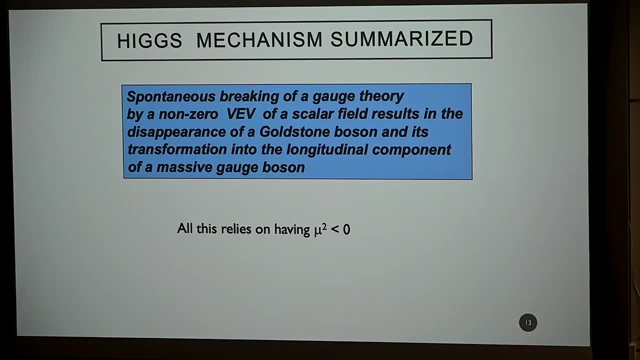 But it still was kind of a nice motivation that maybe there's something there- And actually I should continue with that. When Michael Dine wrote this paper where he's evolving the supersymmetric parameters down and getting mu less than zero, it only works if the top quark is about 175 GeV. 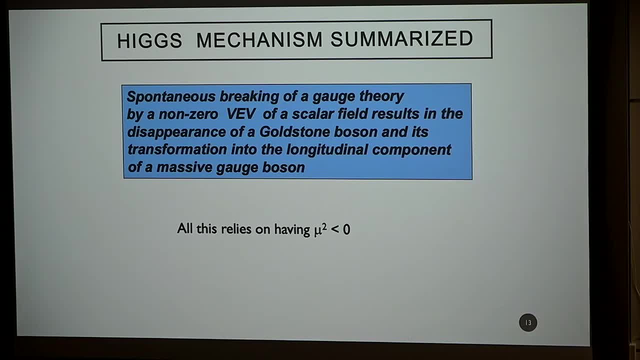 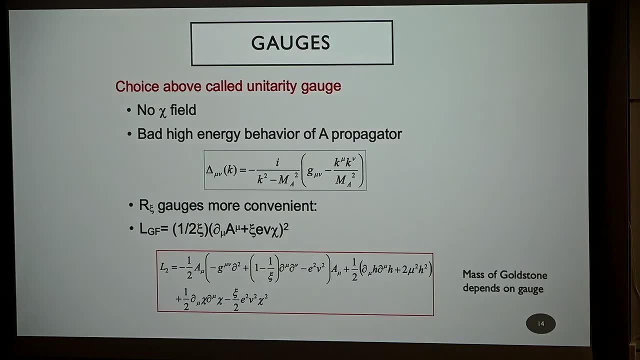 And this was way before they found the top quark. So that was actually something kind of cool, making you think that there might be something there. Okay, let's see here. Okay, so an aside on gauge fields. I made this transformation. 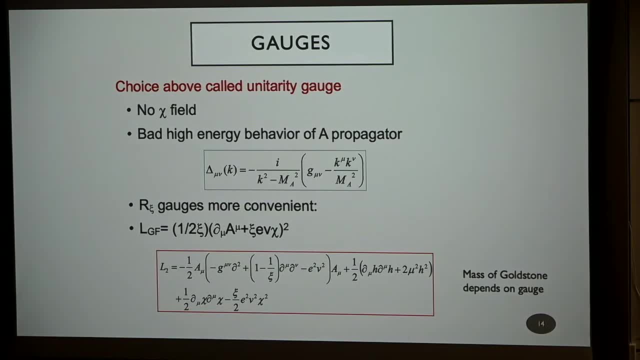 to get rid of the chi field. But this particular gauge is not very nice for calculations because if I calculate the propagator of my A field it's got these terms: K, mu, K, nu, over M squared And terms which grow with energy. 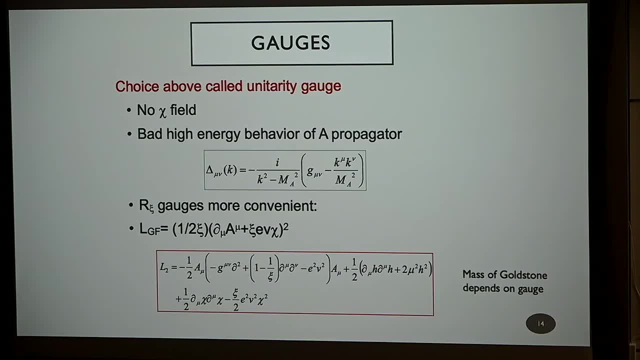 are very bad from a theory point of view. I will show you later today and tomorrow that when you have effects growing with energy, you tend to violate what's called the unitarity bound And such theories tend to run into trouble. So you can of course add gauge fixing terms. 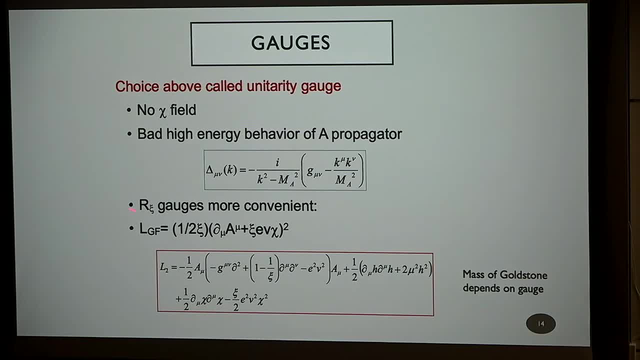 to change your gauge, And the gauge we mostly use these days is called RC gauge, which is just making this transformation Again. it's just putting it back and doing the algebra which I strongly recommend that people do: some algebra And you get a term. 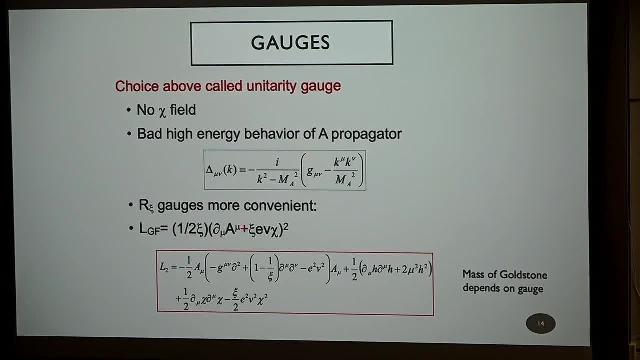 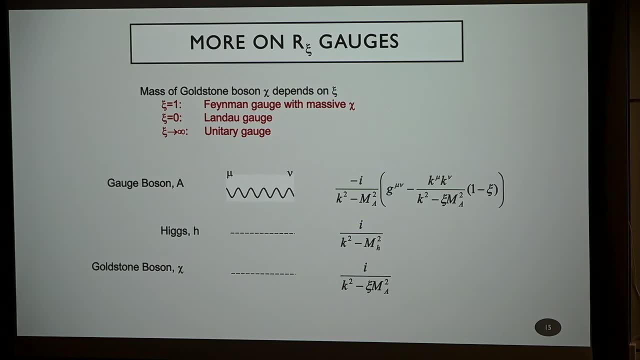 where the interactions of the two gauge fields here depend on the gauge shift. Okay, So the propagators of the gauge bosons, which now I'm talking about an abelian model, but in a minute I'm going to tell you. well, we can do it for SU2, cross, U1. 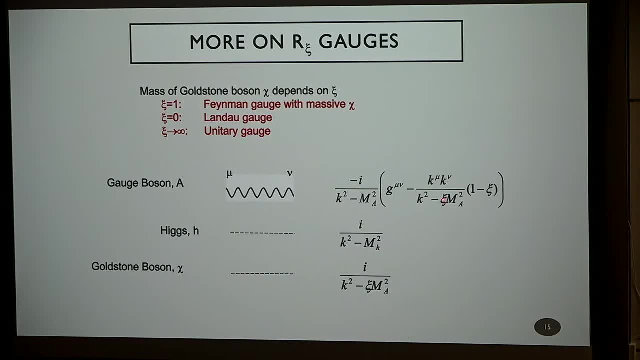 The propagators of this massive gauge field depend on this gauge transformation property. So most of us know and love Feynman gauge. Feynman gauge is 8 equals 1 and it's just G mu nu for the propagator. So in Feynman gauge 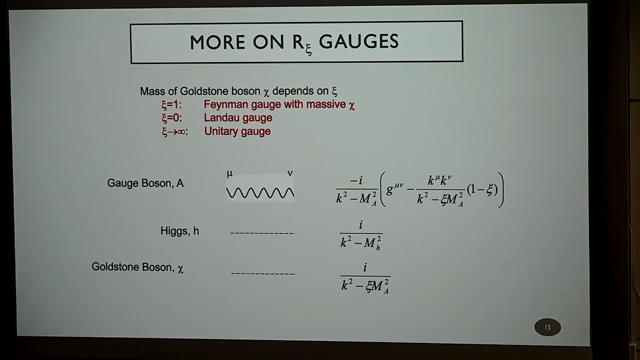 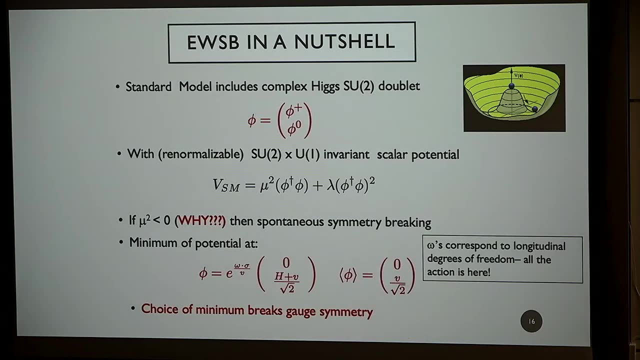 the goldstone bosons propagate, however. So if you're calculating something, you have to include the goldstone bosons, which can be a pain. Okay, So now let's talk about the real model Now. I'll do this in two slides. 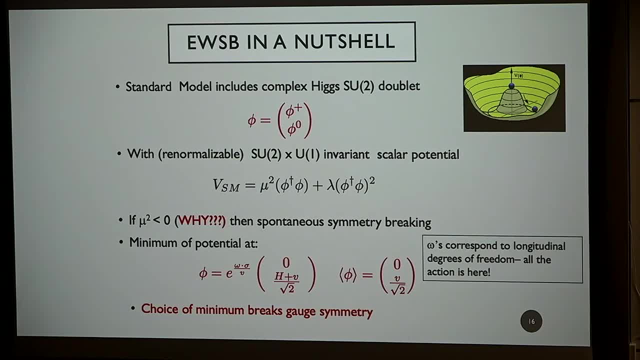 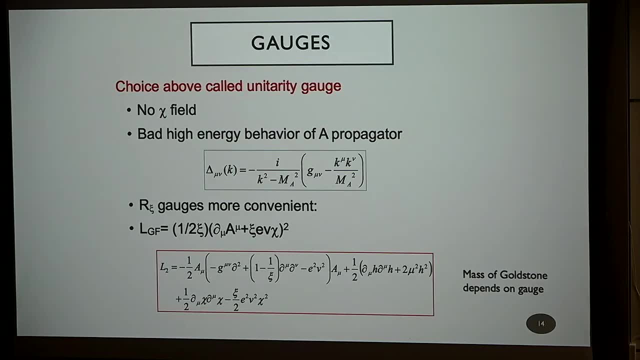 Okay, so in the standard, Yes, Yep. Chi is not a degree of freedom, because chi is just a number, It's something we put in by hand. It's not a field, It's just free. I can pick it as I like. 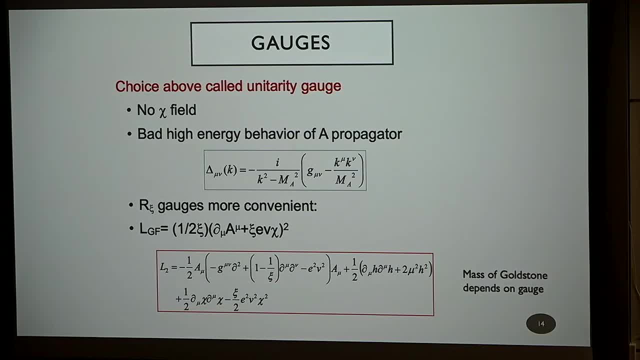 If I felt like it, I could pick it to be 2 thirds, Like you know, that wouldn't be convenient, But Oh, you mean this guy. Yeah, so the counting is different And in fact, when I do the counting, 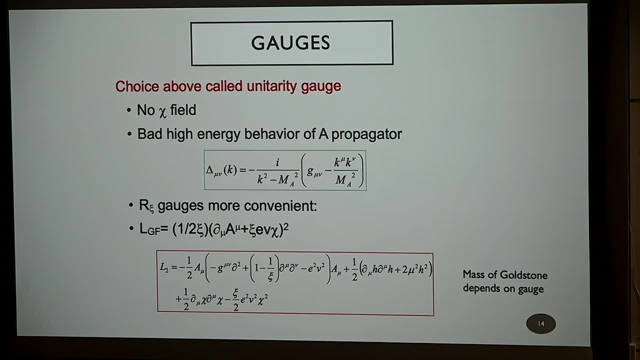 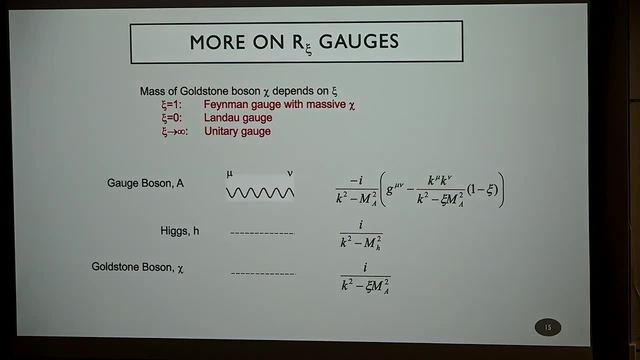 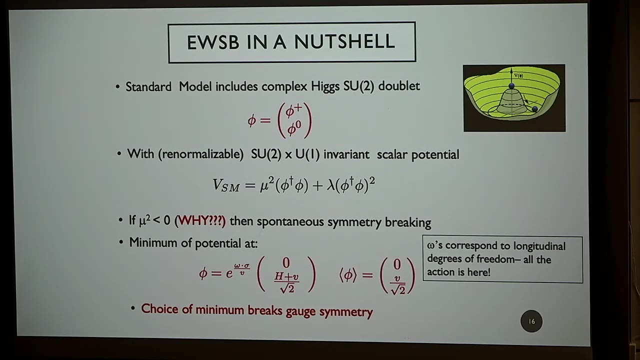 it's gauge dependent how you do the counting. Yeah, Right, Yes, I'll show you in a few minutes and you'll say that I'm sliming you because that's a very good point, Butyeah, So You looked at my slides ahead of time. 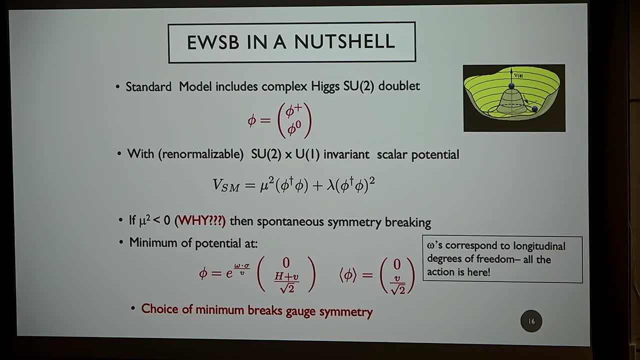 Well, you could have really gotten me on this one, because there is a point So electroweak symmetry breaking. So now let's look at the real standard model with the Higgs. I'm going to put in a complex SU doublet. 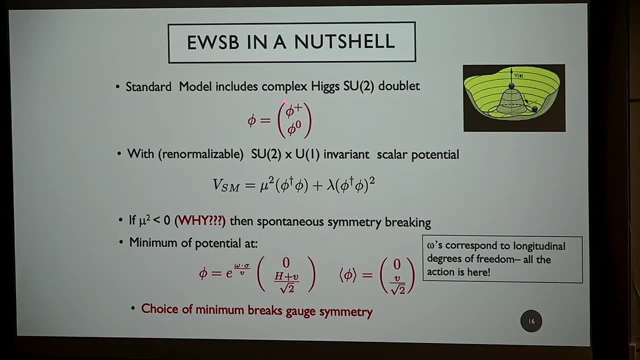 So a phi plus and a phi zero. It's complex. So there are 2 degrees of freedom upstairs and 2 degrees of freedom downstairs. So there are 4 degrees of freedom in my phi field. So then I can write down the most general renormalizable. 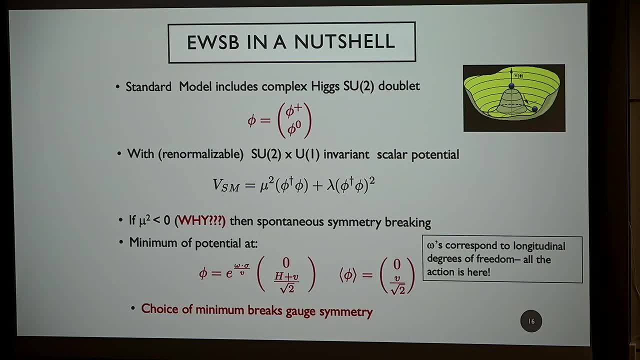 SU cross U invariant scalar potential. So here's my potential: Mu squared phi dagger phi, plus lambda phi dagger phi squared. And this is exactly the same thing as I wrote down for the Abelian Higgs model, other than the fact that the phi is now an SU doublet. 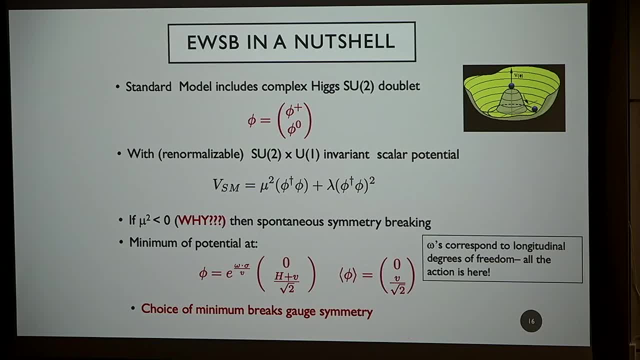 So this mu squared again will take it to be negative and I'll say, well, I don't know why, but if I take it to be negative, exactly the same thing happens as in the Abelian model, And the minimum of the potential is here. 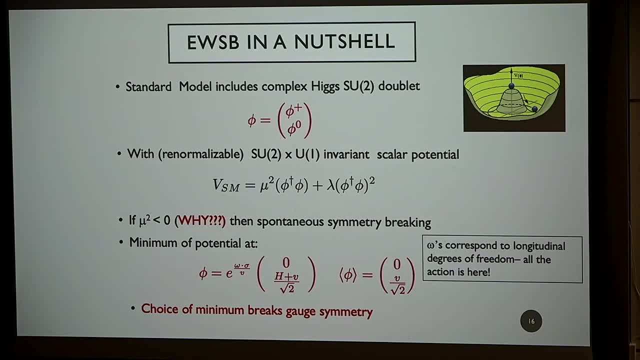 H plus V over square root of 2.. And now my goldstone bosons. I'll call them omega here. So there are 3 of them. It's omega, dot sigma, Sigma are the Pauli matrices And omega is the freedom, because phi has 4 degrees of freedom. 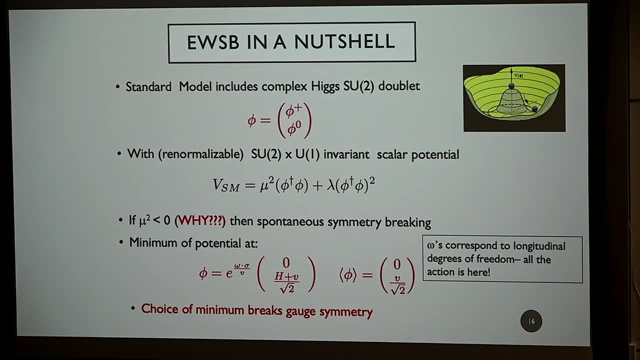 H has 1 degree of freedom And the omega has 3 degrees of freedom. here I've tried very, very hard- I've probably been unsuccessful- to call the standard model Higgs capital H. You'll probably find places in my notes where it's not capital H. 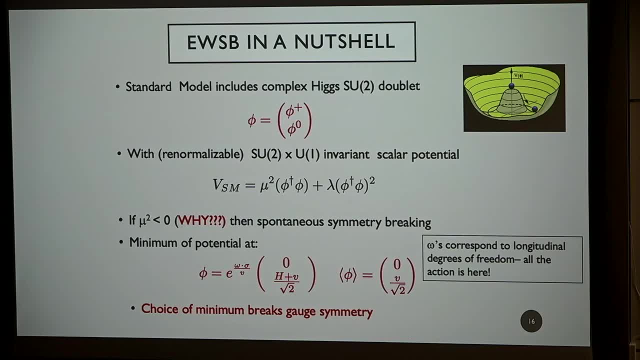 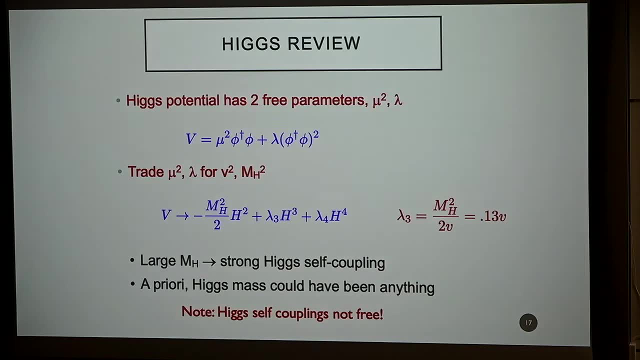 but I've really tried to make it always be capital H. Okay, So now we can do the same algebra as before, And I'm not going to do it, I'm just going to tell you the answer. I'm going to tell you that. 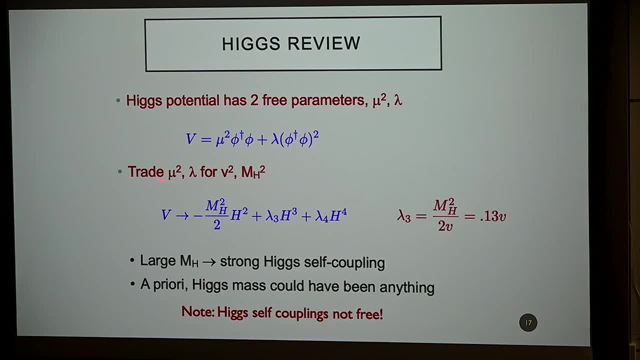 we have the potential. It's got 2 parameters, But now I can trade the mu squared and the lambda for V squared and the mass of the Higgs squared. Yes, You mentioned in your favorite models you had a scalar and another Higgs. 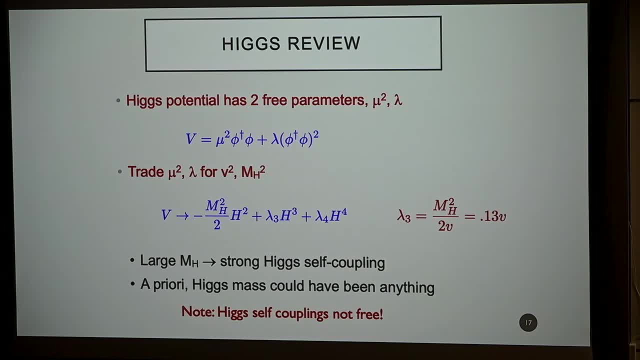 Does that when in models in which a second Higgs is added, does it always have to be a doublet? It can be an SU singlet, in which case it doesn't do a whole lot. It can be an SU triplet, in which case there are tons of limits on it. 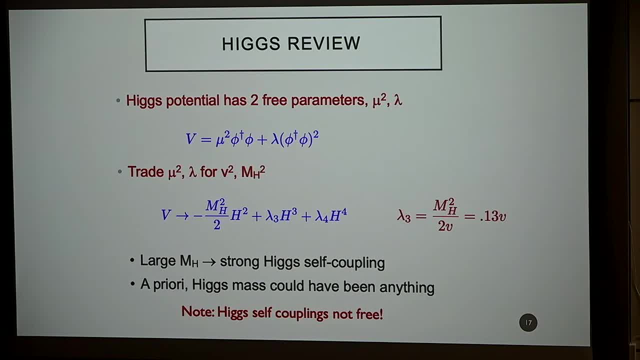 from consistency of the theory. It can be any representation of SU. I wrote a paper with SU quadruplets, which is not very interesting, by the way. But no, it doesn't have to be a doublet. The doublets are the easiest and maybe the most motivated. 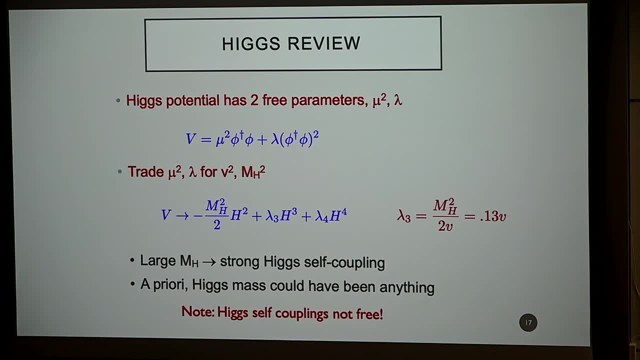 but it doesn't have to be. Take your favorite representation, write a model, have some fun, And actually that's one of the things you should get out of my lectures is that when you build a model with some new scalar, there are all these things you have to check. 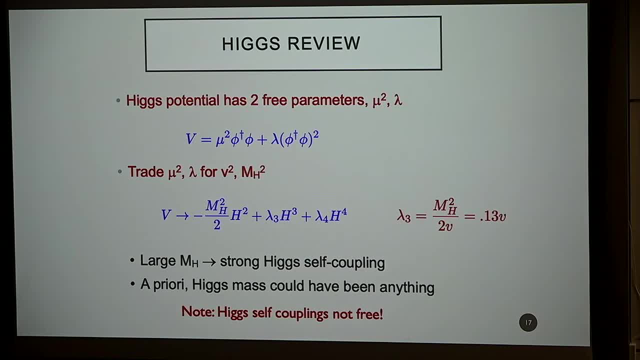 to make sure it's a good model. And you know it's formulaic. you gotta check this, this, this unitarity, blah, blah, blah. So hopefully by the end of my lectures you'll have your checklist for my model And most of the models you'll see. 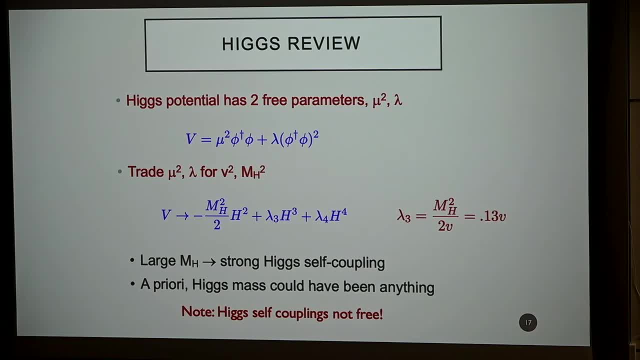 are stringently limited at this point. Okay, We solve for v squared in terms of mu squared and lambda. We multiply everything out during our algebra and we get the potential. It's got a Higgs field with a mass. It's got a Higgs cubic term. 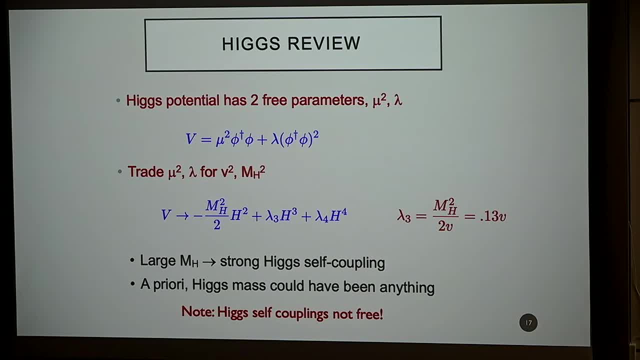 and a Higgs quartic term, And the really, really important thing to remember about the standard model is that these things are predicted. The trilinear couplings of the Higgs, which I call lambda three here, are predicted in terms of mh squared over 2v. 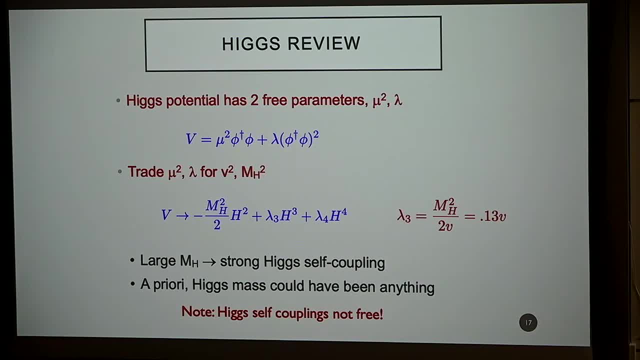 So you've probably heard a lot about Higgs mass talking about measuring the trilinear coupling. Well, in some sense that's just crazy, because if it's not exactly mh squared over 2v, bingo aha. right now you know it's not the standard model. 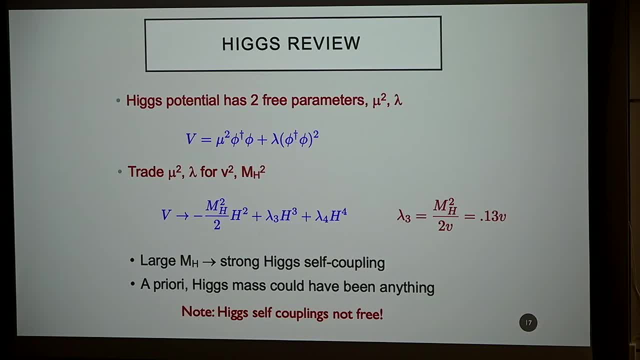 These are absolute predictions and there are no free parameters, And that's why it's such an amazing model is because you are not free to adjust anything. You've got the Higgs mass and you've got v And that is it, guys. 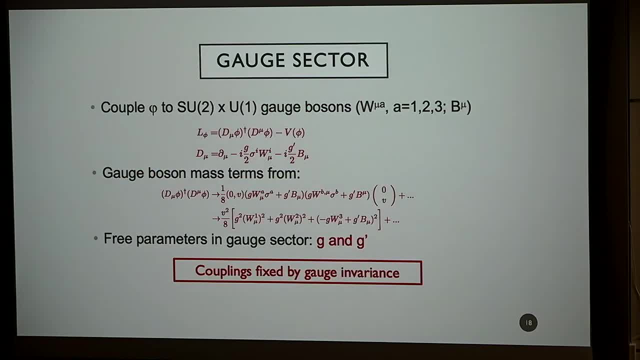 So it's a very, very simple model. Okay, Yeah, questions. Okay. so a little bit of algebra here. I'm not going to work it out, because it's simple. You can couple the gauge bosons to the SU doublet. 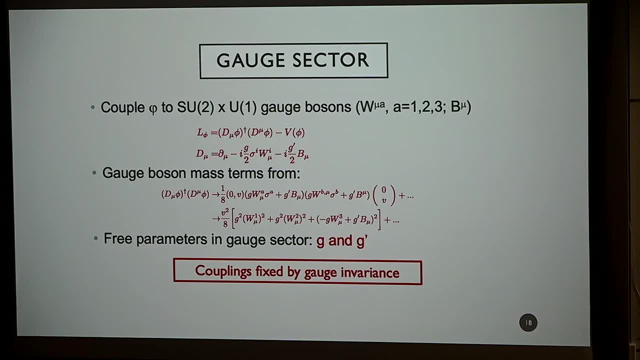 So now I have a covariant derivative which I've written down here. It's exactly like the one I wrote down for the coupling of the photon d, mu minus iea. So here g is the SU coupling, g prime is the u1 coupling. 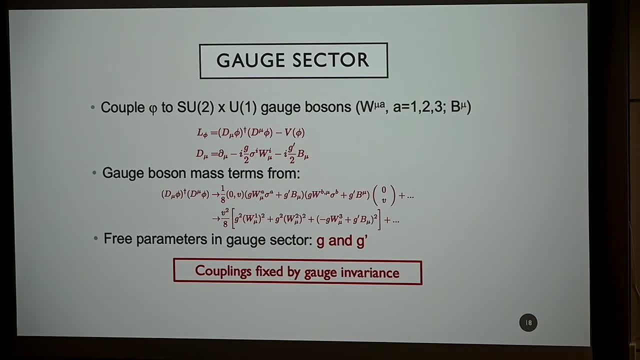 b is the u1 gauge boson and unfortunately w mu a is the SU gauge boson And this is historical, the way people do this stuff. w mu a. these are SU gauge bosons, So they are not the physical w bosons. 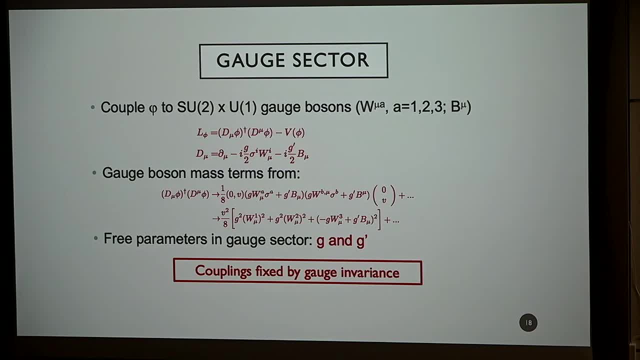 Sometimes you might use a different script or something for them, but it's confusing, I think, because these are the SU gauge, bosons that couple. So here we go. So we write down: d mu phi, d mu phi with the covariant derivative. 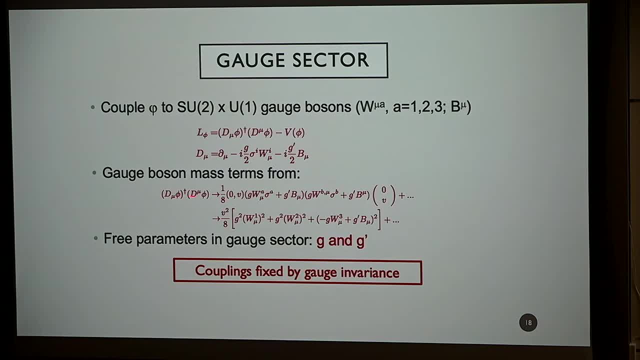 and you can get the mass terms. So let's see here. So the phi has a one over the square root of two which goes to one half, and then you've got these guys squared. so that's the eighth from two d mus. 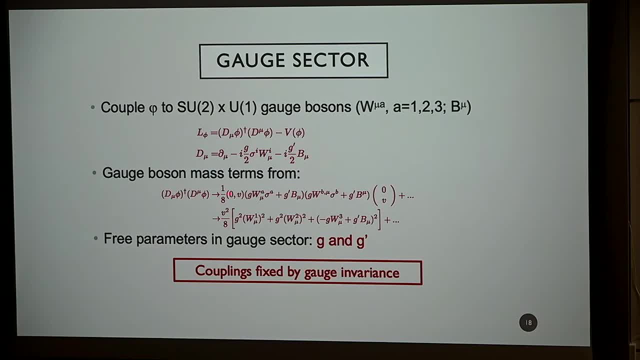 and from two, one over square roots of two. And here's the v. I just wrote down the v in the phi field. Here's the v, And here are the two covariant derivatives. Okay, so you multiply this thing out and you've got. 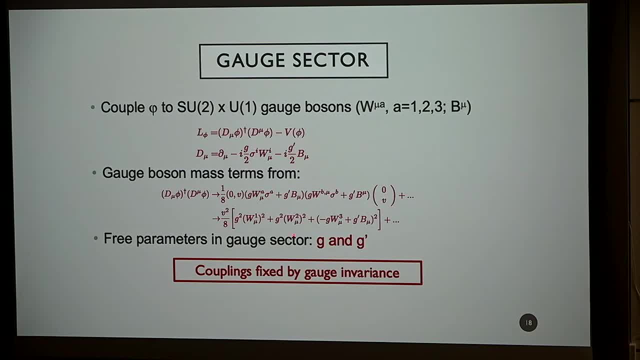 g squared, w1 squared, g squared- w2 squared, and then another combination here. So this combination here is going to get a mass and be the physical mass of w boson, And this combination here is going to get a mass proportional to v squared. 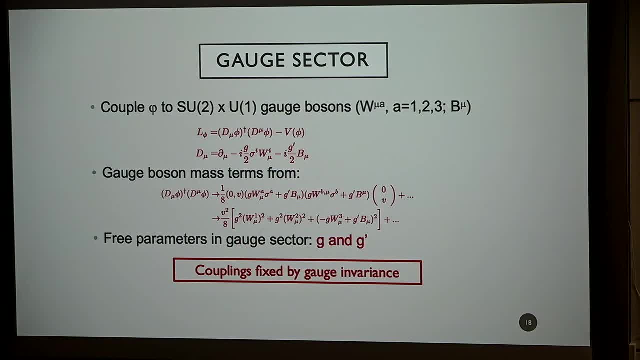 and be the physical z boson. And again, let me state the really important thing: There are no free parameters here. There are no free parameters, These couplings, they're absolutely fixed by gauge invariance. Okay, so here's just some algebra. 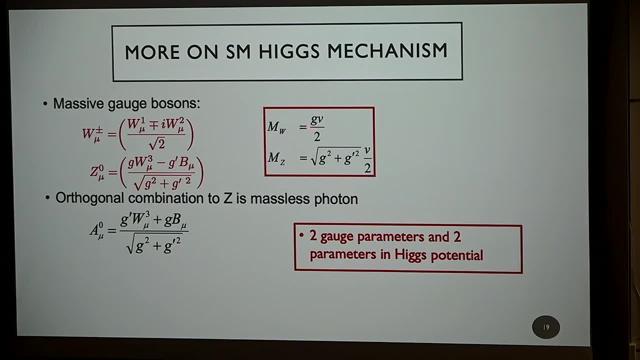 You get the w mass and the z mass. so the w mass is the SU coupling times v over 2.. The z mass is the SU coupling v over 2.. So the masses are proportional to the vev and to the gauge couplings. 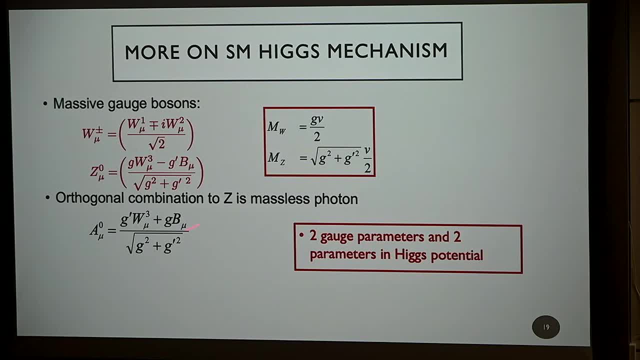 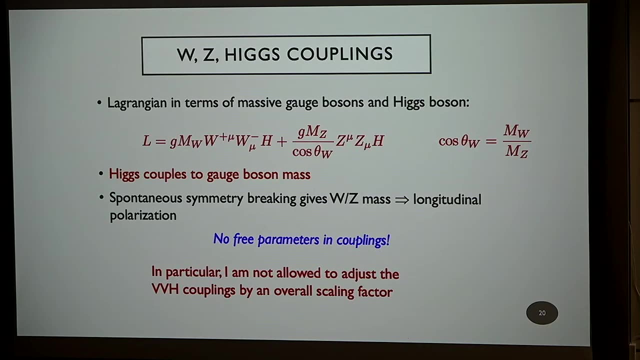 And so the orthogonal coupling to the z is the photon, and it's massless. So here we go. So we started out with two parameters and the Higgs potential, and now we've got two gauge parameters and that's it. This is the standard model. 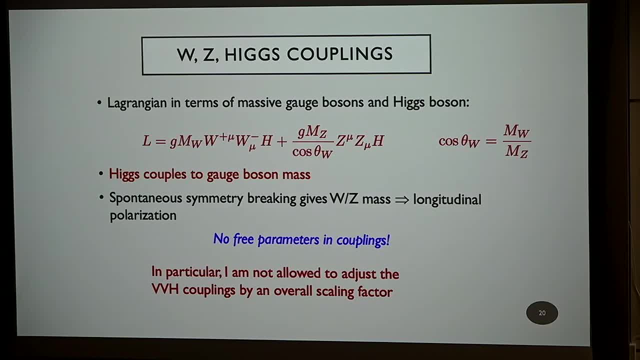 Here are the couplings to gauge bosons written one way. So the physical w is coupled to the Higgs, proportional to the SU coupling and the mass. So here's the mass, And the z is coupled proportional to the gauge coupling the mass. 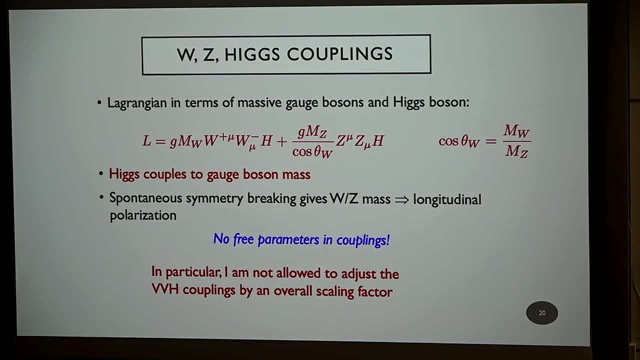 And cos theta w is just the ratio of the masses here. So it's nothing deep and profound, It's just the ratio of the masses. So the spontaneous symmetry breaking gives the w and z a mass, and again it gives them all the physics. 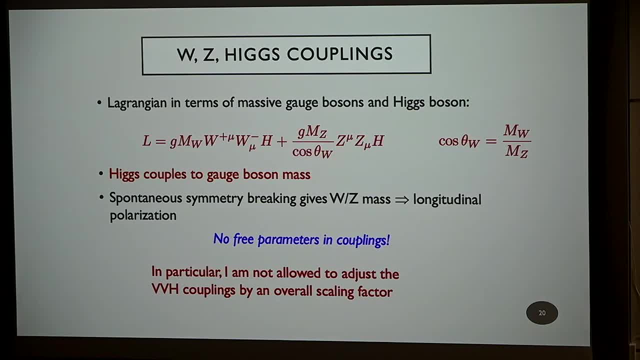 And again, there's no free parameter in the couplings. So when you look at the limits on the couplings of the Higgs to the w and the couplings of the Higgs to the z, well, if it's not exactly one, it's new physics. 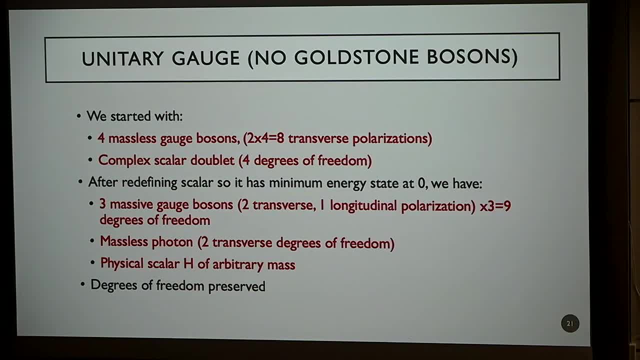 Okay, Okay. so here's the counting for you. I'm going back to unitary gauge, which is the only gauge that you can really do this in, because unitary gauge has no goldstone bosons. We have four massless gauge bosons: the SU2 and the U1. 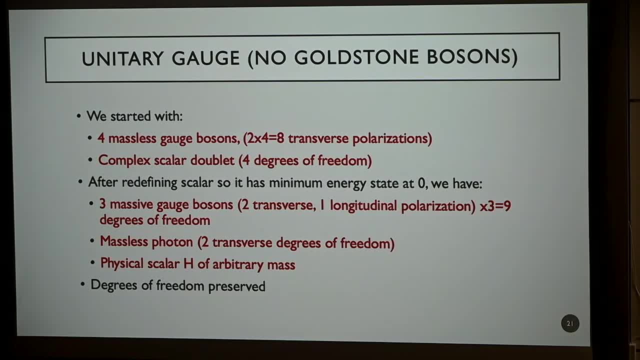 gauge bosons, So they only had transverse polarizations because they were massless. We had a complex scalar doublet which has four degrees of freedom aka 12 degrees of freedom. So after the spontaneous symmetry breaking, we have three massive gauge bosons. 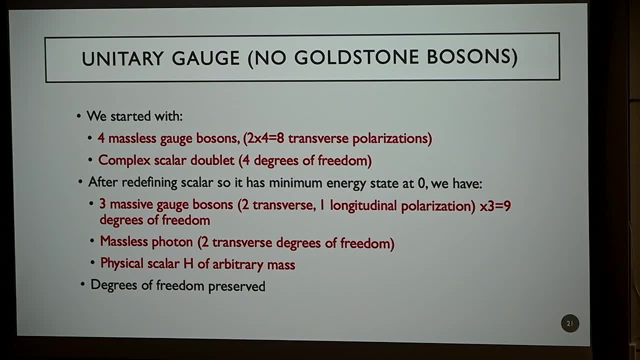 the w and z, and they each have three polarizations, two transverse, one longitudinal, So they're nine degrees of freedom. We have a massless photon, two degrees of freedom and a physical scalar. So in unitary gauge you can do the simplistic counting. 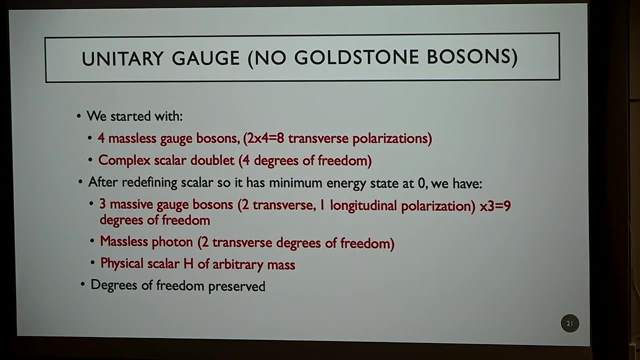 where the degrees of freedom are preserved. This kind of simplistic counting only works in unitary gauge, But you can see. what's happened is you've changed degrees of freedom from your scalar field to the transverse or to the longitudinal polarizations of the gauge bosons. 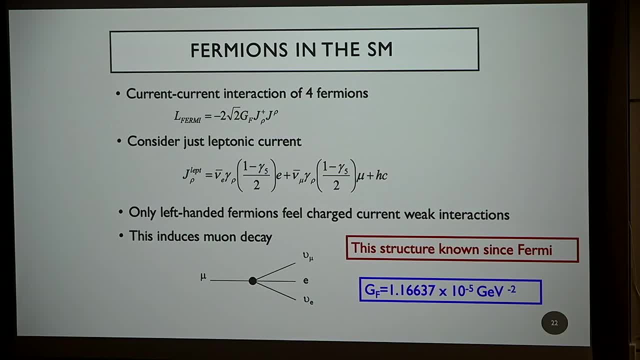 Okay, So far our model has no fermions, so it's not very interesting. In Fermi we had a structure of how four fermions interacted, So we had that the fermions interacted through couplings or leptonic currents. here we'll call them. 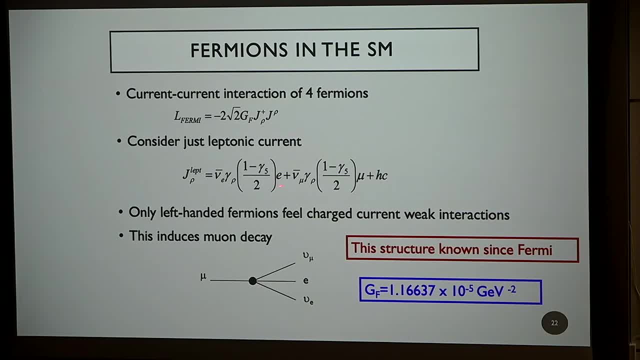 And these currents were just the couplings of the electron to the neutrino, muon to the neutrino, and by explicit measurement. way back in the day we knew that the fermions or the leptons only coupled to the weak interactions by left-handed couplings. 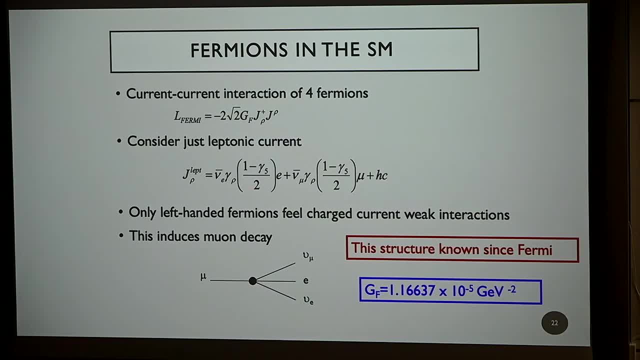 One minus gamma, five over two. So only the left-handed fermions felt the charge: weak interactions. So you have muon decay. you measure the electron coming out. so the only things you can measure are the energy spectrum of the electron at different angles. So by measuring this we induced. 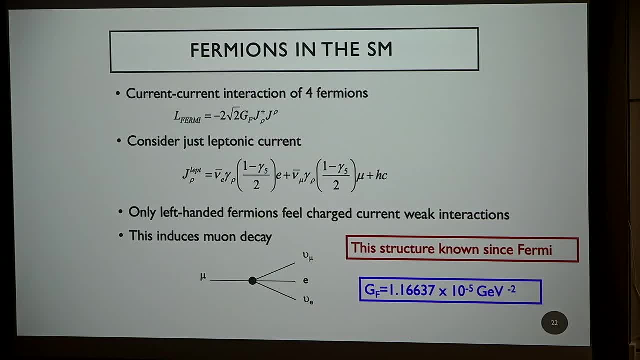 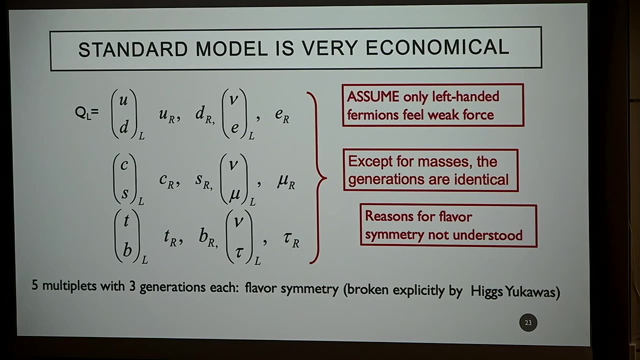 that it was left-handed one minus gamma five, And this has been known for a long time. So when it came time to put fermions into the standard model, we just made an assumption. This is probably pretty obvious, but could you explain again how muon decay tells us? 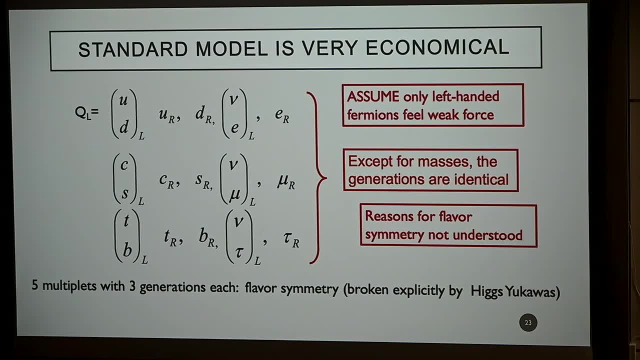 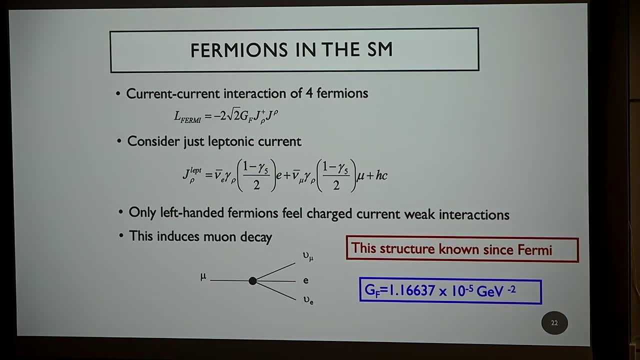 that you can only couple to left-handed particles. That's not so obvious. That's a really good question. In fact there are tons of theory papers. So you would make an onset. you would say: maybe it couples A times one minus gamma five plus strength, B times one plus gamma five. 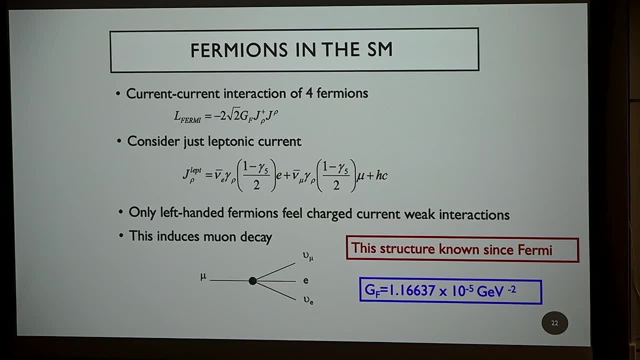 plus strength C times a scalar coupling like that. And then you do tons of measurements And you would see that this is what came out. So it's an experimentally inferred thing. So no, it's not obvious. Yeah, yeah, they used to measure these things. 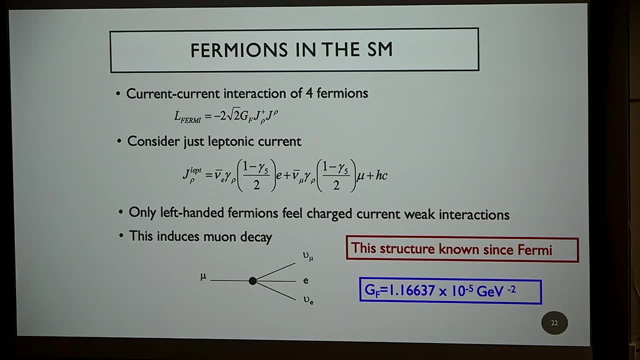 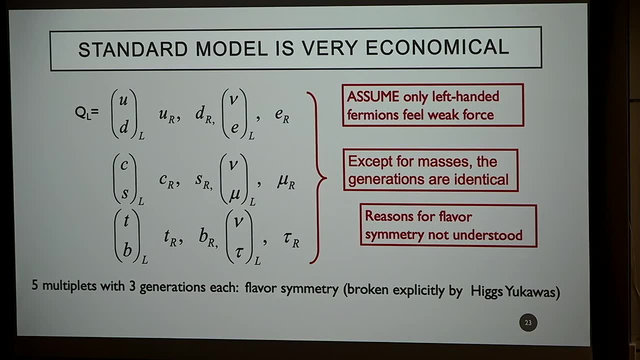 there are a whole lot of old time experiments measuring these. So then we say we're going to construct our model of weak interactions exactly the same way. So we're going to put a weak interaction- and then it talks to the weak interactions- into a left-handed doublet. 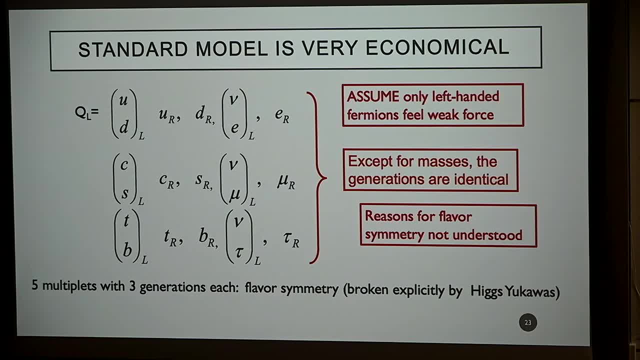 So here are the quarks up down left and the neutrino and electron left. So here they are. So we'll by onset say that they talk to the weak interactions, So they will be SU doublets, and then we'll assume that the other guys 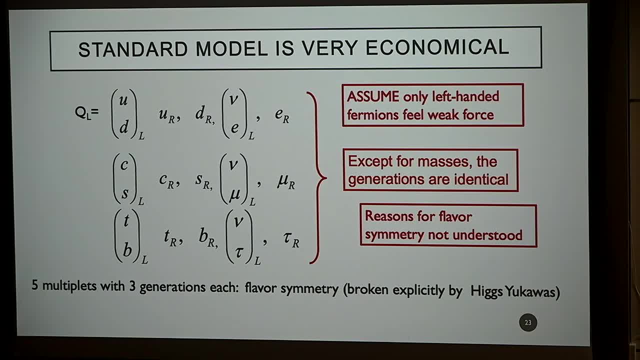 are SU singlets, So this is put in by hand. And except for the masses, all the generations are identical. So if we didn't have any masses or interactions of the fermions, we would have a U3 to the fifth symmetry, So we had 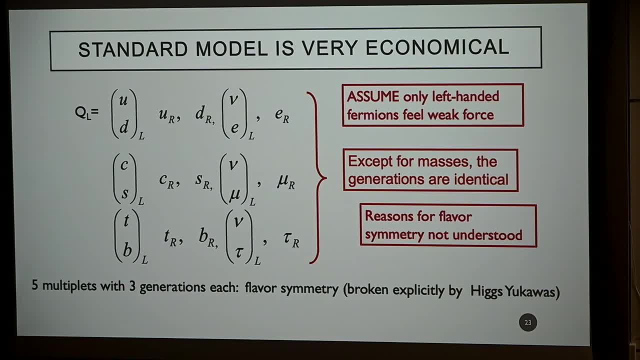 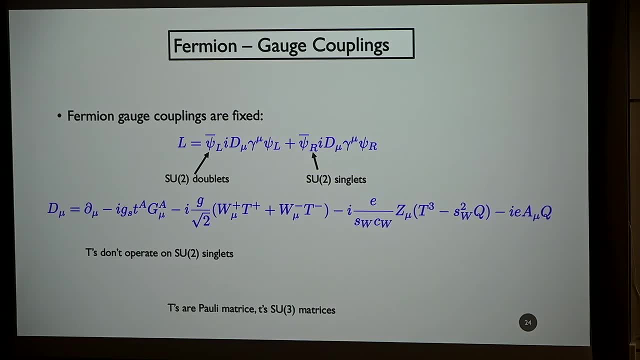 five multiplets. Okay, we put them in by hand. But now something kind of interesting happens. So the fermion couplings to the gauge bosons are again fixed. There are no free parameters. Couple with the gauge covariant derivative d mu here. 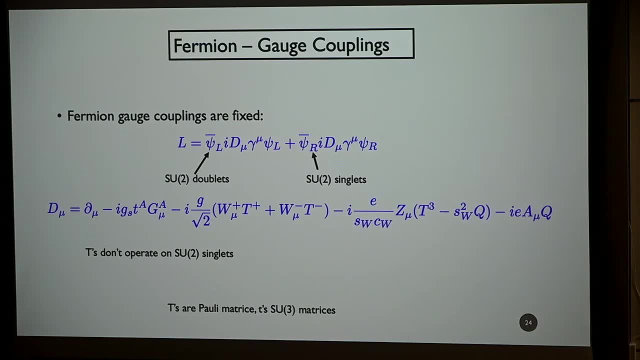 And the right-handed singlets couple with the gauge covariant derivative d mu. So I just wrote down what it is here. So this is color which only acts on the quarks. These are the gauge interactions. So T plus, T minus are combinations of the polymatrices. 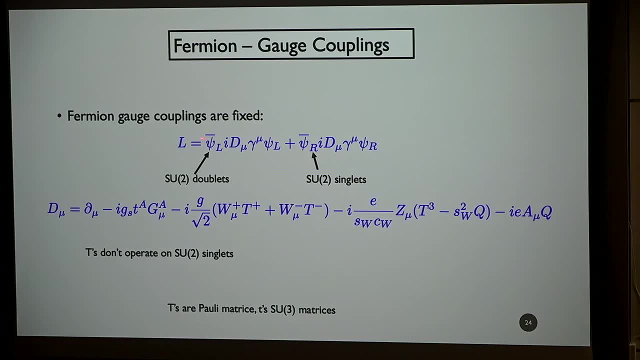 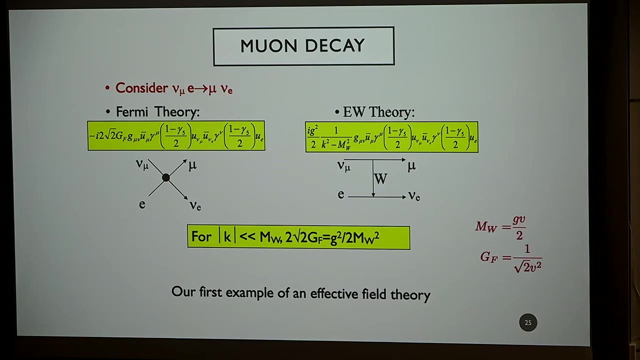 T3 is a polymatrix, So these guys, the Ts, only act on the left-handed guys. These guys act on the right-handed guys. So it's fixed. Oops, So now we can go back to our theory of muon decay and we can learn one more thing. 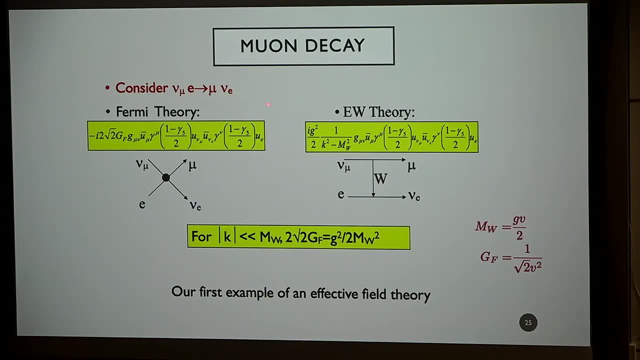 We can learn that if I'm looking at, I put here nu e goes to mu nu, just to make it easier. It's the same interaction. So in the Fermi theory the interactions of the muon and the electron and the neutrinos would have the left-handed structure. 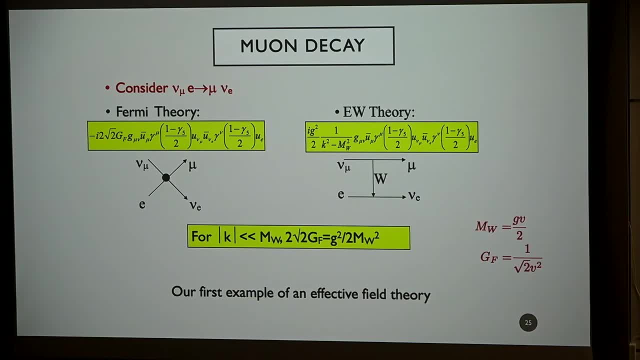 of G Fermi here And that defines the strength of G Fermi. That's just put in. But now I can calculate this in my electroweak theory, because now I've postulated that my leptons interact via the weak interactions here. 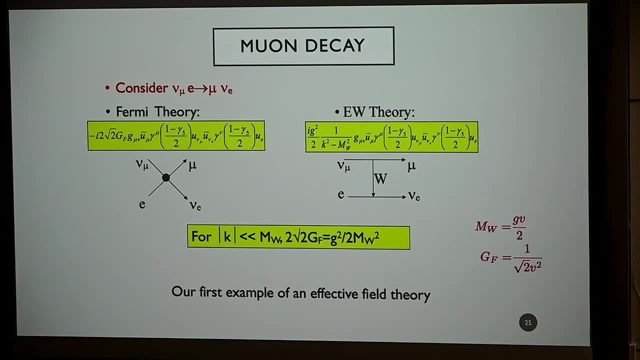 So we've got the muon with the neutrinos, So it's G over square root of two and the one minus gamma five at the vertex. And then there's a propagator here and the momentum K is much, much less than Mw. 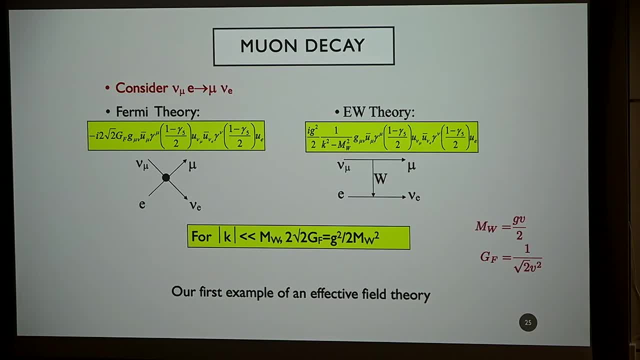 So these two things are supposed to give us the same answer. So if K is very small, we've got this side two square root of two G. Fermi equals this side G squared over two Mw squared. So by matching them up we see that this parameter V. 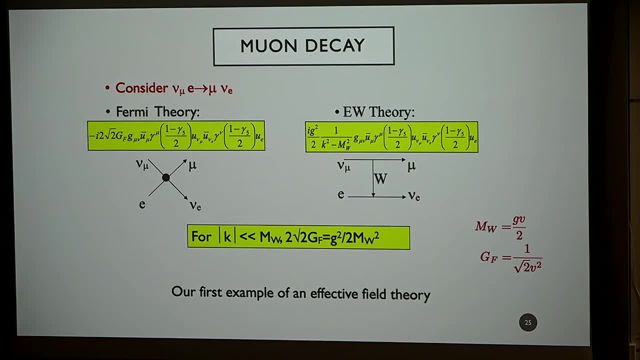 the vev of the scalar field is not a free parameter. It's fixed by muon decay. In particular one over square root is G Fermi. So V squared is 246 GeV. So here's our first example of an effective theory. 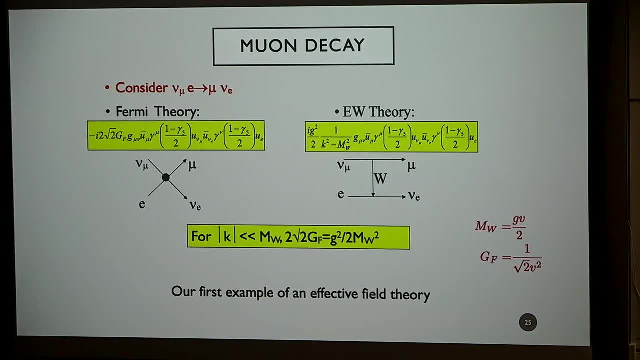 So the effective theory is the Fermi theory, which reproduces the exact high energy theory of the SU2 cross U1 theory. So by making this matching, what we've done is we've reduced our number of parameters even further. So now we've. 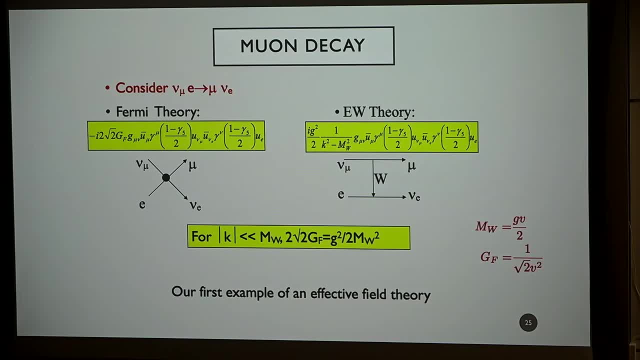 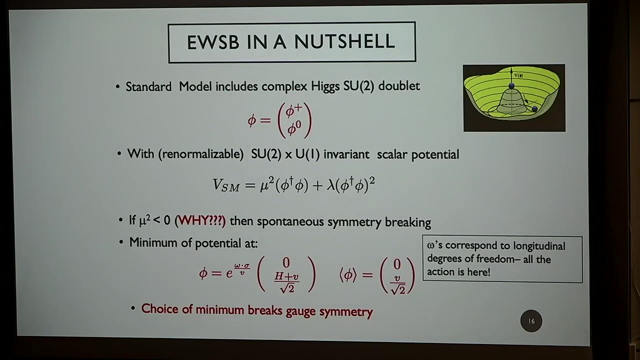 Yeah, Ah, but this doesn't tell us what the Higgs mass is. It just tells us what V is, And that's a really good question. Let me go back. I think I have the formula here. That's why I like slides. 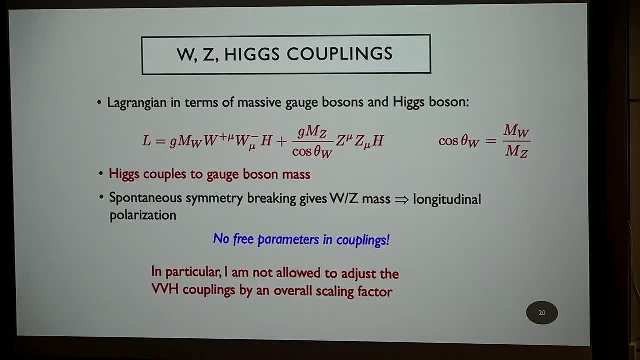 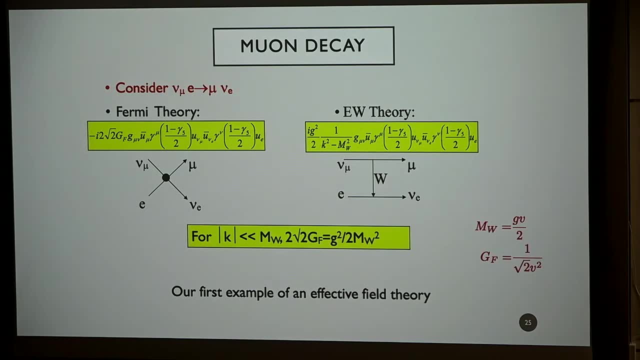 even though I know they're not good. But no, I didn't write down that formula. Okay, The Higgs mass is still a free parameter. So by the counting in the scalar potential, I had mu squared to phi fourth. So then I'm going to change. 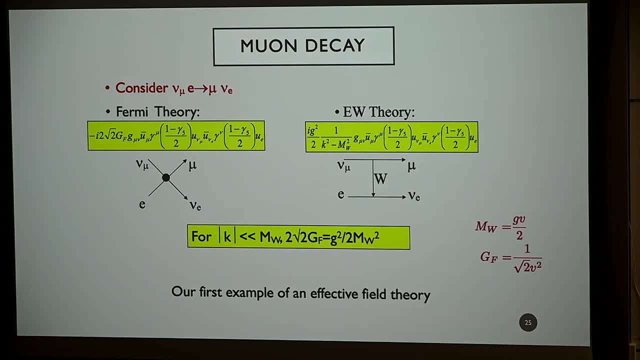 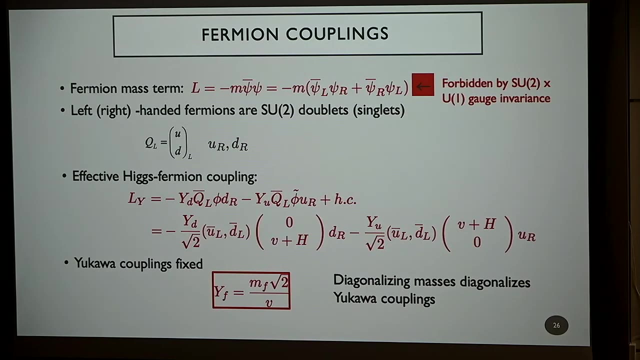 that mu squared and the lambda for G Fermi and M Higgs. So M Higgs is still a free parameter in my theory, But it's only got one free parameter now. Okay, Yeah, Actually a question about that. So isn't the BEV technically? 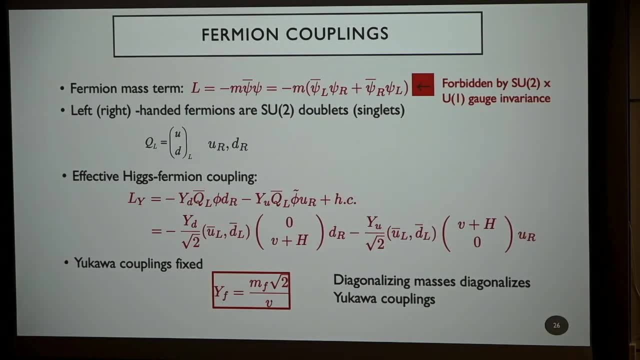 also a free parameter, just very tightly constrained by the Higgs mass. It's not an approximation, It's the matching of the weak interactions to our gauge theory. So it really is fixed because our gauge theory has to reproduce the weak interactions. But wouldn't it only work. 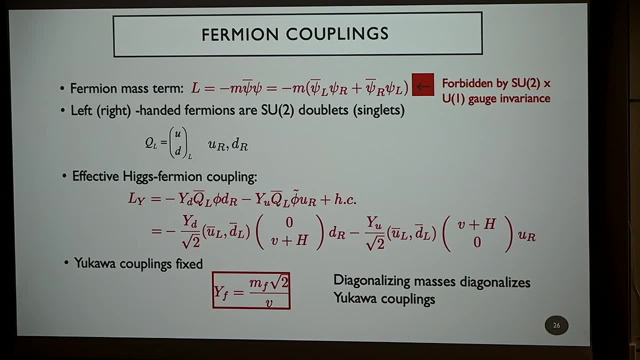 for K equals zero. Well, the mass of the muon is really much, much less than 80 GeV, So it's pretty exact, Yeah. So let's see what time. This is one more miracle of the standard model which you have to appreciate. 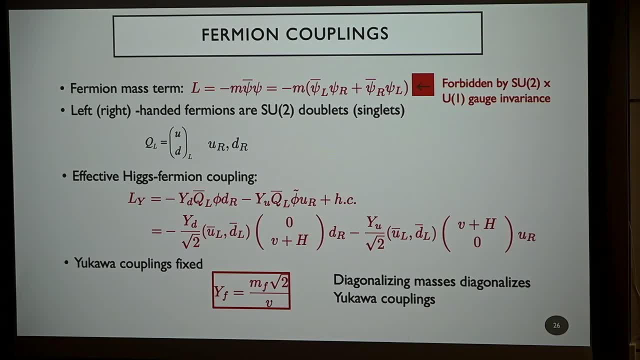 that this stuff is really miraculous the way it comes out. So we want the fermions to have a mass. We know the B quark is a mass. You might think maybe the up quark was massless, But you know the B is pretty heavy. 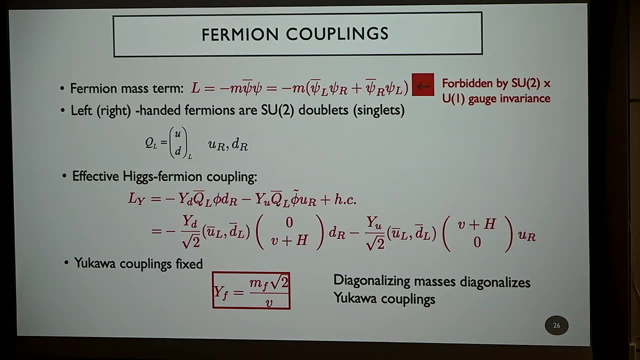 The top is pretty heavy, So our theory has to accommodate fermion masses. So what if I try to just add a mass term? Well, you can't do it the way we've constructed the theory, because the left-handed particles are SU2 doublets. 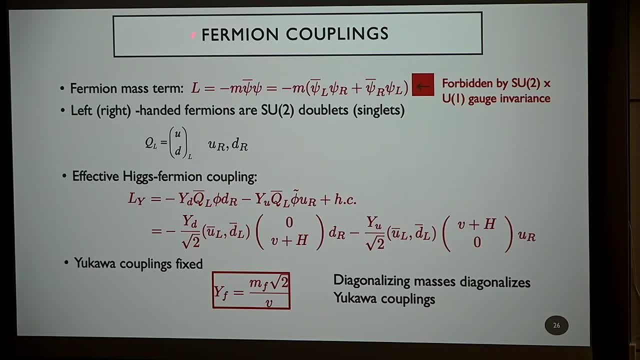 and the right-handed particles are SU2 singlets. So a mass term would couple left-handed particles with right-handed particles. So I am not allowed to add a mass term again by this requirement of gauge invariance. So gauge invariance. 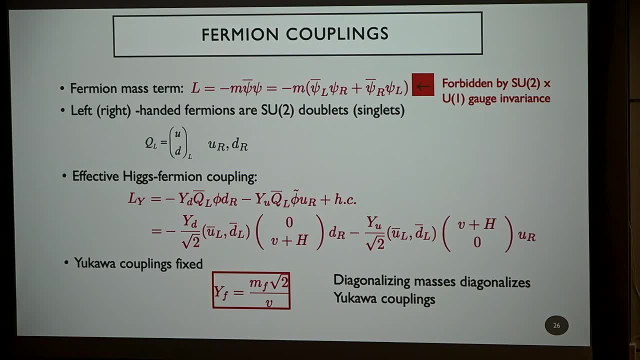 SU2 cross. U1 gauge invariance and left-handed fermions are SU2 doublets. So I can construct a gauge invariant object out of these two SU2 quantities. So I can construct an interaction side-bar left. So this is my up-down doublet. 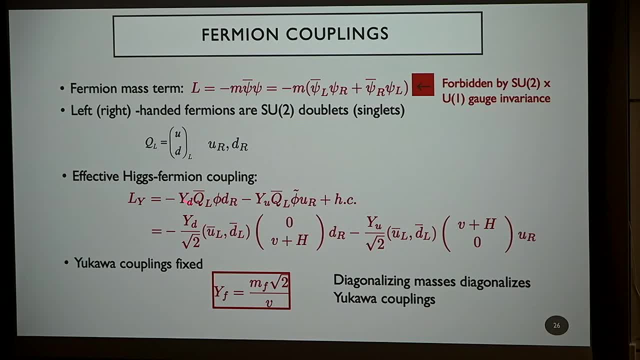 SU2 doublet. Phi is an SU2 doublet, So the indices work out here, And D is a right-handed singlet, So this guy can give me a mass term for my fermions. So what it does is it takes a component of the left-handed guy here. 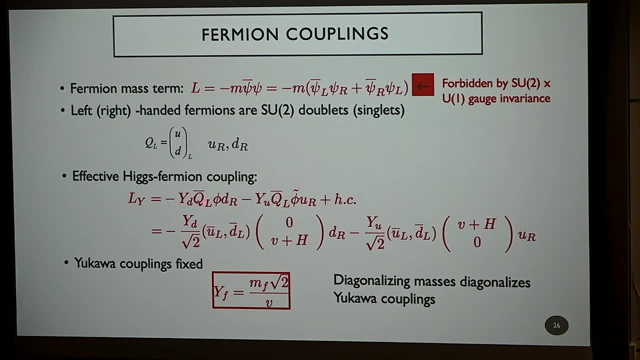 talks to the down component of the phi, which has a V in it and the right-handed down quark. So you have, here is V plus H downstairs from the phi and here is the SU2 doublet and here is the right-handed guy. 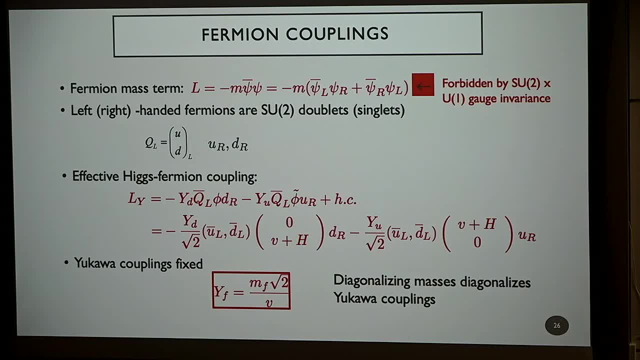 So it gives me a term which is D-bar V, D, So it gives me a mass term. So that is good and that is fine. The phi-tilde: there is I sigma 2 times phi, which makes it so that we have V plus H upstairs. 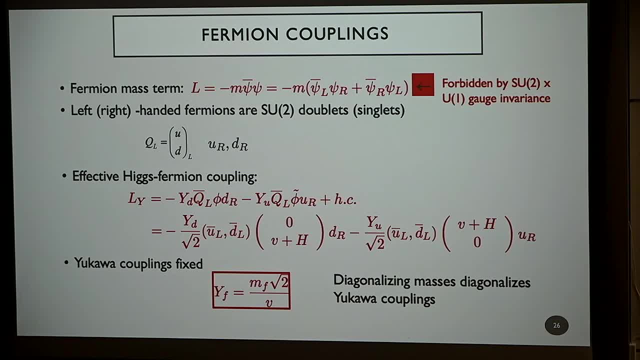 so we can give the top quark mass. So now, this is great, We can give everything a mass. And so this Yukawa coupling in front here is proportional to the mass. So the Higgs couplings to the fermions are proportional to the mass. 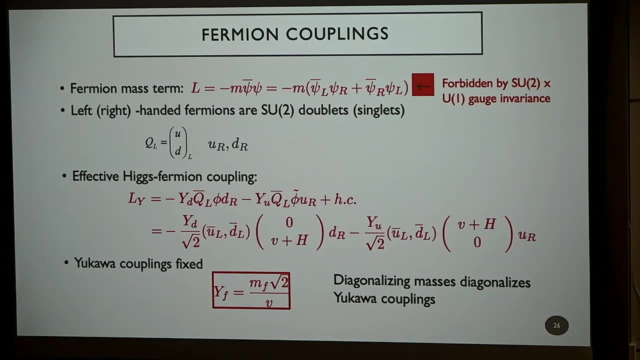 So now I've just done this simple example with one fermion, but if I wanted to, Yeah, So up there across U1, that's pretty straightforward. But once you've broken SU2, what here is specifically fixing the masses to the Yukawa couplings. 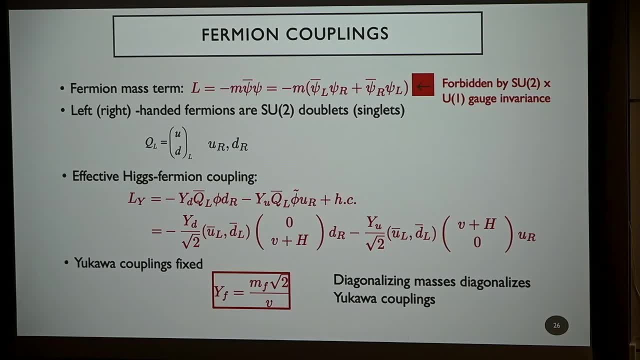 I mean, why can't we just add in extra terms and have those be incredibly tiny or have massless up quarks? Well, we need a gauge symmetry, So we're going to start with our gauge symmetry, So everything is going to start. 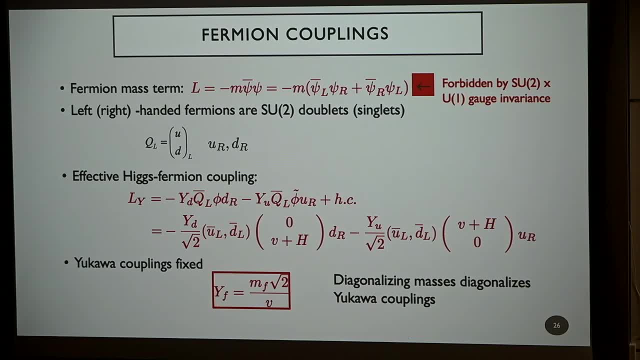 in a broken phase, So we're not going to add in anything else. in a broken phase We're going to say: I'm starting with my gauge symmetry and that's it. That's my model. And in that context, where that's my model, 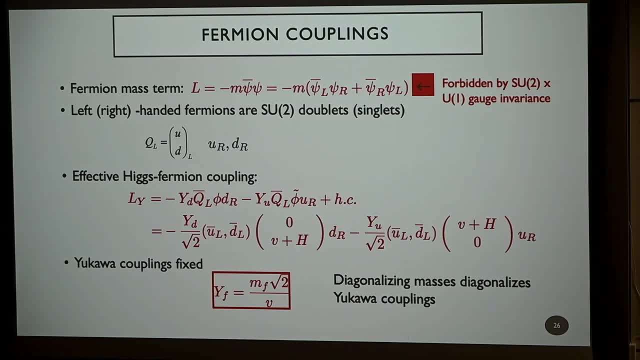 and that's it. I can't add anything else. Well, after this is broken, what's stopping you from just changing the In a U1?? After it's broken? I guess it's similar charges, But you, You want to just add it. 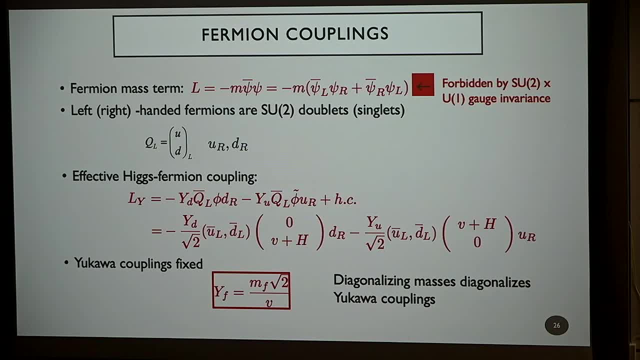 in quantum electrodynamics. Yeah Right, that's what I'm. We're only doing: a spontaneously broken theory. That's our theory. That's our theory. It's a spontaneously broken gauge theory. Yeah Yeah, it's bad if you do that. 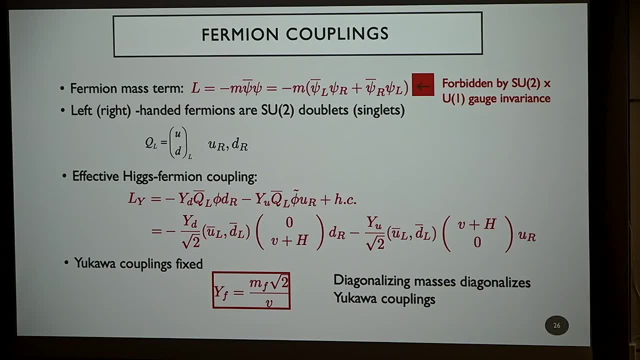 The specific part that I'm asking about is like: why are the masses fixed to the Yukavas? Because I mean, I know that massless up quarks have some appeal in where they can. That's another discussion. Let's save that for discussion. 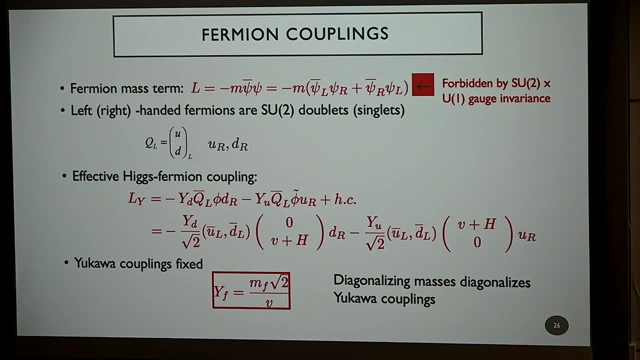 Yeah Well, I mean, there's no problem in this construction of having a massless up quark right. It wouldn't couple to the Higgs. So Suppose I said that there were some generation indices here, I had generations one, two, three say: 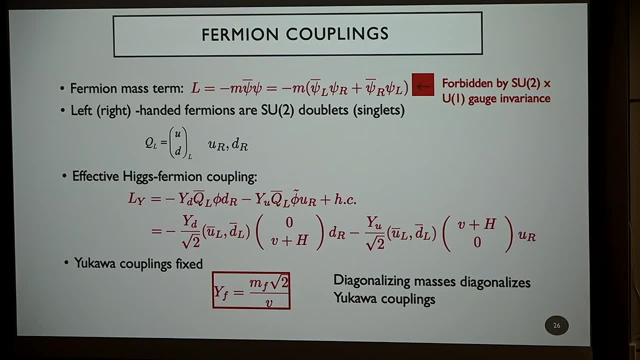 And then I had to diagonalize my mass matrix. See, I didn't get that. So when I diagonalize the mass matrix, I'm also diagonalizing the Higgs couplings. So there are no off-diagonal couplings to the Higgs. 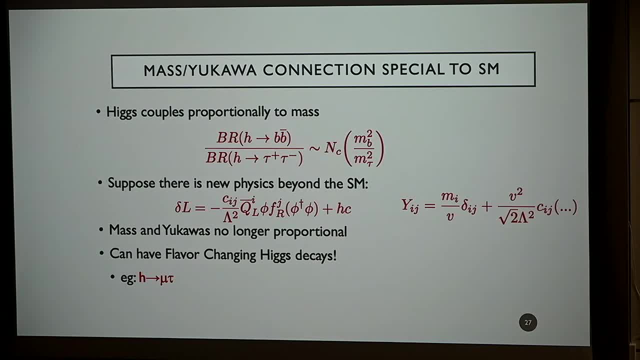 So this, This mass-Yukawa connection, is very special to the standard model. So the Higgs always couples proportionally to mass. So, for example, if I measure the rate that the Higgs goes to Bs normalized to the rate that the Higgs 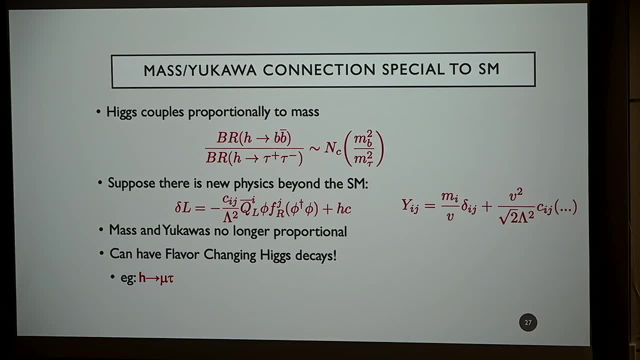 goes to Taus, well, there's a factor of three, because the B has color and it's just the ratio of masses, And this kind of relationship has been verified experimentally. So suppose, Suppose the standard model weren't everything, Suppose there was some physics out there. 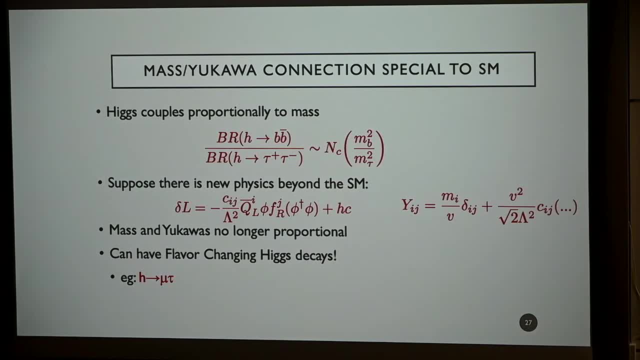 that I didn't have, So suppose I'm going to add a term to my Lagrangian, which has the doublets Q left. here's the Higgs, the right-handed guys, where these are generation indices i, j, 1,, 2, 3.. 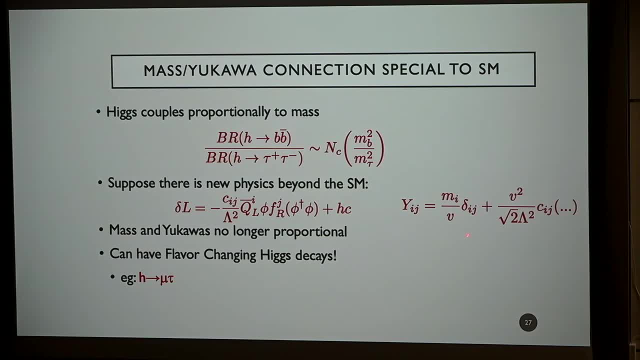 And it's got some matrix c, i, j, So then the Yukawas would be the mass terms as before, but then there'd be this extra piece from this term I added, And in general I can't diagonalize these things simultaneously- 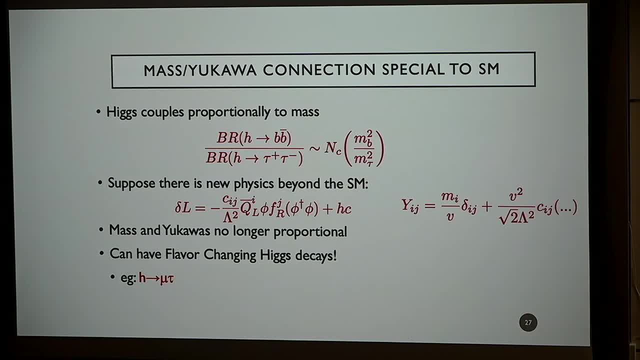 And so the mass and the Yukawas are no longer proportional. and then you get things like Higgs goes to Mu Tau. And this happens if I just blindly construct, for example, a two Higgs doublet model and I don't pay attention to the fact. 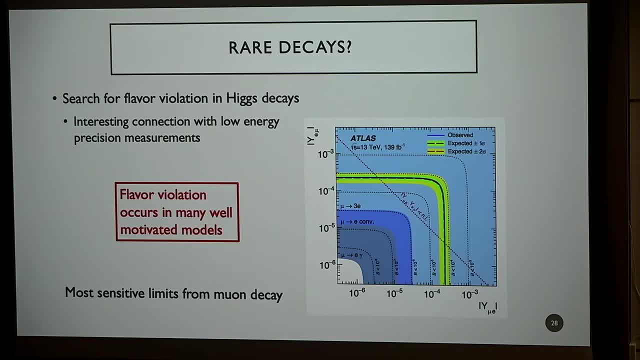 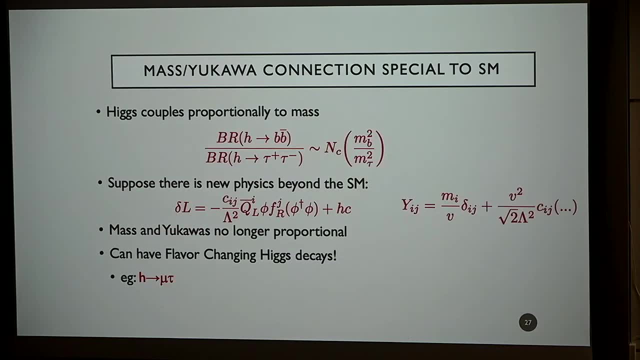 that I don't want interactions like this. So What do you mean? What do you mean by? Well, you could construct c i j in such a way that it could be simultaneously diagonalized, Sure, But in general you can get flavor-changing. 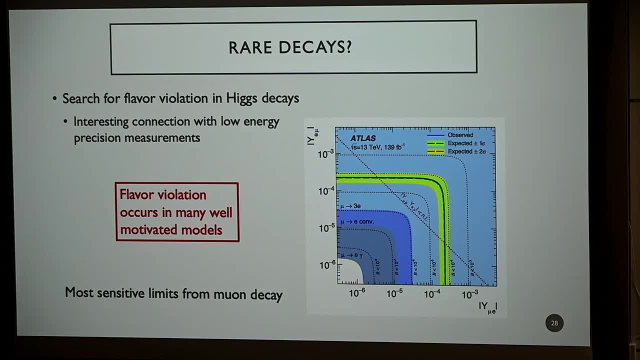 neutral currents unless you pay attention? Yeah, Are flavor-changing completely ruled out, or is there some little bit of room? Well, I'm glad you asked that, because here's the plot: There are a lot of flavor-violating Higgs, decays. 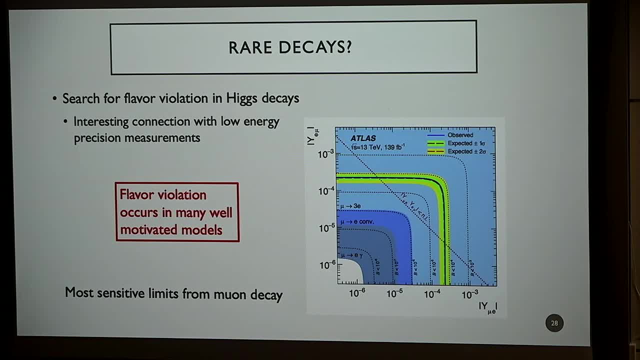 They look for things like Higgs goes to Mu E or Higgs goes to Mu Tau. I mean, there are a lot of plots that I could show you from the LHC. But yeah, people really want to look for this. And what's interesting about this? 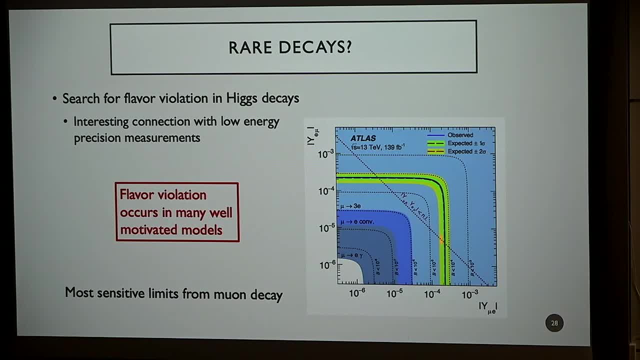 is the limit from the LHC? is this dashed line here? So these are off-diagonal Yukawa couplings And what you learn from this is that if you want to look for these flavor-violating Higgs decays, you can look for things like Mu to 3e. 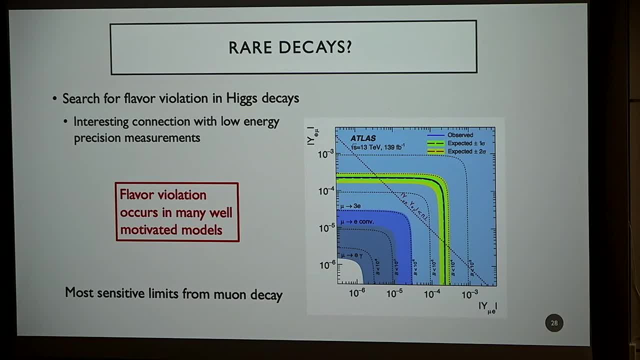 or here's Mu to E gamma down here. So precision experiments which are honed in for looking for these specific things are a better place to look for these guys And of course they're not completely ruled out. They can certainly exist at very small levels. 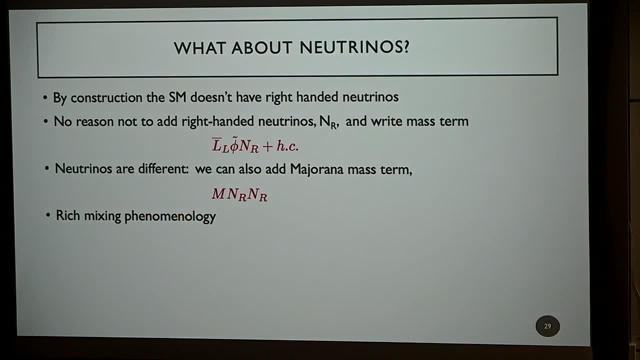 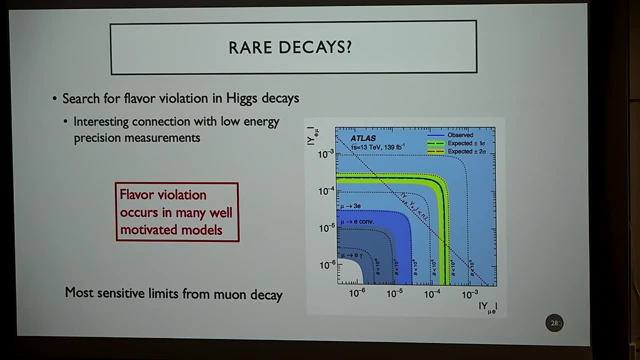 Okay, Yeah, Oh, that's a theory bound And that's the Yasi-Nir bound. It's a theory bound saying that you don't expect these couplings to be too big. They kind of make a fudge factor that the couplings are sort of proportional. 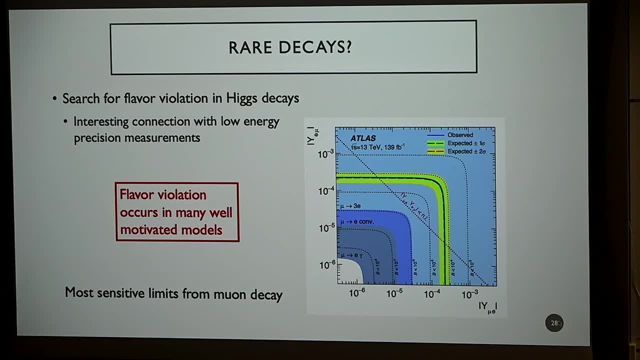 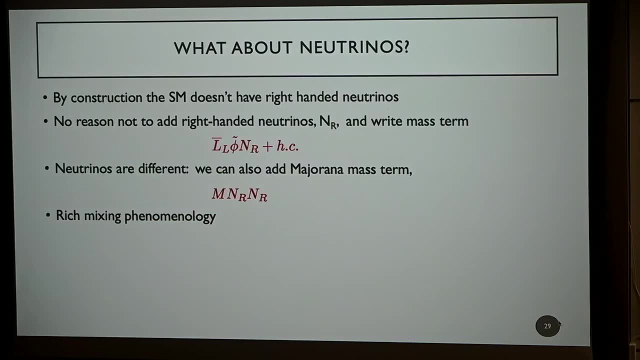 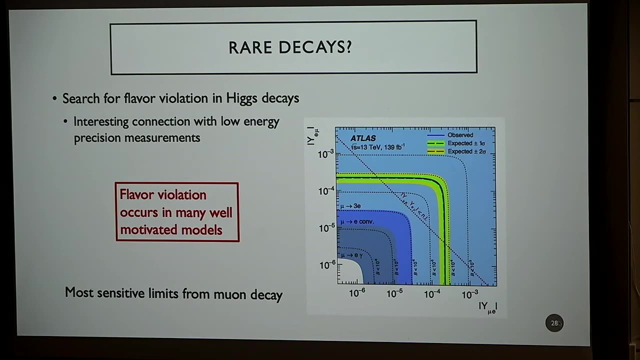 to the masses in a scale. It's not a rigorous bound, It's one theory thought: Oh, it's the observed limit. Ah yes, So it's the observed exclusion region. Yeah, Good point. Yet if we had found this: 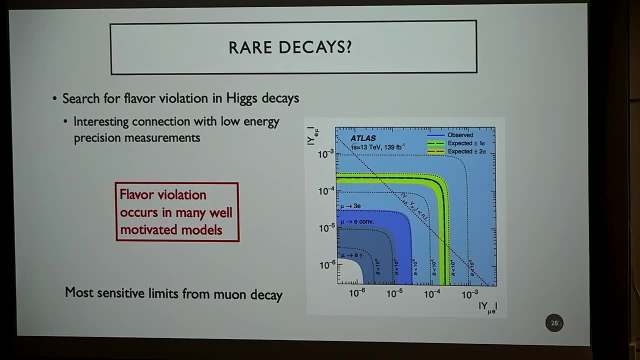 you would know it- You'd probably be reading it in the New York Times- if we had found flavor-violating Higgs decays- And in fact if we had found flavor-violating Higgs decays at the LHC, you might say you didn't need to do these things. 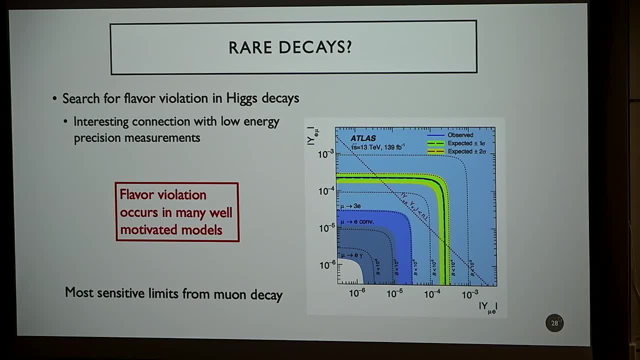 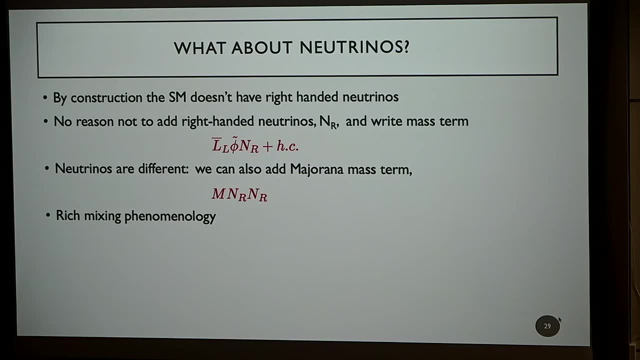 because we'd already found it, But no such luck. Okay, So I didn't say anything about neutrinos. By construction, we don't put neutrinos into our standard model, And this is purely by construction. It's purely an assumption. 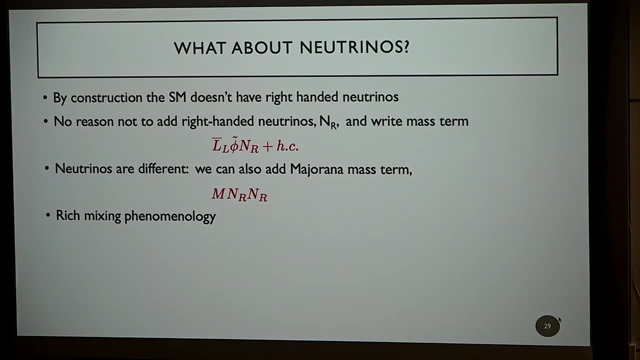 I could have put them in. I could have said: well, let's just have some right-handed neutrinos, the same way we have right-handed down quarks and right-handed electrons and right-handed other stuff. There's no theory reason why I couldn't have just done that. 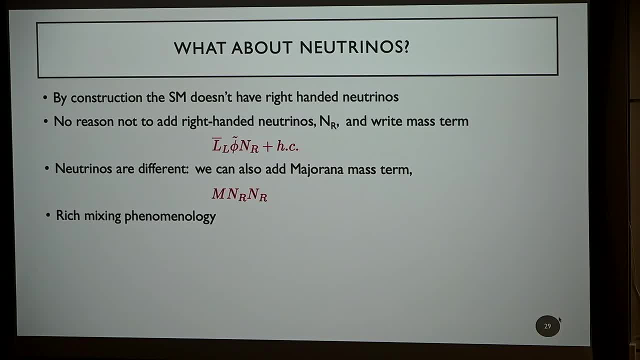 In fact, some people do. They're connecting the lepton doublet with the right-handed neutrinos. Bingo, it's the same as always. The thing is is that neutrinos are different, since they have no quantum numbers. We can also add a mass term. 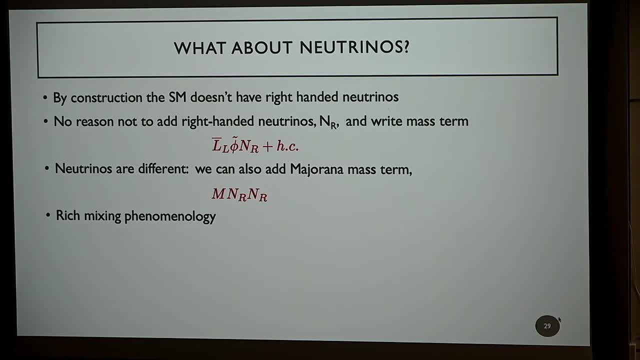 which is a right-handed, right-handed guy, a Majorana interaction, And so then you have two sources of masses for the neutrinos and it becomes very, very interesting constructing the mass terms for the neutrinos. So you get this rich mixing phenomenology. 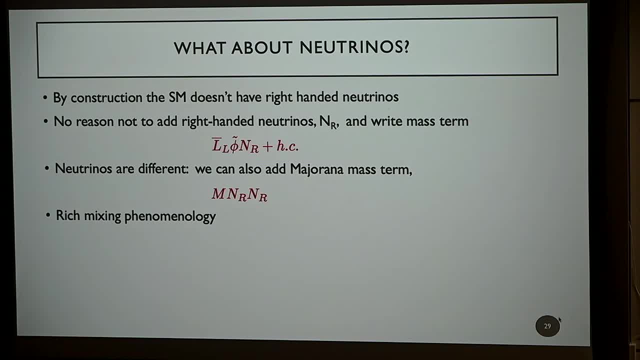 with the Majorana mass term and the Dirac mass terms. So that's all I'm going to say about it, But it's actually kind of interesting working it out. But it's very, very different than the quarks, just because of the possibility. 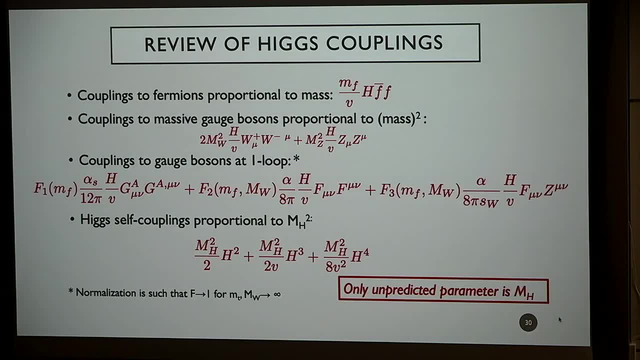 of adding this Majorana mass term. Okay, So let's just review this. here I've talked about the couplings to the fermions- are proportional to the mass. The couplings to the gauge bosons- Here I wrote mass squared and that's because it's Mw squared over V. 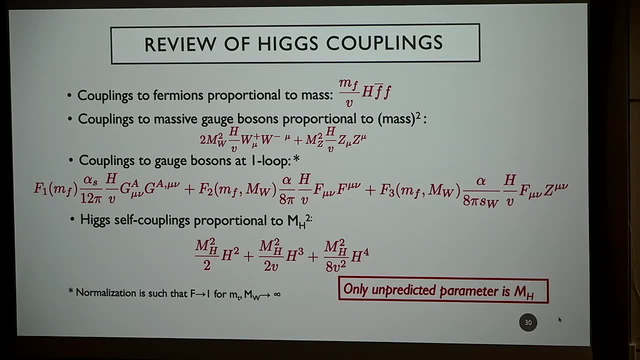 Sometimes I might write it as Gmw. you can go back and forth with these because I know Mw is Gv over 2, so take your pick. The gauge bosons don't couple to the Higgs at tree level, the massless guys- because the Higgs couples to masses. 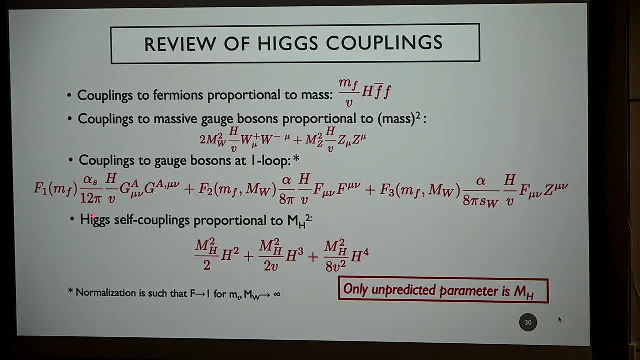 So the gauge bosons couple at one loop to the gluons, to the photons and a mixed term with the photon and z, And I've written it this way just because these functions out front are normalized such that they go to one when the stuff inside 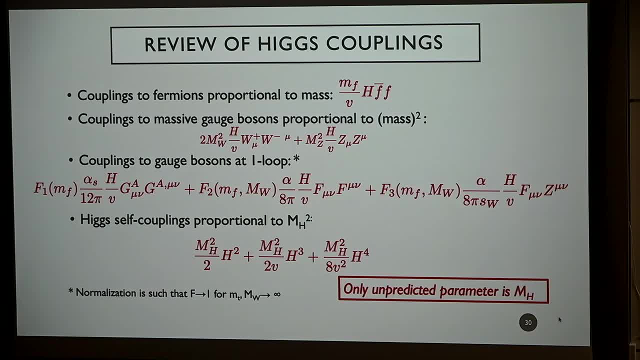 goes to infinite mass. But you can see that the Higgs will couple to gluons at one loop, it'll couple to photons at one loop and it'll couple to the photon and the z And this is a huge motivation for people who like to build models. 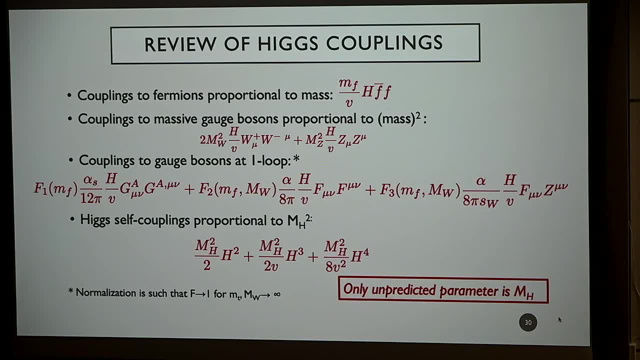 because, in particular, the coupling of the Higgs to the photon is pretty well measured, And so you can play with models where there's new charge stuff interacting in loops with the Higgs and try to learn something about it that way, Excuse me. 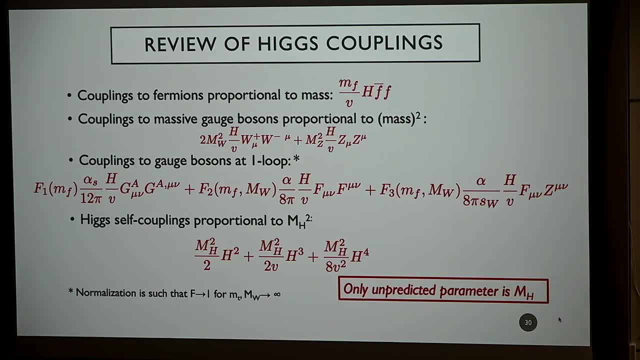 Again, just for summary, the Higgs self-couplings are proportional to the mass squared of the Higgs. So in this whole big construction here I've really only done two things. I've assumed that this mu squared parameter was negative. I've worked through all my algebra. 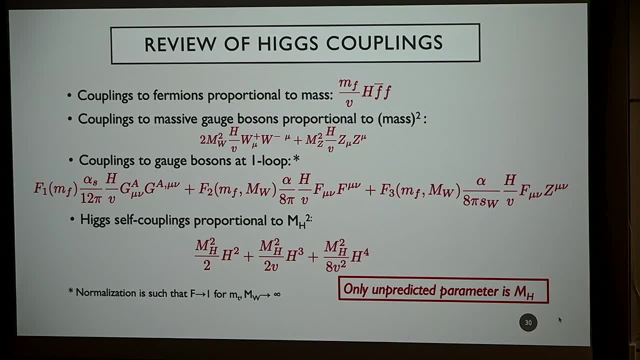 and everything is fixed now, except for the Higgs mass. So we have a theory which is full of predictions, Okay, Questions, Yeah, yeah, I will show. I do have that later. We'll get to that, Because that's a good point. 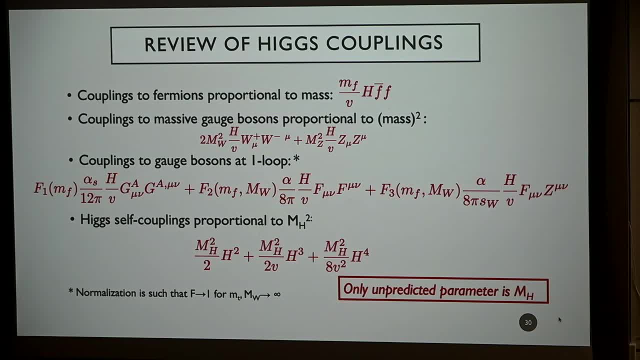 Because I've been tree lab. Yeah, Right, you still have to have this negative effect though, Yeah, And in fact, I'll talk about the Higgs potential tomorrow, Maybe tomorrow, maybe the next day, But yes, Because, yes, this is a very classical picture. 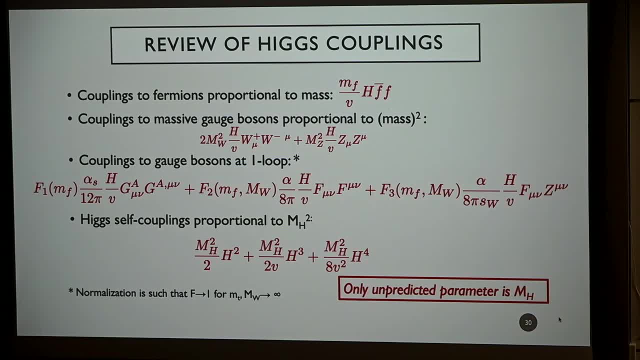 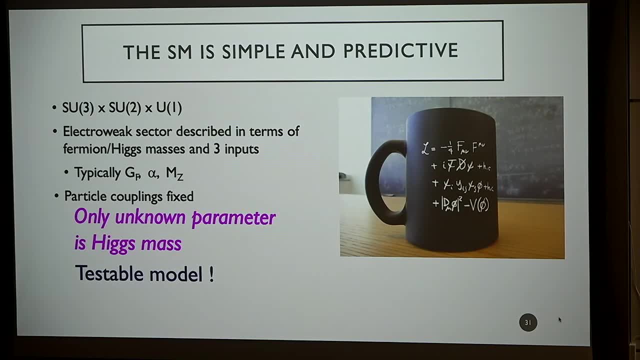 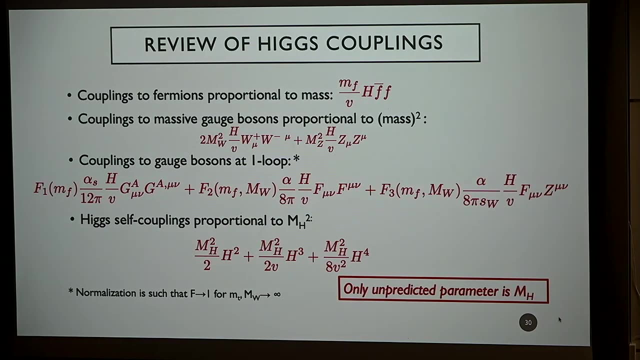 A spontaneously broken gauge symmetry. Okay, Simple and predictive. There we go. I don't know What was it. Oh, the little footnote. There's some function in front of these things. I just normalized it so that those things are one. 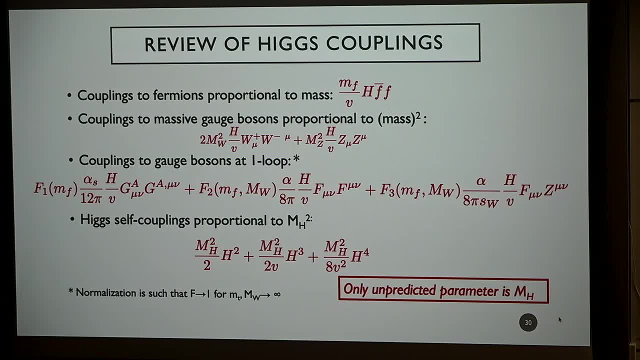 when the stuff inside becomes very, very heavy. That's useful for various reasons, But it doesn't mean anything. It's just normalization, Because I didn't tell you what those functions were yet, Right? So you write the standard model on a mug. 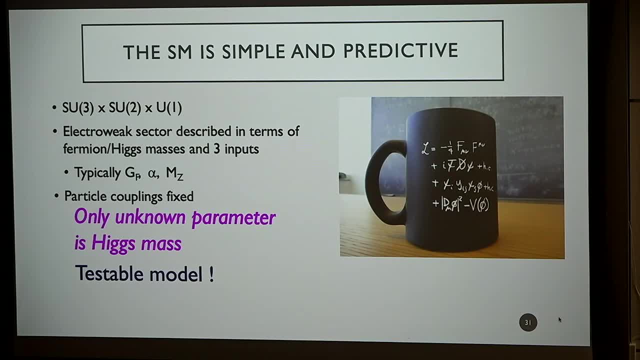 Anybody want to tell me what's wrong with the standard model on the mug here? Does it have two? It's missing the psi bar here. Yeah well, it's missing the psi bar, right, It's psi bar, phi. psi. 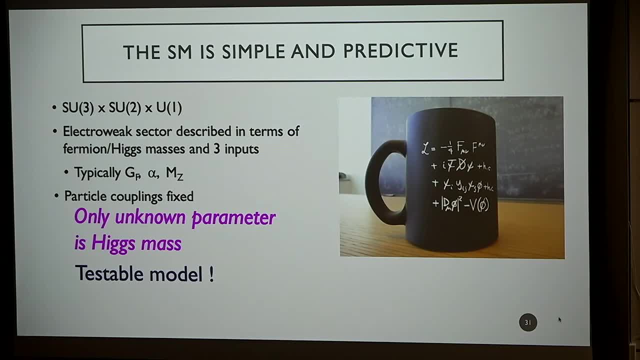 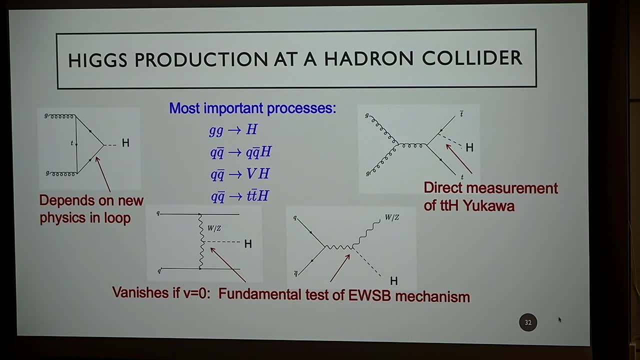 Which was pointed out to me recently. Okay, That's not my picture, but you know lots of people have those t-shirts and it's wrong. So if you're buying the t-shirt, you know you're scamming people. Okay. 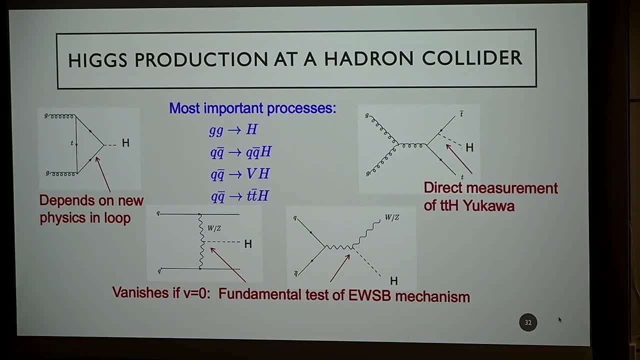 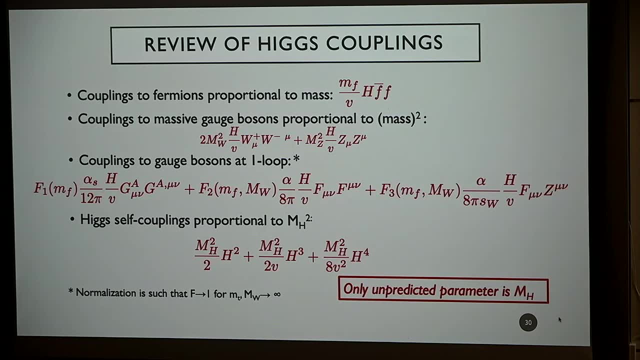 So now we've got this beautiful model. Yeah, Yeah, That's true. 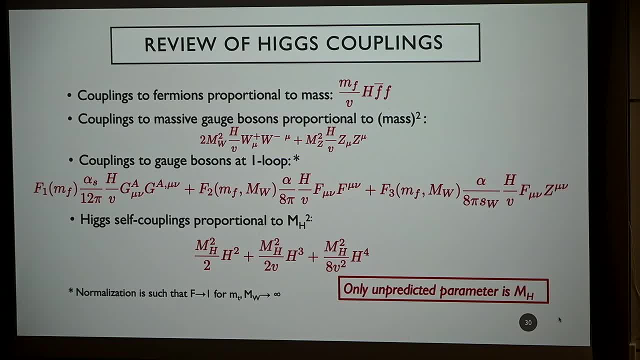 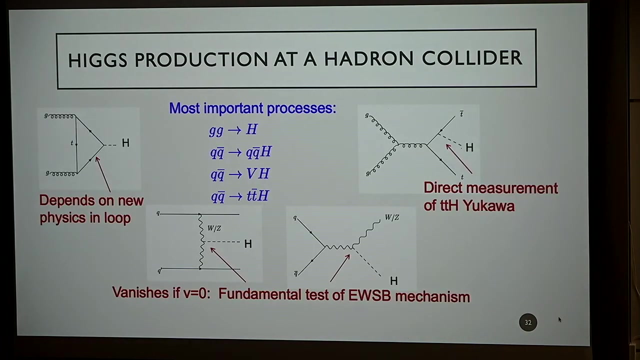 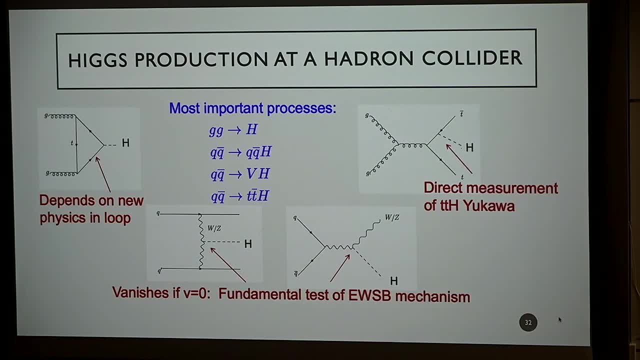 which connect the Higgs to the gauge bosons. So this one here we call associated production. 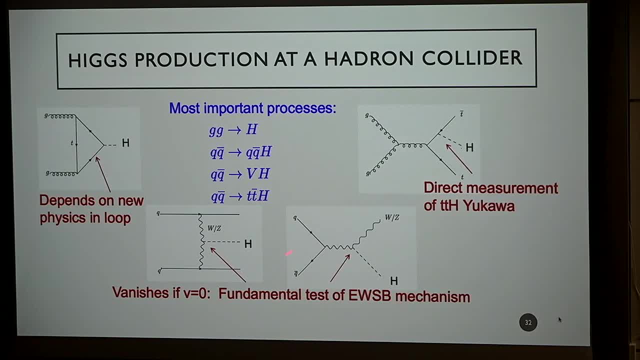 So it's QQ bar goes to WW Higgs, or QQ bar goes to Z Higgs. So this coupling here, the WWH coupling, is GMW, So it vanishes if V is zero. So if we didn't have the VEV, this thing would vanish. 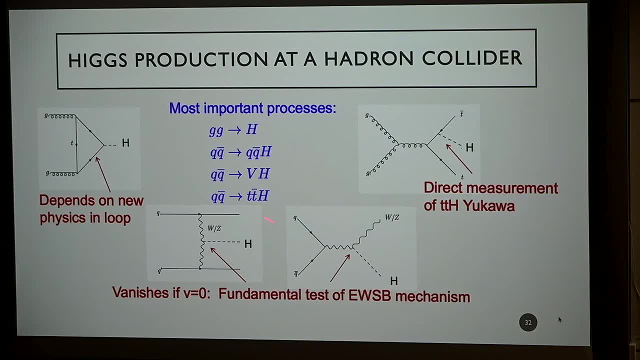 This is proportional to the same couplings WWH, and we call this vector boson fusion because it's as if the quarks spit out a W and the quarks spit out a W and the two Ws just fuse together to make a Higgs. 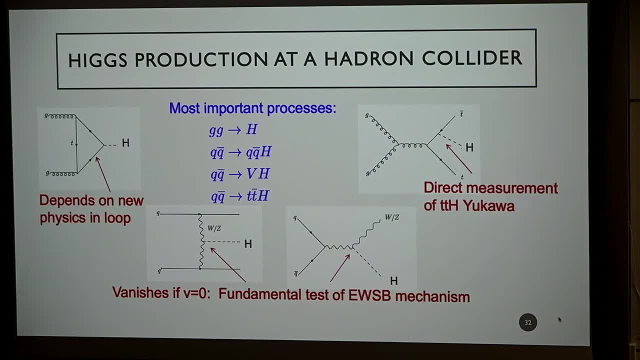 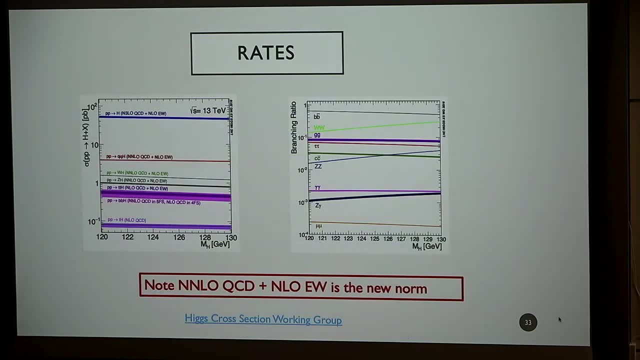 So again, this interaction would vanish if V were zero. So these are the really important ways we make the Higgs. And here are the rates and I just want to show this before I start talking about the individual things. So this is the mass of the Higgs. 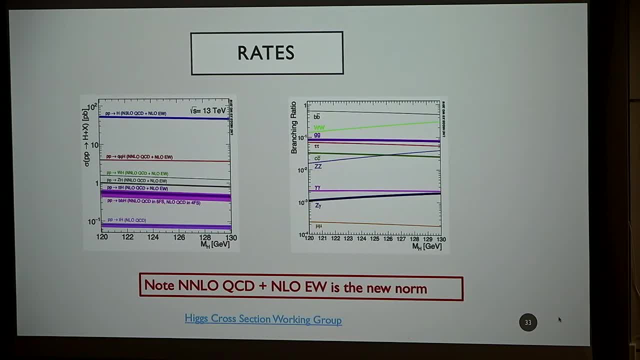 So these rates aren't very sensitive to what exactly the Higgs mass is. It's measured to be 125, but it doesn't really matter here. And here's the rates, And notice that this is a logarithmic scale. So here's the gluon fusion rate. 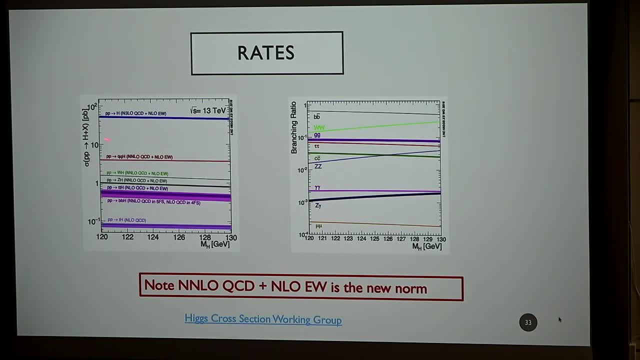 and it's an order of magnitude above all the other ones. So all these down here are much, much smaller contributions, But what you should look for, what you should look at on this, is a fine print on each of these lines, because each of these things are calculated. 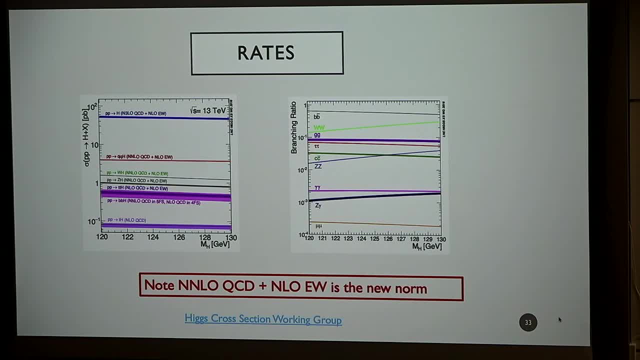 to NNLO QCD plus NLO electroweak, And this is a huge triumph of particle physics that we can calculate these things to next to next to leading order, And I hope some of you are working on this, because in order to measure Higgs properties, 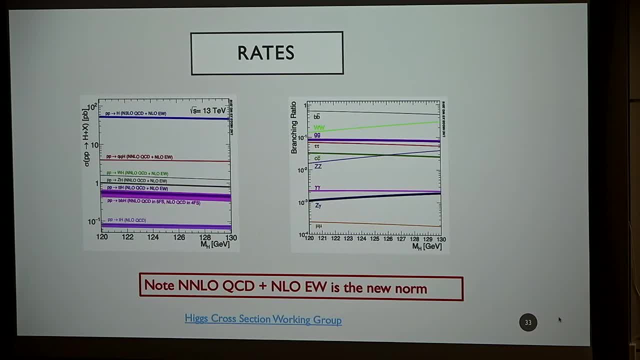 and to compare them with our theory, we need even further precision on our calculations. So, once we've made the Higgs, how does it decay? Well, since the Higgs likes to couple to mass, it mostly decays to BB bar pairs. 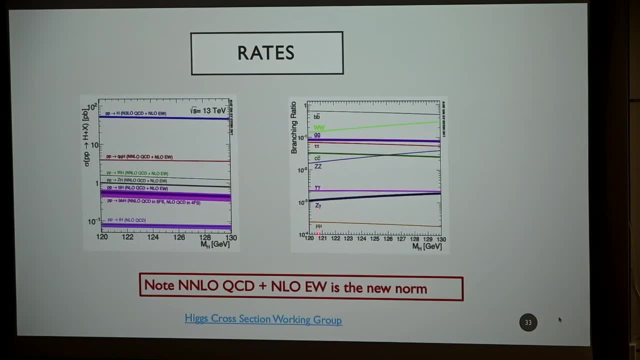 So this is the branching ratio. Again, notice that this is a logarithmic scale here. So here's the Higgs to BB bar, Three orders of magnitude. down here is the Higgs to two photons, and then there are a bunch of other Higgs things. 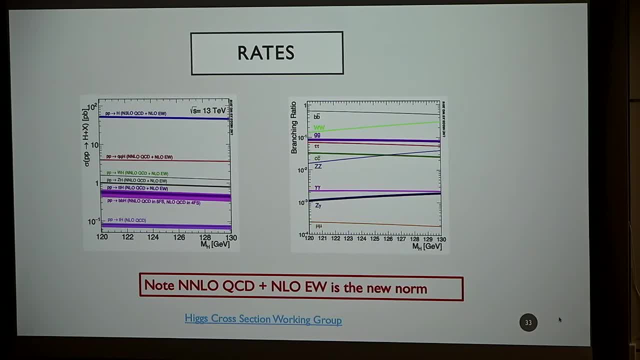 So when you see WW, you're going to be able to see the Higgs to two photons. So when you see W here, you should turn your brain on and say, um, does that make sense? What's plotted here, Right? 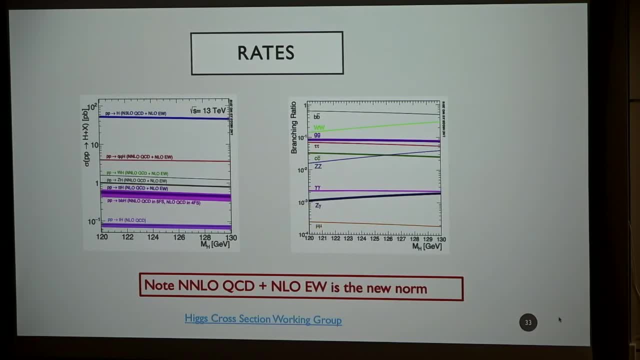 Because the W mass is about 80 GV and the Higgs mass is 125.. So what is plotted here is not really WW, can't be right? Yeah, So thinking of those QCD corrections, QCD is non-perturbative. You don't say they're any good. What do you mean? QCD is non-perturbative. These are calculated in the perturbative regime Where the coupling constant is 0.118, and it's a perfectly well-defined perturbation theory. 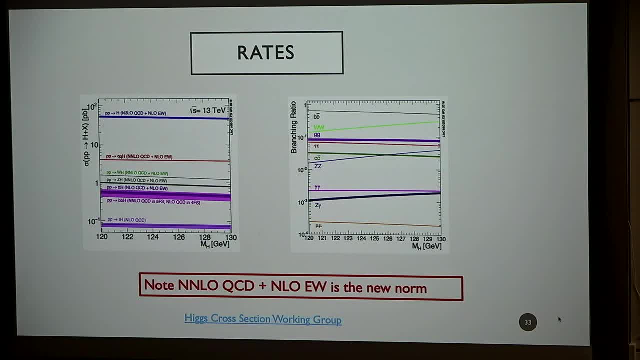 We calculate at PT above I don't know- 10 GV or someplace. But no, they're absolutely calculated in the perturbative regime. OK Yeah, We're not calculating like the lattice guys do at 1 GV, where the coupling is very, very big. 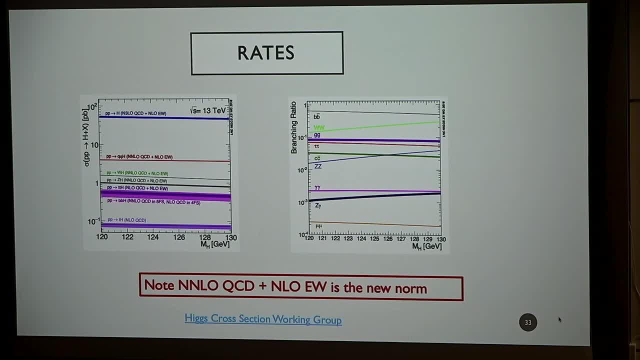 Yeah, I guess. actually I have a follow-up. Isn't the LHC running in the non-perturbative regime, though? What do you mean? No 13. 13 TeV, I guess, is still within the perturbative regime. 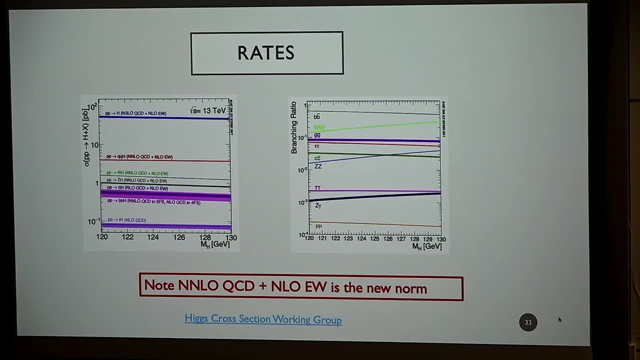 I don't have a plot today, but I'll dig one up for you tomorrow, Because what we're colliding at the LHC is the partons, the gluons and the quarks. So when we collide the gluons together to make a Higgs, 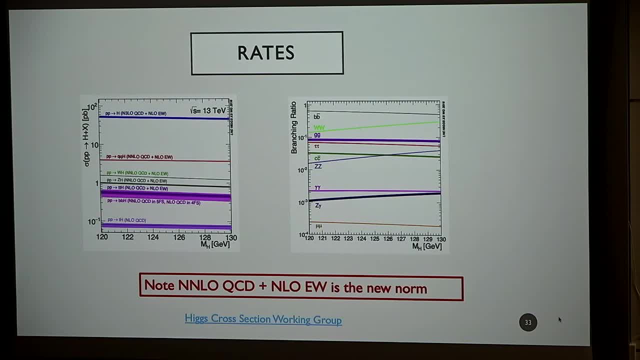 the invariant mass of the two gluons is the Higgs mass right, Because it's mostly produced on resonance And at the scale MH equals 125, alpha S again is: I don't know, it's probably 0.11 or something. 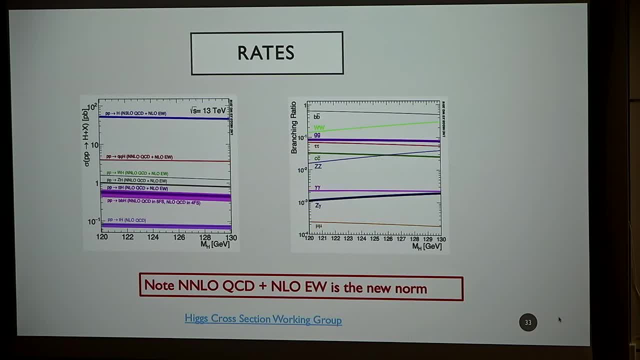 So it's perturbative. But let me continue with what WW means. Anybody know I'll take comments, Yeah, Yeah. So really what it is is one W on shell and the other W going to two fermions. So all those branching ratios are hidden in there. 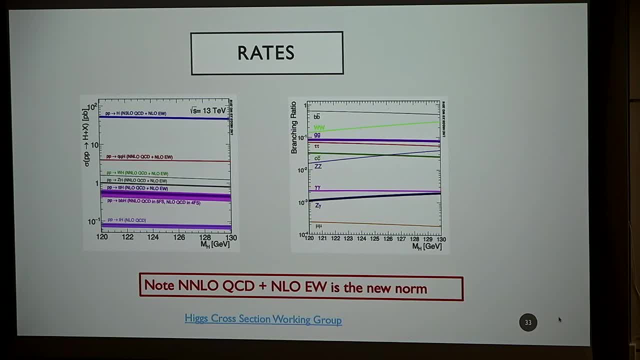 So this is a three-body decay that we're doing. Yeah, Yeah, It's a shorthand for a three-body decay. So, for example, ZZ is clear here. So I've got one Z. The Z is decaying to whatever two leptons. 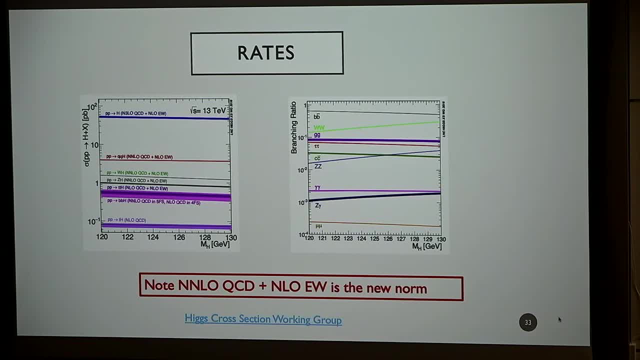 So I know it's a Z, because I measure those two leptons, I reconstruct their invariant mass And then the other Z is going to all the fermions here. So yeah, this is kind of a shorthand way to show it, So it's a cheat. 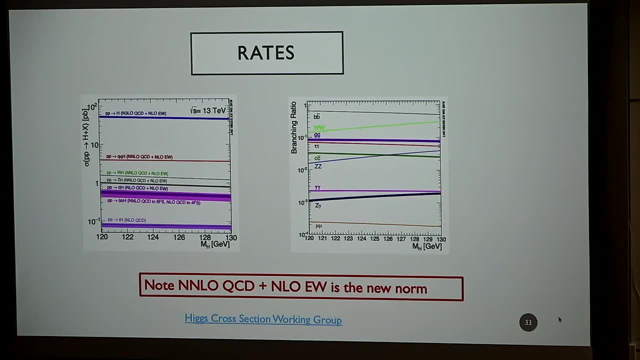 OK Yeah, I don't know if this is quite a well-planned question, but I'm a little curious about how the Higgs looks kinematically at kind of the end stages. How would we actually detect it? Oh, I'll show you that. 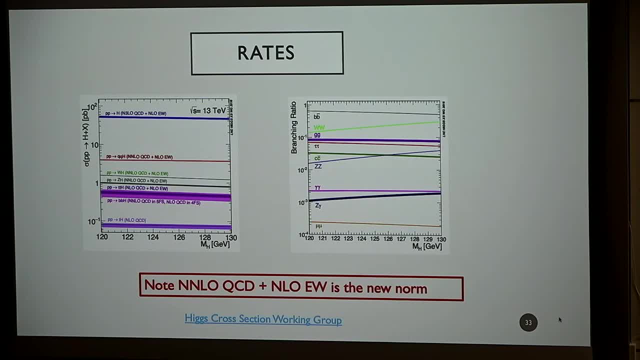 That's coming. Yeah, I'm going to get more and more detailed and I will show you that And that will address the question about is it perturbative and so forth. So can you make a comment on why the branching ratios seem? 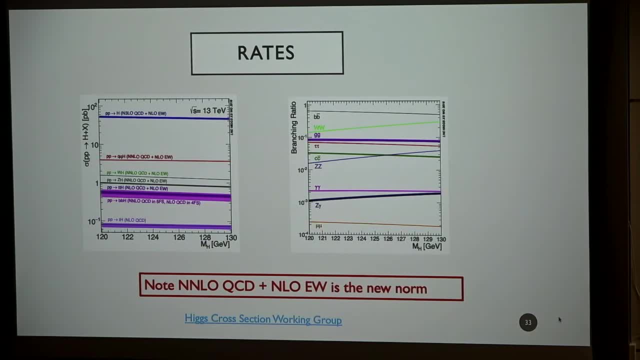 to go up for gauge bosons but down for the quarks, I guess, and the muons as you increase the Higgs mass. Oh Well, it's because of this business of we're below threshold right, Because we can't really make the two W's. 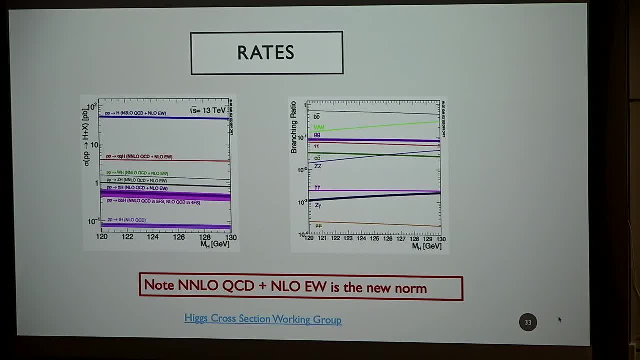 So we're approaching the threshold for this, And so it's a three-body decay versus a two-body, basically. But I mean we know the Higgs mass, But it's the difference between two and three, So that means that the increase. 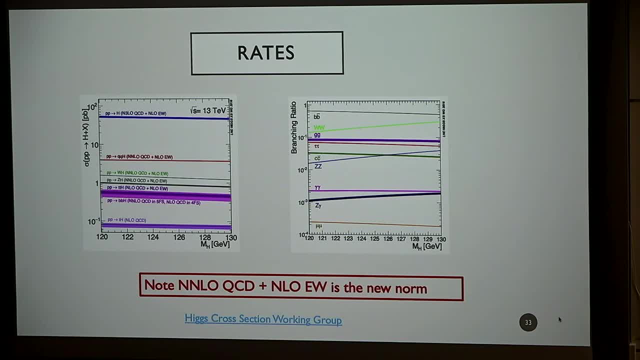 is mostly due to the increase of the. It's just different, right. I mean, they're spread out differently in phase space And in fact, if you want to be really boring, I could calculate that for you. I like calculating stuff. 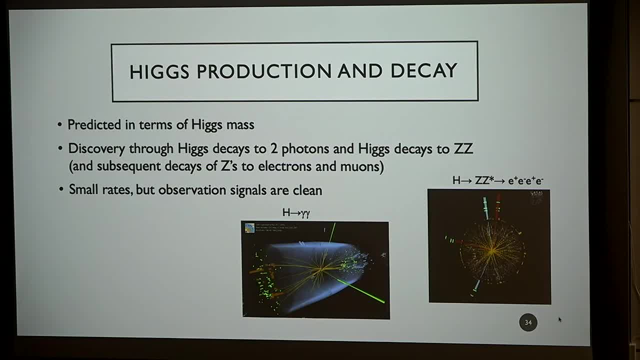 Actually it's not boring. I love calculating stuff just because I think you learn from it how things are different, And in fact, what I'll do is add to my notes the reference to somebody who calculates this stuff in gory detail, because I think sometimes 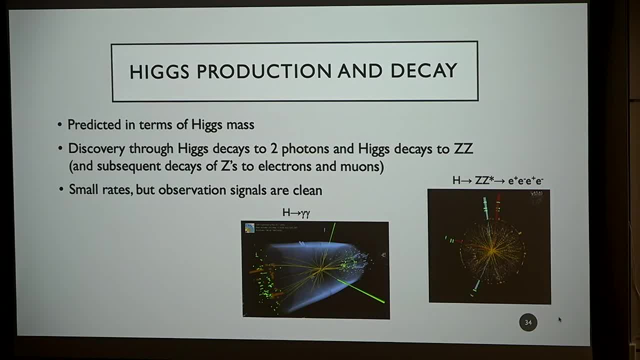 that's helpful. So I have just a few more minutes, So I'm going to show you some public relations slides because I think they're so cool, just to show you where we've gone here, Because, as I said, the Higgs production- it's predicted. 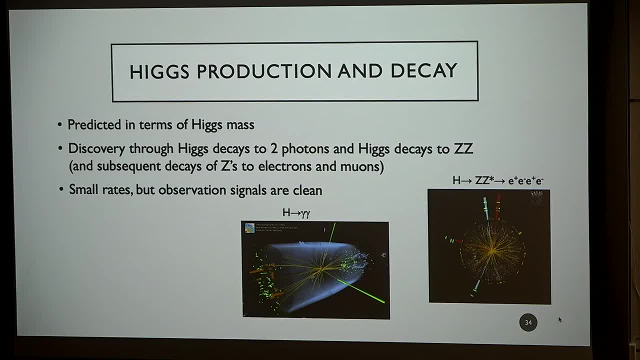 It's predicted in terms of the mass, And now it was discovered 10 years ago through ZZ star- the one we've just been talking about here- and gamma gamma. So, even though the gamma gamma branching ratio is 10 to the minus 3, it was a discovery channel. 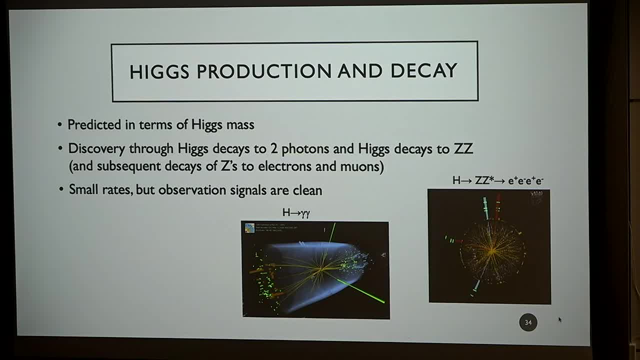 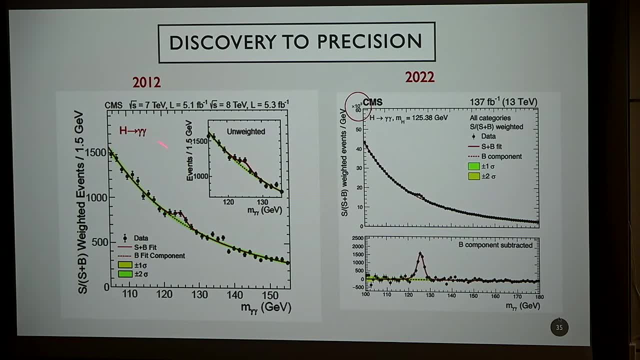 because it's so clean, It sticks out so much above the bat, It sticks out so much above the background. So where have we gone in the last decade? And so I think it's interesting to look at these? So this is the Higgs to gamma gamma spectrum. 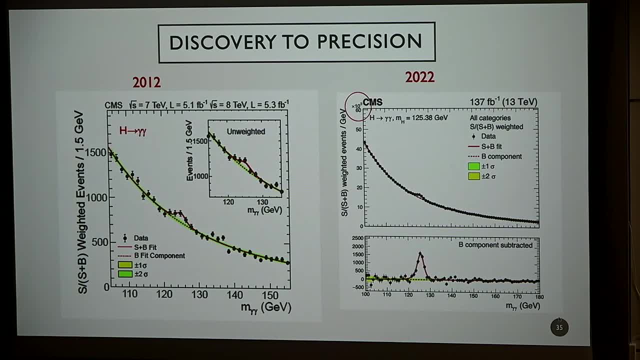 So you're looking for two photons. Now at the LHC there are lots of photons floating around. You can make qq bar goes to two photons. That's this whole thing falling down, And the Higgs is this little pimple here. 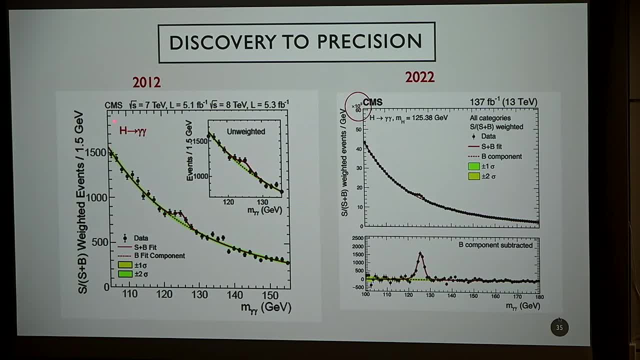 So here was the discovery And here we are 10 years later. But look at the difference in the scales: 1,500 to now. this is 10 to the third here. So we really have a lot more Higgs bosons to measure this kind of little bump here. 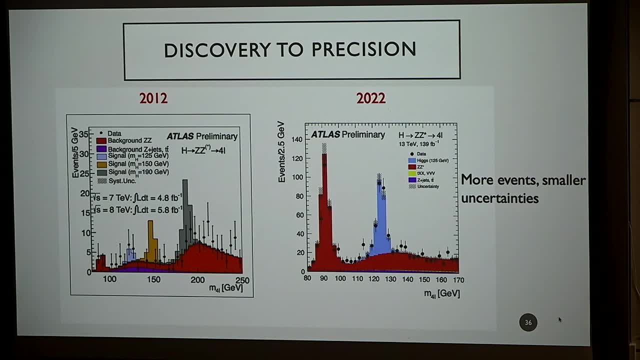 And it's the same thing for looking for the Higgs to ZZ star- that in 2012, we had what? 30 events. So this blue one here is the observed Higgs, And over here in 2022, we have 100 events. 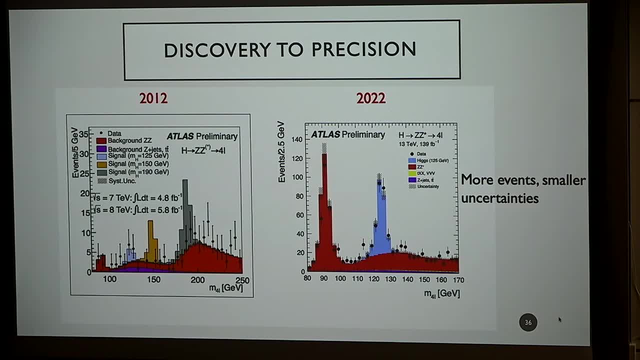 So we have smaller events and smaller uncertainties. Yeah, Why do you not bother about how you produce Higgs? Well, no, what they do is they add them all up. So in your Monte Carlo you've got glu. glu goes to Higgs. 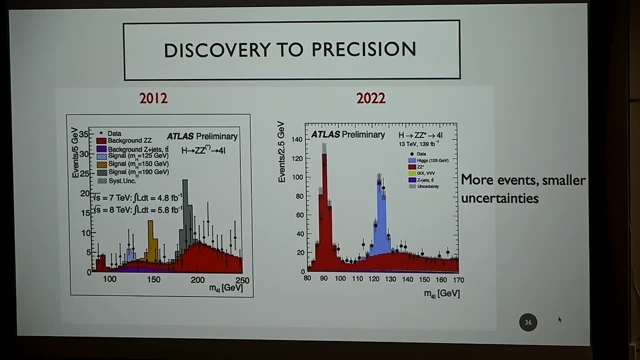 You've got glu. glu goes to glu plus Higgs. You might have the other stuff, But the other stuff doesn't really matter because it's so much smaller. So no, I don't care how I make it, I put it in my Monte Carlo and out it comes. 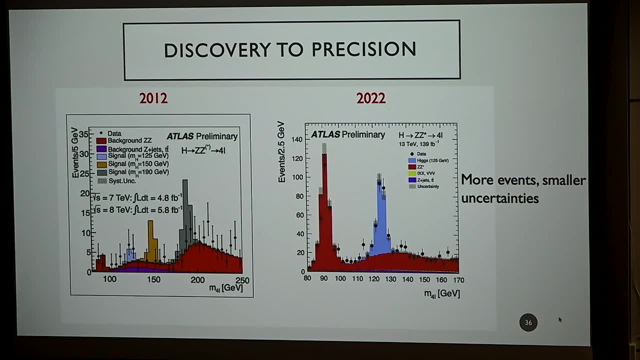 Yeah, Why is the signal a little bit bigger? or is it heavier on the physical Higgs than the 150 and 190 on the quantum 11?? Oh, this guy, Why would this signal have been bigger than this signal? Well, the biggest background is from Zs. 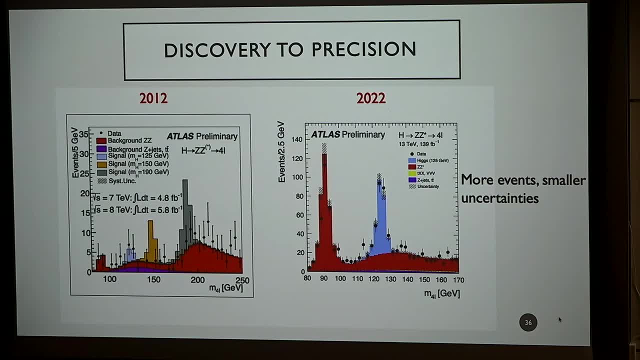 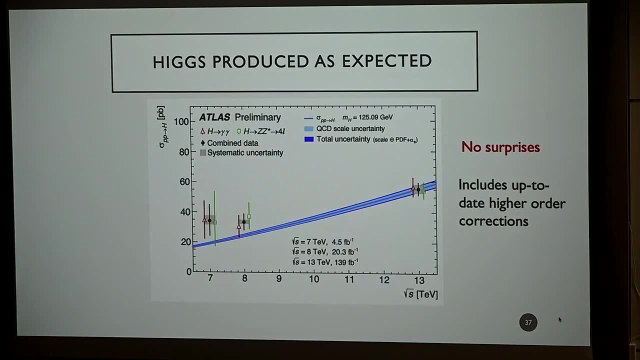 So the signal sticks out more from the Zs than it does here. OK, And as I was advertised, there is nothing, nothing, nothing, sadly nothing surprising in what we see at the LHC. So when we calculate all these cross sections, so here we go. 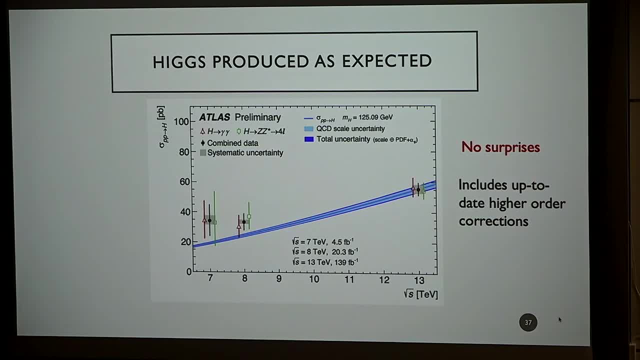 Here's making a Higgs, Higgs decaying to photons, to Zs. Here up here we have the predictions and the data. It looks just right. The earlier data had larger uncertainty, See the size of the error bar. 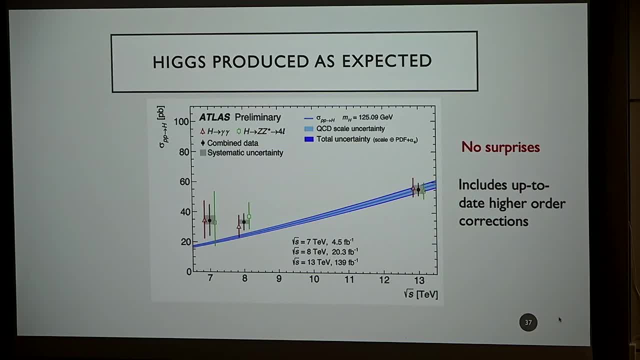 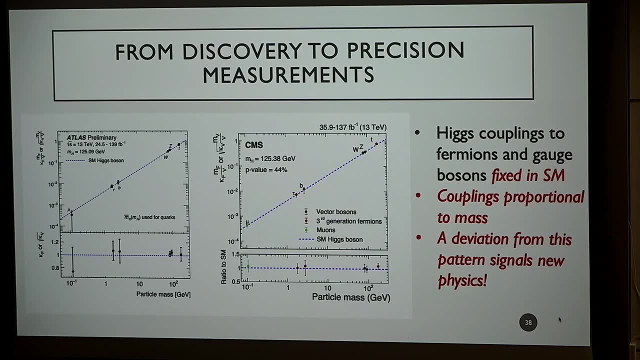 It's larger, But it pretty much just looks exactly like what we think. So this is my last slide, I think, for today, before I go on tomorrow. So we're really changing how we study Higgs physics, because we now have more than discovery. 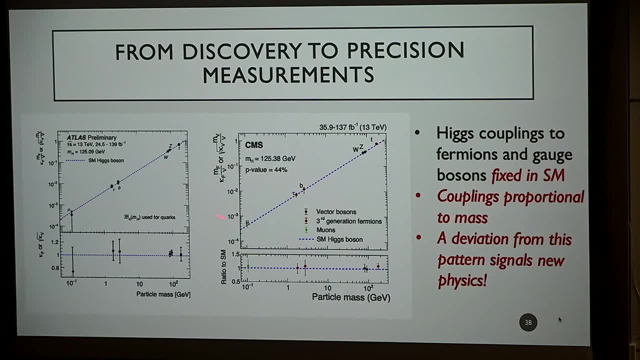 We've got these precision measurements, We've taken our measurements and we've measured the coupling strength of the Higgs as a function of the particle mass- CMS Atlas. to be politically correct, This plot is logarithmic and this is linear. 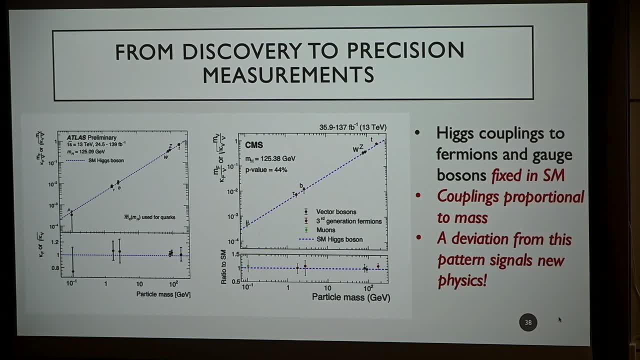 And we see that even on a linear scale it looks like things are pretty much just like what we expected, And I have to say again, if it's not one, it's new physics period, That's it. So any deviation would signal new physics. 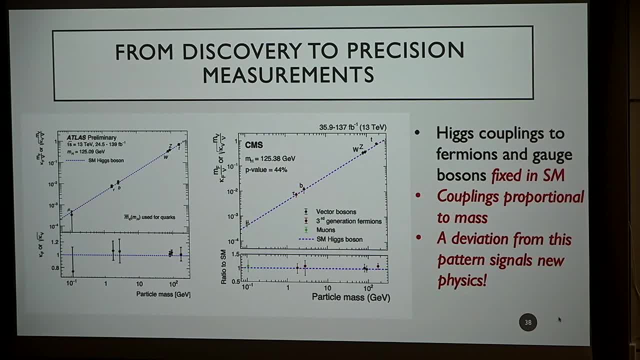 So I'll stop here and I'll take questions. I'll be around all day for questions. Yes, Yeah, I've got that tomorrow And I do have it and it's cool and I'm going to tell you that why. 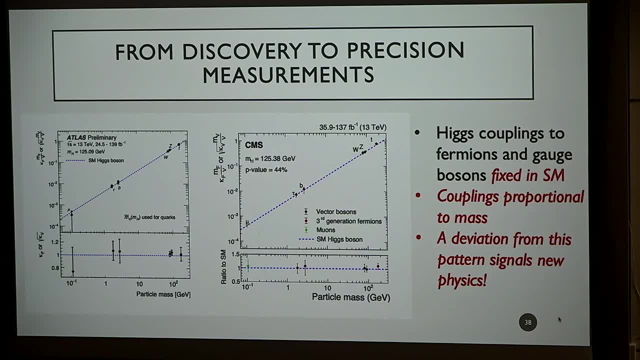 Did anybody here write a paper about this? I knew there would be people right And I'm going to tell you why the Higgs comes in. Yes, I definitely. I think that's a sociological question. Because of plots like this, we get super excited. 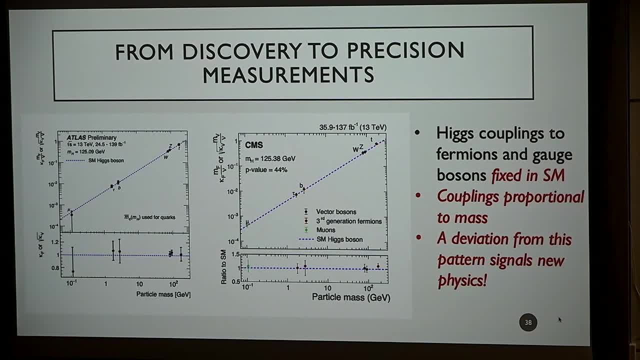 when we see something that looks like it might not be the standard model. That was the W mass from CDF. That was the 750 to two photons. You know, we really want there to be new physics, And so as soon as we see something, 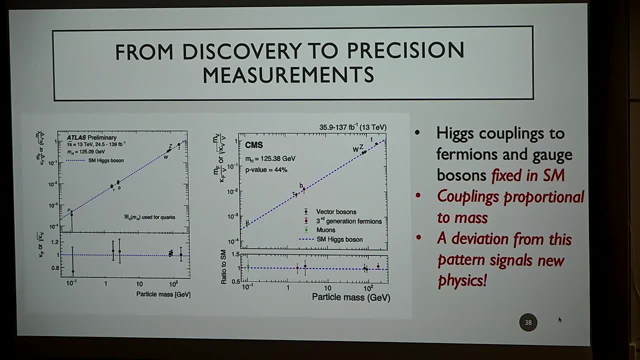 that we think it's new physics. a lot of people are thinking about: well, what could it be? And so, like I said, one of the things that I think you should get out of these lectures here are the things you check when you're building your new model. 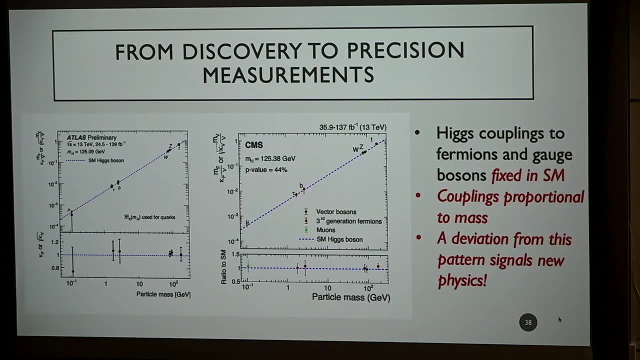 to explain something. Yeah, I just didn't understand why the H degrees didn't come in so hard. when you have the Oh, you just have more. It looks like you have more degrees of freedom. Why is that like OK. 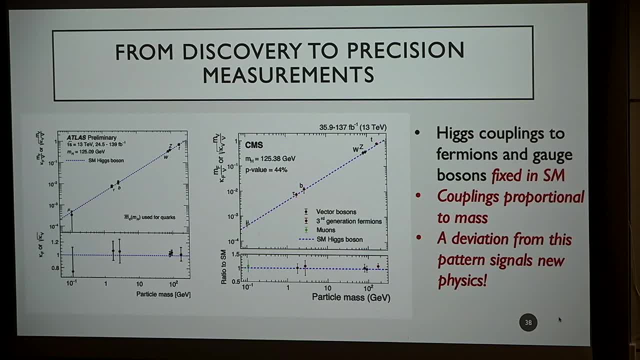 Well, this counting is too simplistic. It's just to sort of get in your mind that we had the scalar field and now we have longitudinal degrees of freedom. It's a simplistic argument. You know nothing deep, Yeah, Yes. 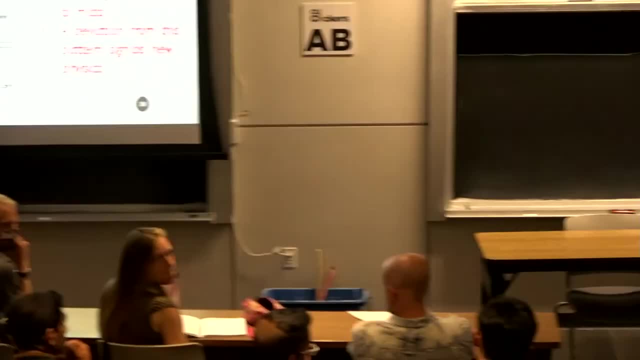 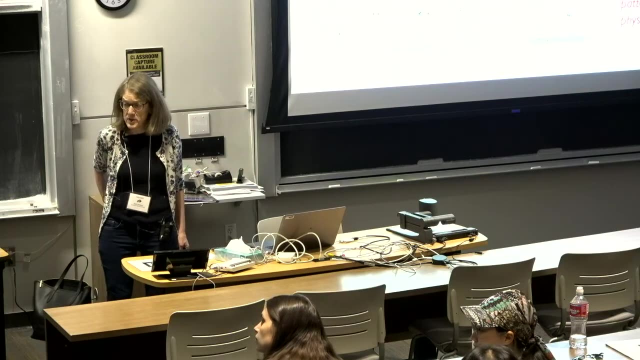 I guess, is there, we're pretty like good, We're pretty sure about the Higgs mass being around, where it's at roughly now. Right, It's measured to 1% precision, Right? So So, yeah, we're pretty sure. 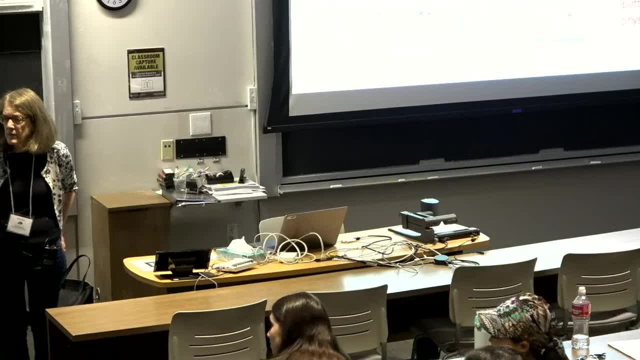 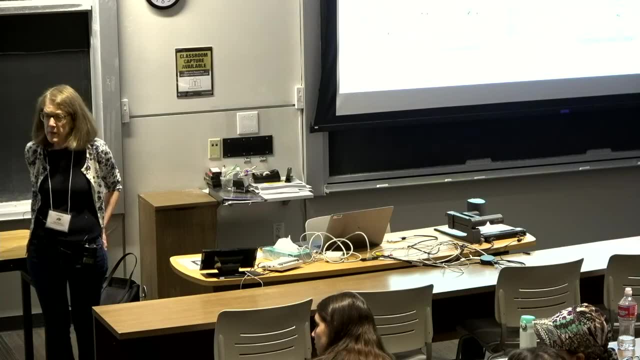 Yeah, The reason I ask is mainly because there's also a very like interest, Like it's sitting at a very interesting place right in terms of 129 versus 129.. I have that in my lectures coming up. Yes, you'll see this. 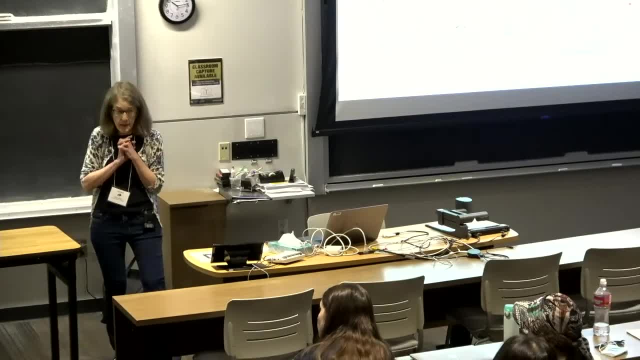 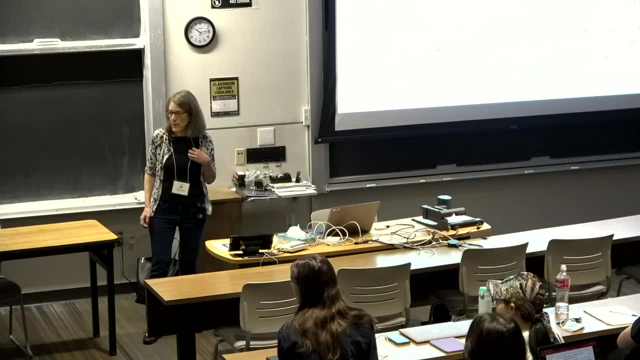 This comes with the potential. What does the whole thing mean? Yes, That is coming. Yes, OK, Go ahead. The branching ratio, the Higgs to gamma-gamma was a higher branching ratio than Higgs to mu-mu. 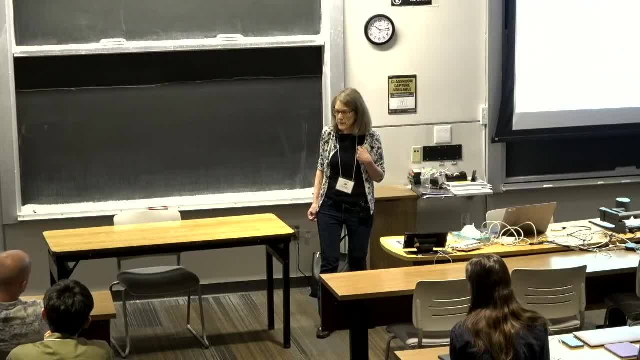 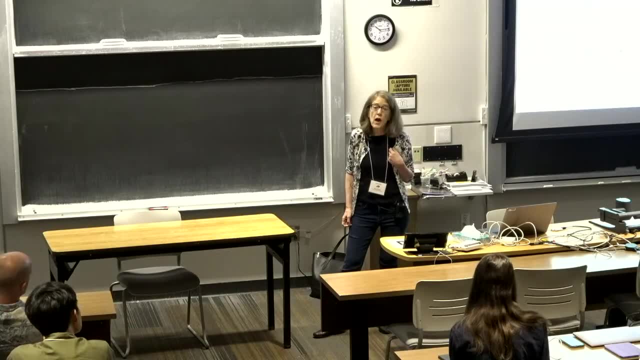 Yep, And I guess with the Higgs to gamma-gamma you just have a top running through the loop, So you don't take too much for a hit. Is that what's happening? No, the Higgs to gamma-gamma, you have a top. 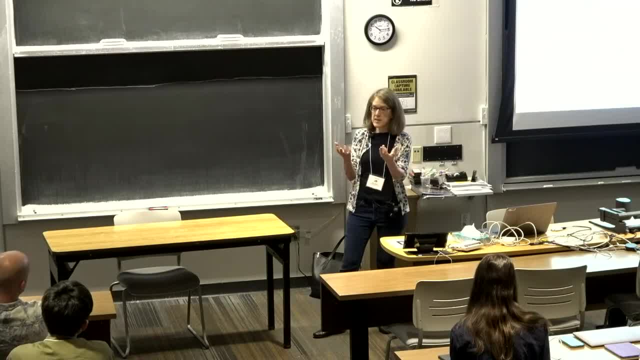 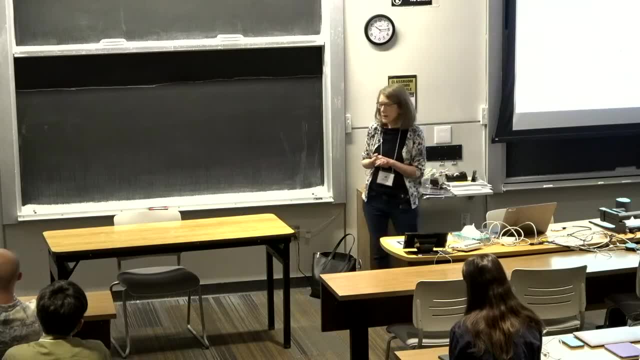 but you also have a W And there's a playoff. They have opposite signs. The point about Higgs to gamma-gamma is that the background is easier to deal with than Higgs to mu-mu. So it's all about signal and background. 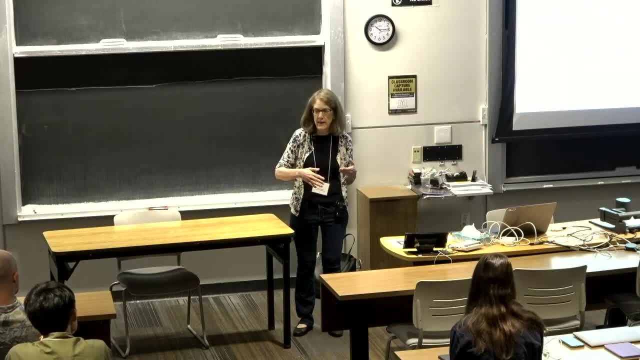 So you can't look at the branching ratios and say, oh, this is bigger than that. You have to look at the signal and the background together. Is there a good way that we know that this Higgs to gamma-gamma is Higgs and not? 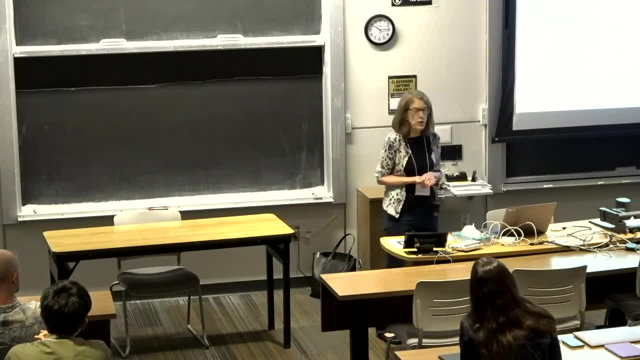 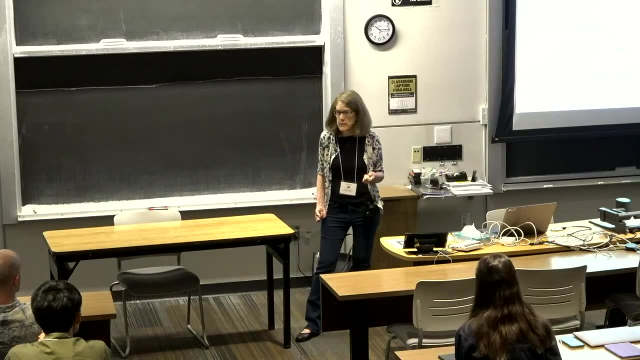 some exotic meson or something. Sure, because you measure two photons, You get their invariant mass and it's 125.. Right, but it could be something else that decays the two photons that we want to have out, But then you wouldn't get that. the invariant mass was 125 GeV. 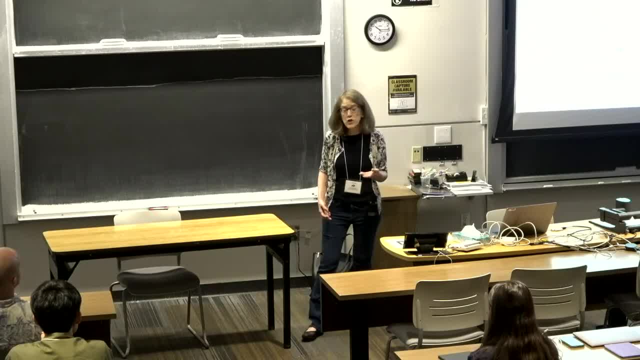 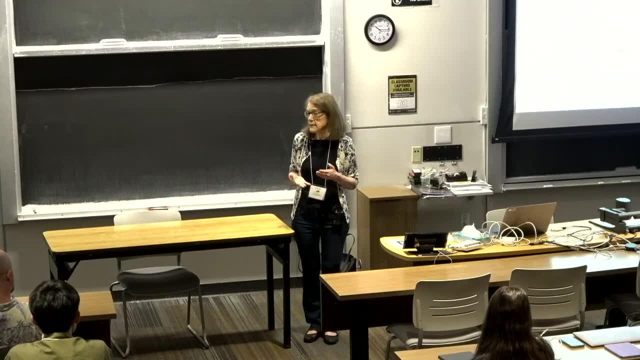 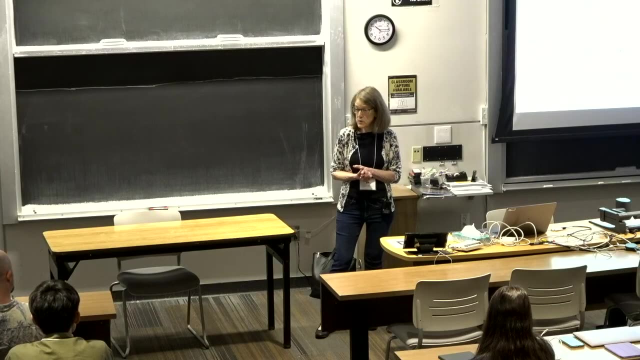 But if this thing weighed 120?? But we don't. No, I'm saying something else. You're saying: is the Higgs something else? Yes, that is. Could the Higgs be? Well, we know that this 125 GeV object decays to W's Z's. 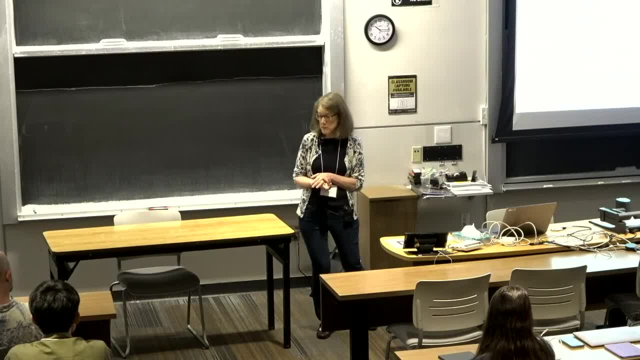 bottoms, exactly like we think. We've measured its spin parity very precisely, so we know it's 0 plus plus. For me that defines a Higgs. Yes, Right, Yeah, OK, One more question, then it's coffee time. 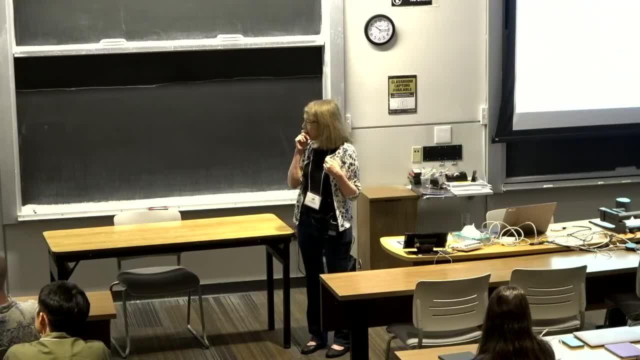 Yes, So it seems like most of the things that you've done in Higgs is precision-physical, Is it? Yes, So is the LHC better there, or like an E plus E minus collider that you mentioned before? I will show you that. 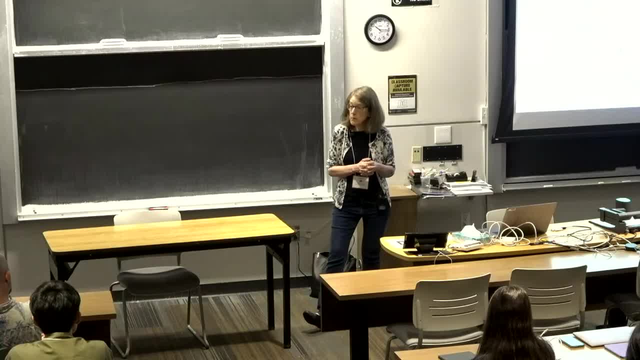 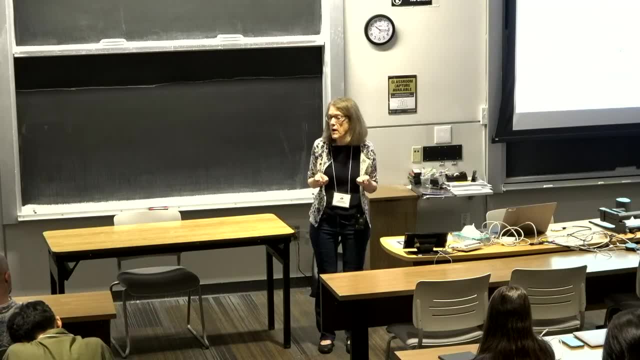 But the E plus E minus colliders can get very much more precise measurements than the LHC. But the LHC is not so much worse than the E plus E minus colliders Because, remember, the LHC is going to run until you have tenure. 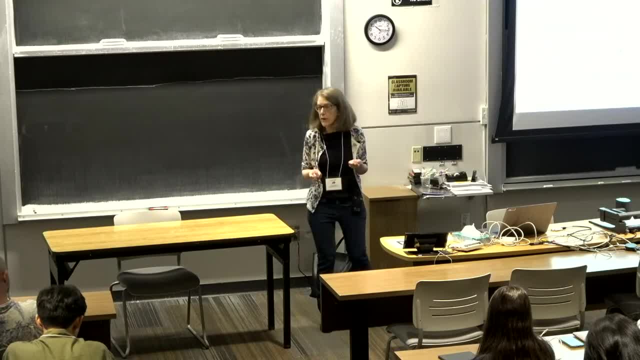 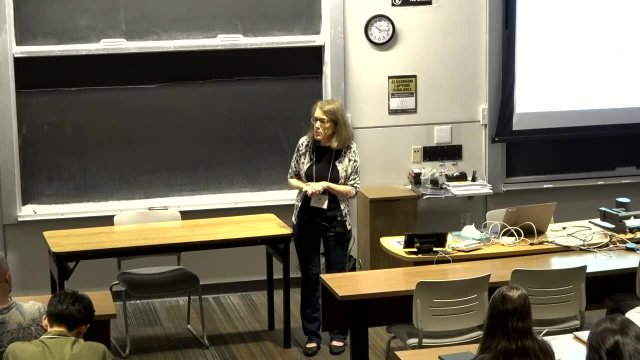 So they're going to get a lot of data. So the square root of n is going to be small, Whereas the E plus, E minus colliders won't start until I'm dead and buried. So the projections are not so different. It's a question of time scales. 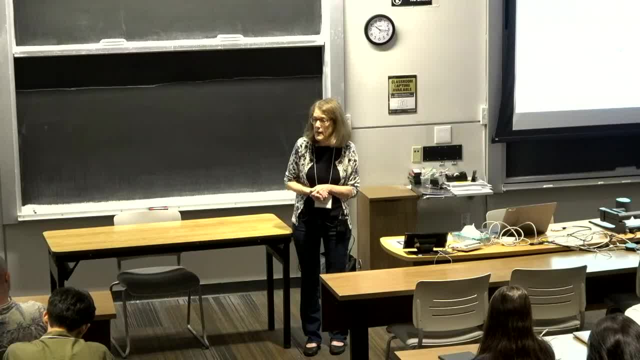 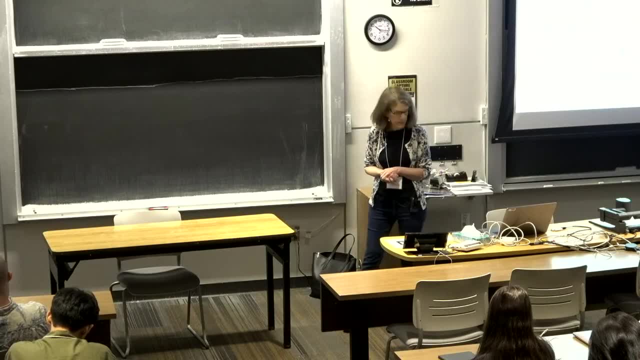 But is there something one can do that the other cannot? Yes, And I will talk about this coming up and it's a measurement of the Higgs whip, without making a lot of assumptions, Because, let me, I'll put this in the chat. 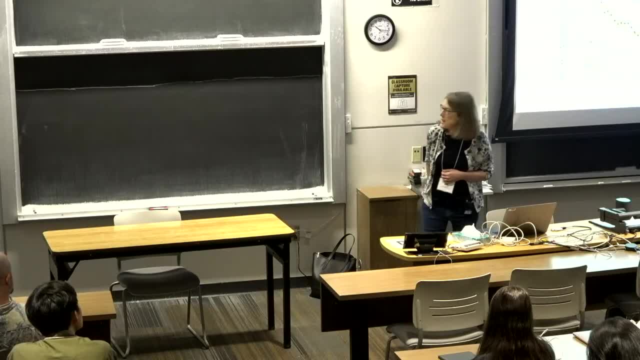 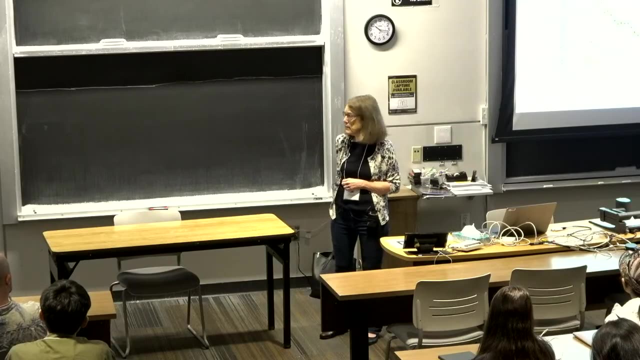 I'll put this up before we stop. You will see, by peering at the scale here, that the Higgs whip is extremely narrow, And in fact it's narrower than the resolution of the detectors. So the LHC has to be extremely clever to measure this. 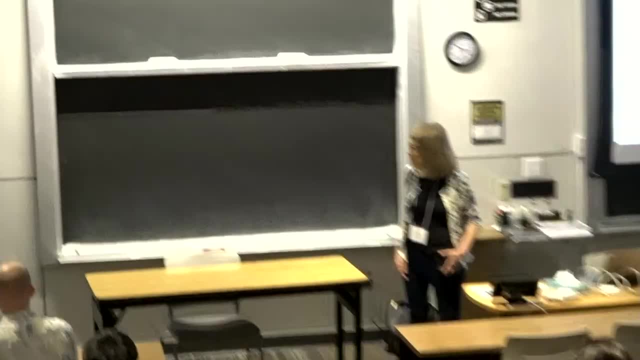 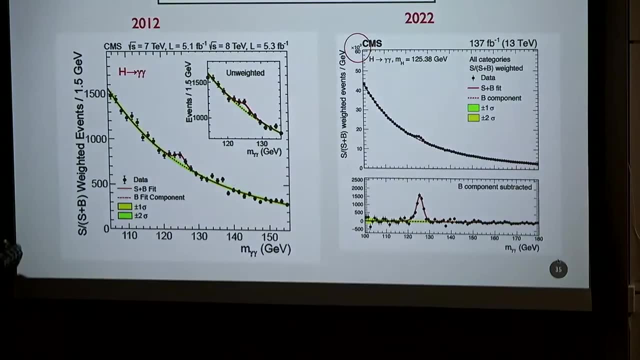 OK, We'll stop. You can get me a coffee break, Ethan. He's got something to say. I ended on time. I want my gold star. You're perfectly on time. actually, The coffee's still getting set up, so I'll take another minute. 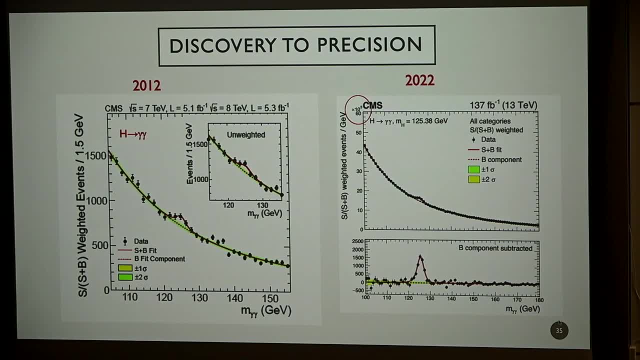 So I didn't make an announcement earlier about the COVID policy. I asked it all by email. I don't know if you know about the policy. That's an option for your comfort level, But one thing we are going to encourage you to do: 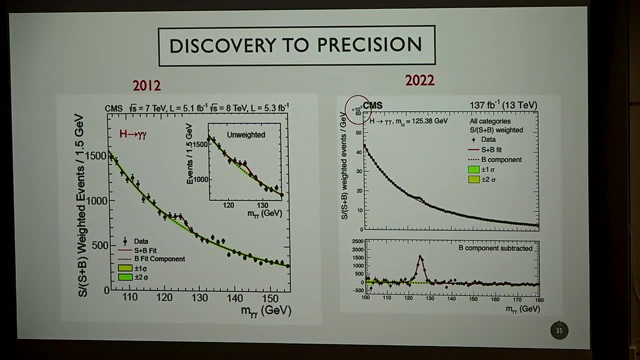 is: try to take a couple breaks outside, because we're right next to the outside door. It's very peaceful today, So the coffee was set up right outside the right door And you can go ahead and go take it outside for a while. 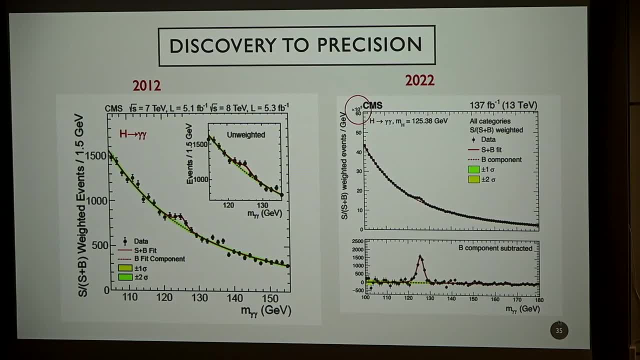 We'll reconvene at about half an hour. Good, Thank you very much. We have seconds. Yeah, Actually, I just want to clarify my first question. OK, if you have something like Uh huh, We were just trying to say that. 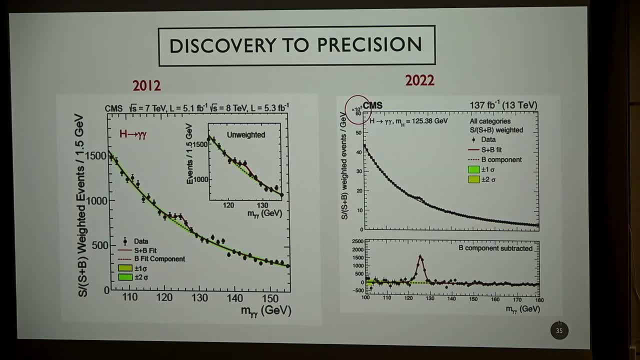 Well, that's really not physical, because I mean we've got this gauge boson and that's its mass, Right right. So I would measure the transverse and the longitudinal guys by their interactions, Right right. 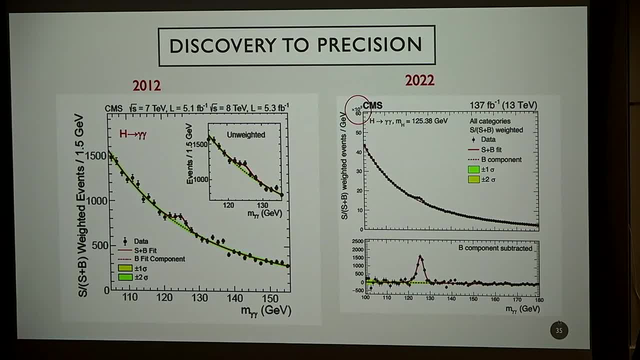 So this is not a physical question. is my point Right, right, yeah, Right, yeah, Okay. that's because I thought you might want to say something. No, I mean, this is the mass term, Okay. 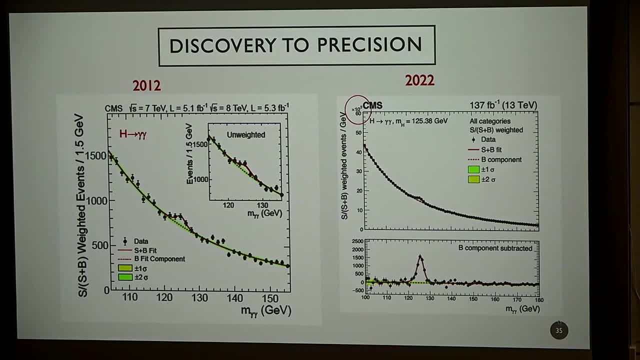 Yeah, Right, But I'll go through if I get to it. I have an example where I go through the couplings Right, And that's the point is how they couple, Yeah, I mean. I'm sure there are plenty of examples. 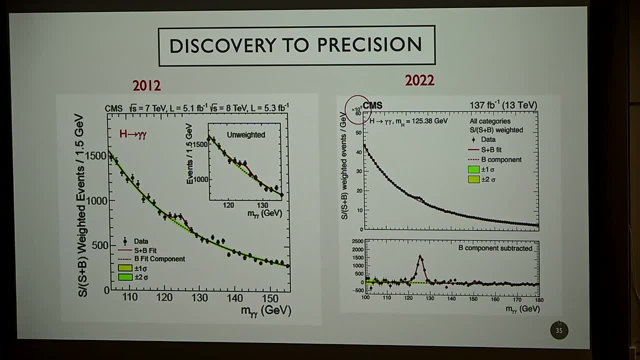 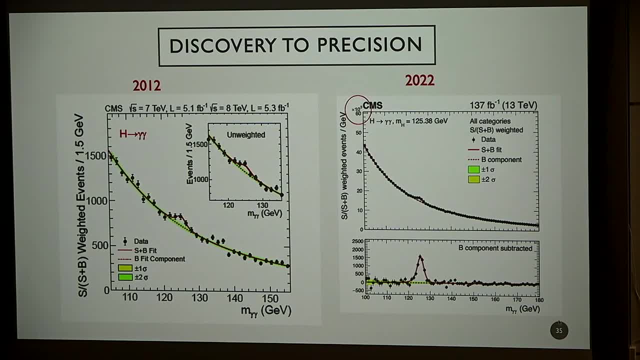 Yeah, Yeah, Yeah, Right. So it depends what question you're asking, Right, Right? Yeah, Because in string theory there are ways to get rid of this. all the physical degrees of weakness, before you've been doing calculations. 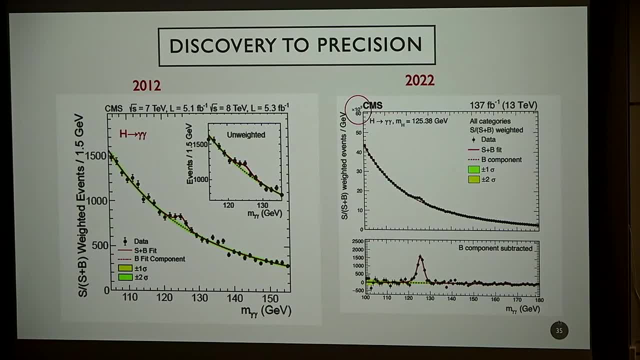 Right, So like light cone, Oh yeah, you can do all these things in light cone. I can't do it, but other people can do it in light cone. I mean, there, there are probably like standards on this. 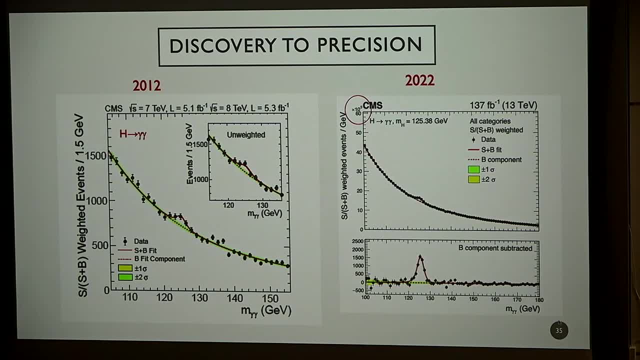 They're very, very wide in this situation, But all that would come out from a physical point of view is interactions and cross-sections. Right, Right, Right, I mean so, But then I mean, if you have the wrong sign for math, then you would have to write down. 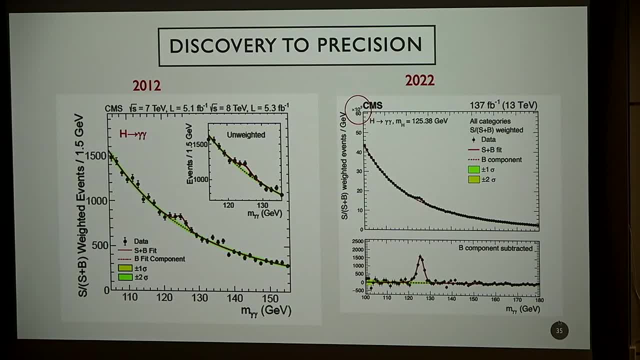 the propagator that has the wrong sign for math, Then you would have to. yeah, like Thomas Thomas. yeah, Yeah, you could do it. Go ahead, Okay, sorry, That's okay, Okay, Right. Yeah, I'm a little bit confused about. 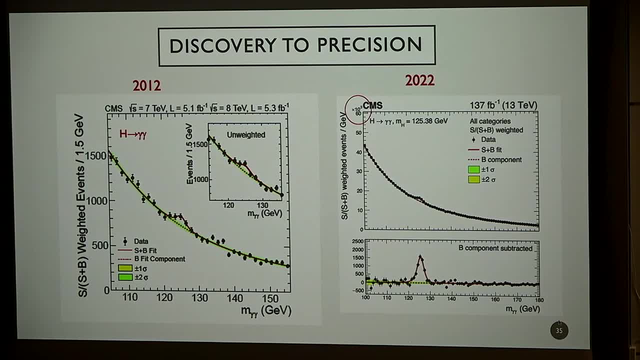 Yeah, Right, Yeah, I'm just wondering. I mean you can further? No, no, Oh, I got to show the PDL thing tomorrow, Okay, Because we're not colliding with protons, We're colliding with the course of gluons within the. 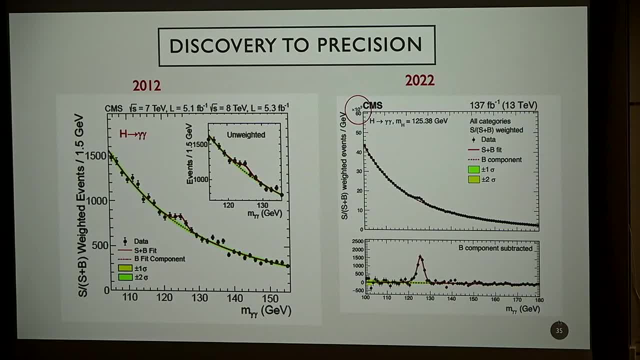 Oh, that's why I'm Like: here is yes, here is yes, So the charges seem to be a little bit different. Okay, No, So it's: you've got the proton, then you've got a spectra, then you've got the. 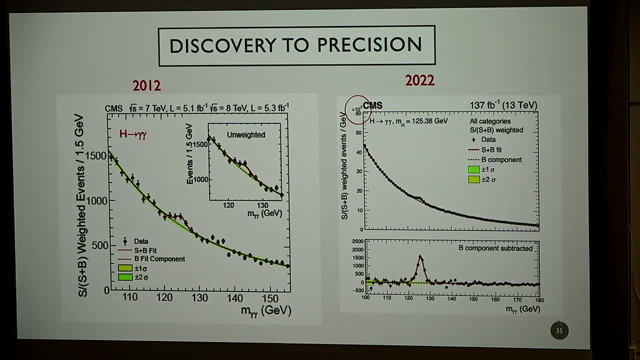 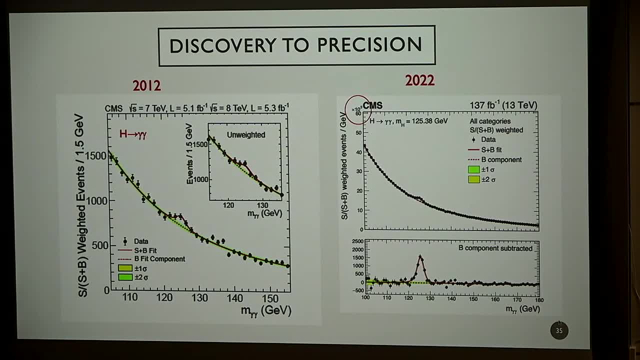 and interaction. I see, I see, Yeah, So these are the constituents colliding and producing something. so this is what happens when you have the two protons collide, but what's happening inside? this is at course of down. Yeah. 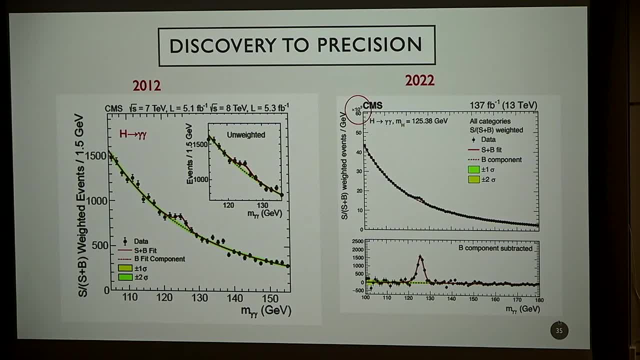 Hi. Hi, I just wanted to introduce myself. I'm tops. I don't, oh, totally understand. Yeah, I stay away from people. You're Tim. I am Tim. Good, Yes, It's so nice of you and I wanted to thank you for answering all my questions. 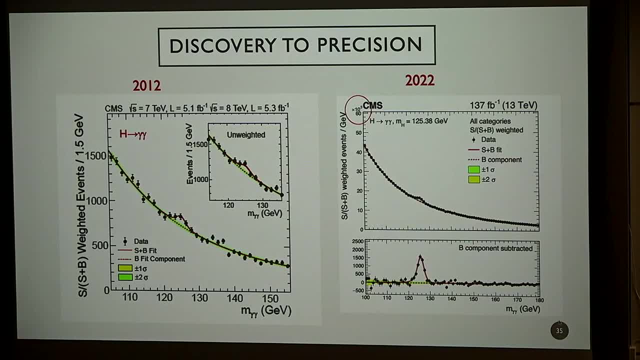 And I hope so. Questions are good because you know everybody learns something from questions, Right? You're saying that you're starting with three and seven. That's more fun. I don't have to get through all of this stuff. 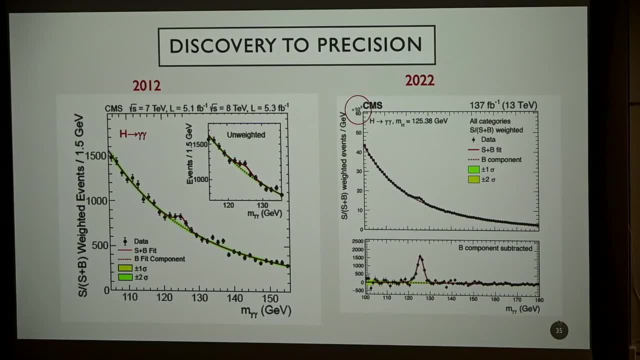 Starting with three and seven, four, and I'm saying I'm looking forward to your questions. Isn't that just an expression of Poincare invariance required on your Go ahead? I have a very unknown question, But you only need it if the 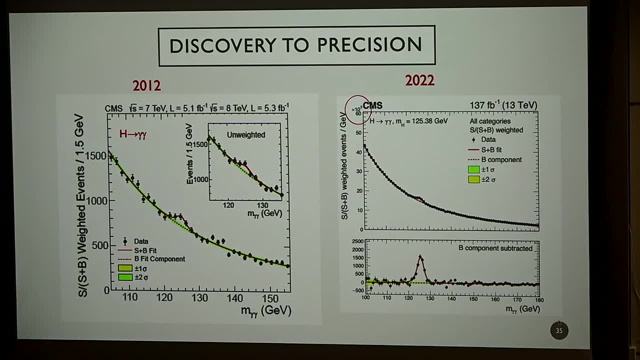 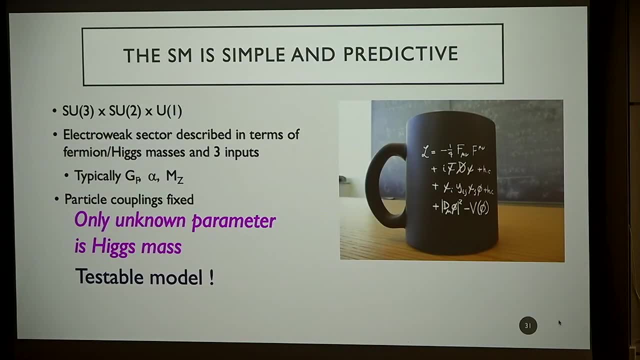 I'm reading your name tag. Yeah, It's not physical, it's never anything. you've measured. It's in the Lagrangian, but you never really measure it. so, yeah, You're probably more familiar with integer from the empathy. 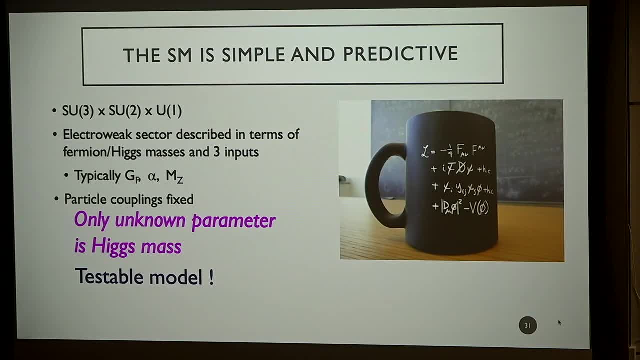 I'd say I wanted to ask you about it. And the bottom one is like a track name: Sayo with a sayo. Okay, so you're saying yeah, notation And, of course, since we were defining, Well, it's mixing direct and while. 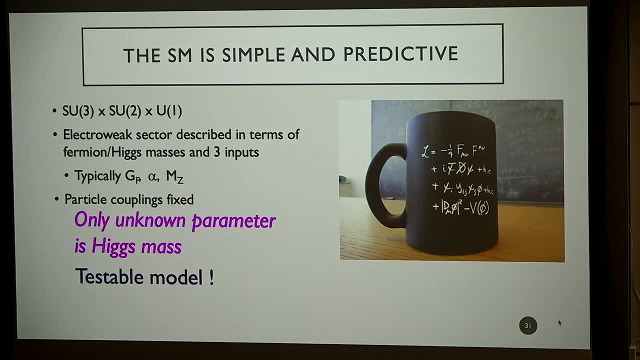 They're just coordinates on your actual group, so they're very much devalued views. They're not physical space time. Yeah, I just want people permission to use stagger. Yeah, it's just yeah, They're all You need all the fine print there. 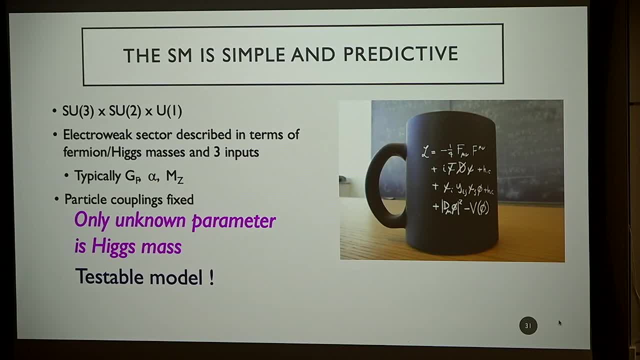 Yeah, And I also thought, maybe for the- sorry for the Yukawa, I think- when we had the sidebar for the. I'm actually not so concerned about the figures of freedom, Not the way I wrote it, Because you know.